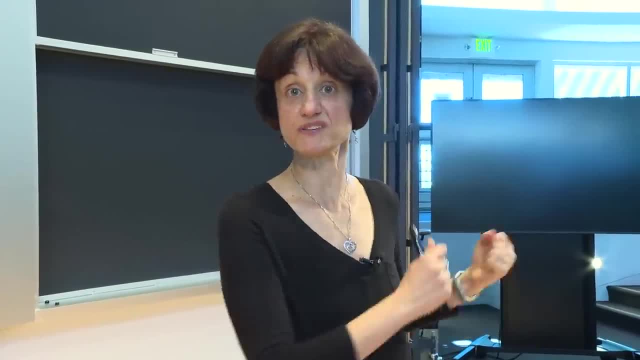 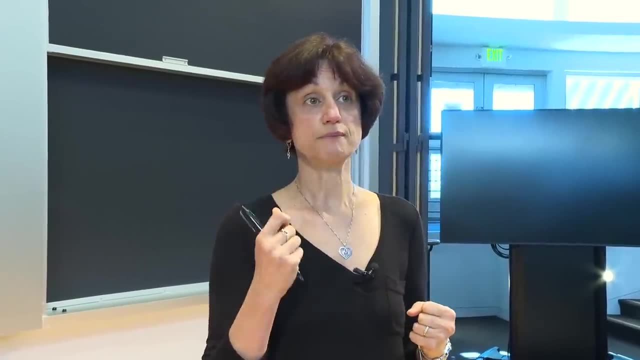 point to another, in particular to prove your mathematical statement. But induction doesn't work without the driver and you will be the driver. You need to come up with creative ideas to fit within this vehicle. So let me give you a problem. This is your decision. let's say it's about nuts, If you want the fourth one to be flat and 2nd one to be provable, then you need to cut off. if you don't cut it off of every dot, You can do it in goodness or Öyley. I'm going to steam around here. So you can actually compare this with the expression. So I'm going to continue cutting here and going to have the next level thing because of Cardioted view of the top right corner equivalent. okay, this is the cat to get the bottom one. Well, that's eight units between years. 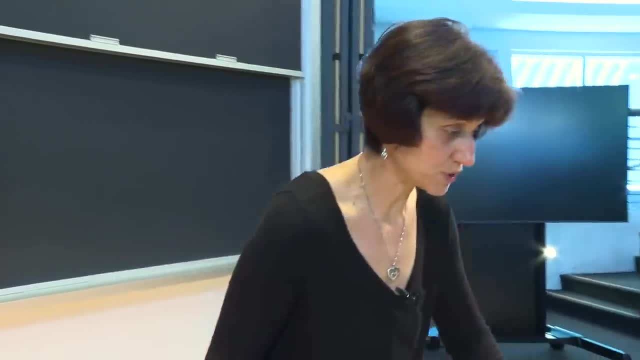 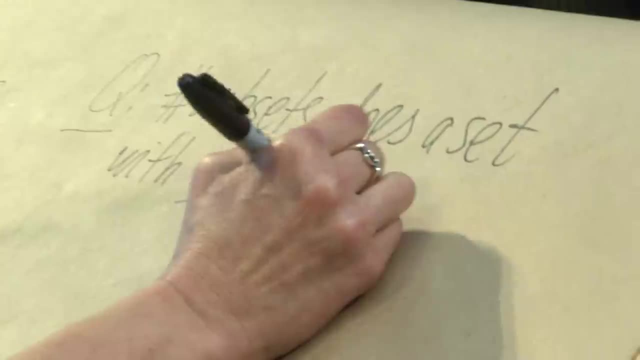 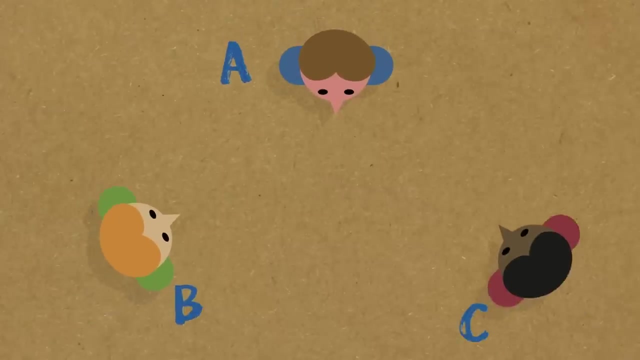 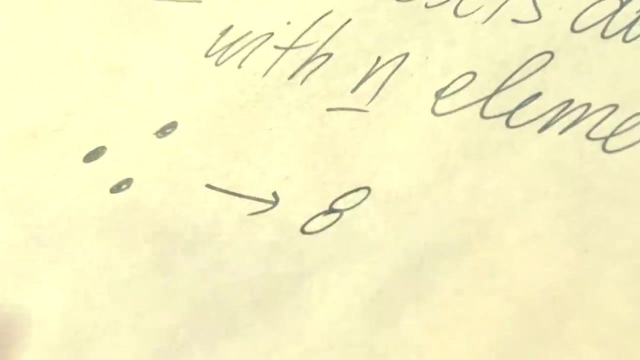 that you may or may not have seen before. It's a very famous one: Find: how many subsets does a set with n elements have? So what am I talking about? If you have three people, how many groups can you extract from them? And so you can fiddle around and maybe you will come up with the answer. eight. 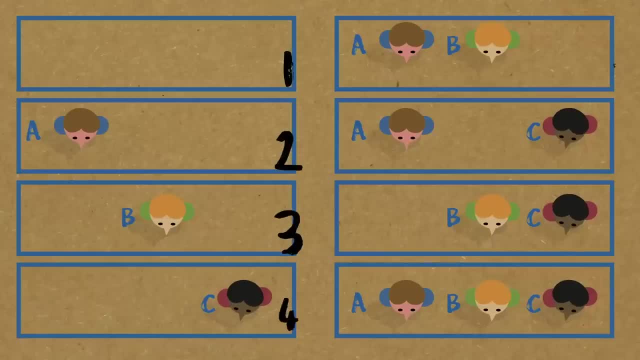 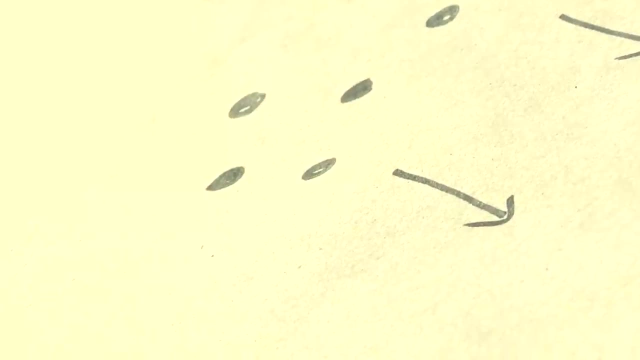 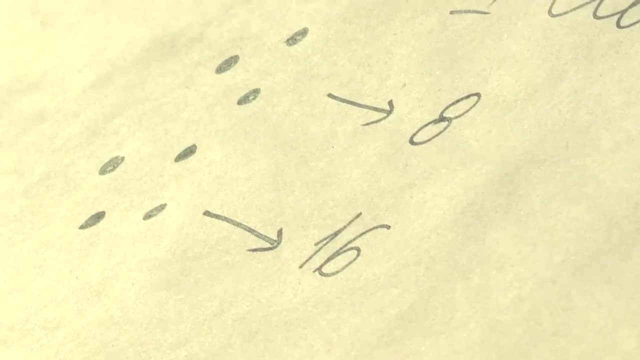 That seems like a lot, but actually that's the case and we will show it. And then you try with perhaps four people and you know, you count, count, count and you come up with 16. And of course you start seeing a pattern And you're saying, oh, maybe the answer is a certain power of two. 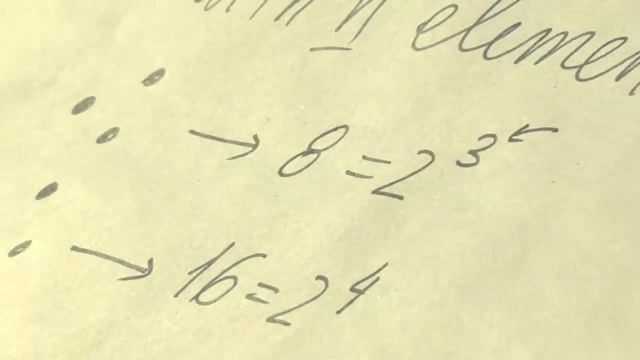 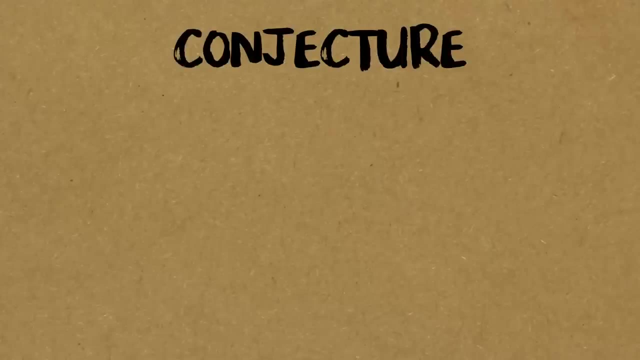 And the power of the exponent looks like it's the number of people or the number of elements. And at this point you say- I'm going to conjecture- that the answer for this problem, which I'm going to call S sub n. 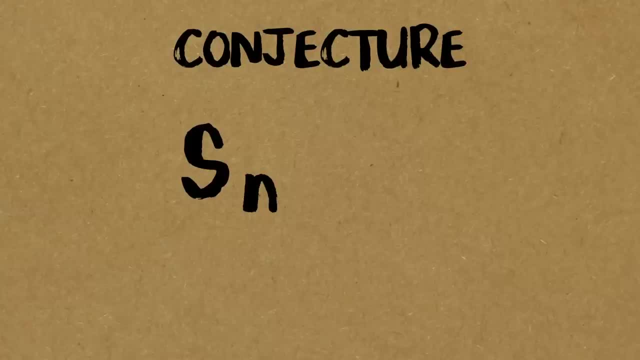 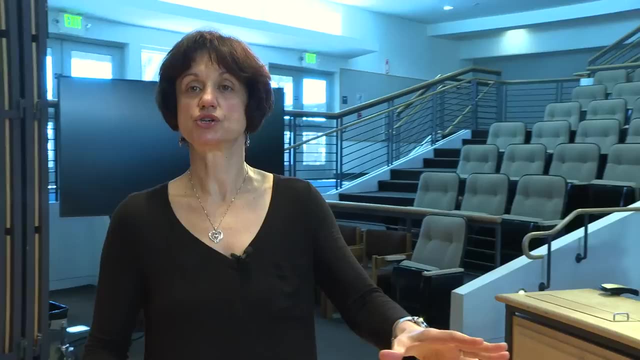 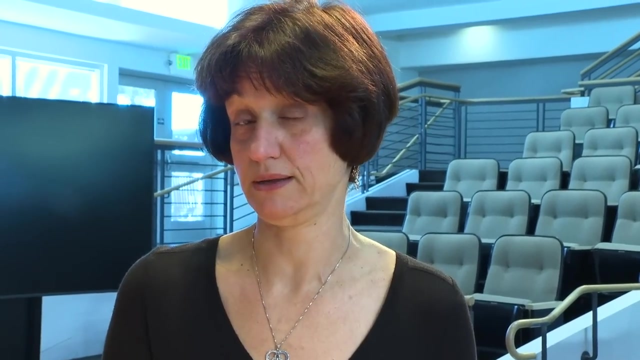 so number of subsets, if you have n people, is precisely two to the n, where n is greater than or equal to one. And now that you have this conjecture, induction can kick in One of the drawbacks of induction, not to disappoint you, but I have to tell you right away. 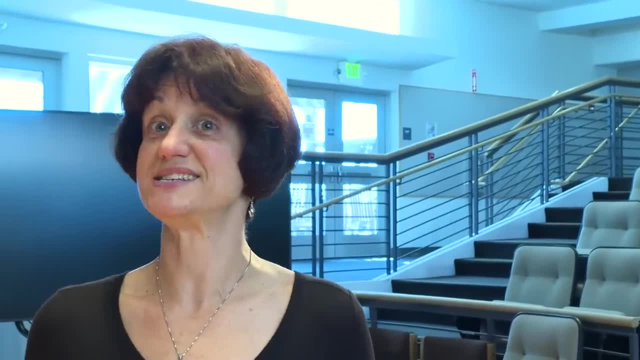 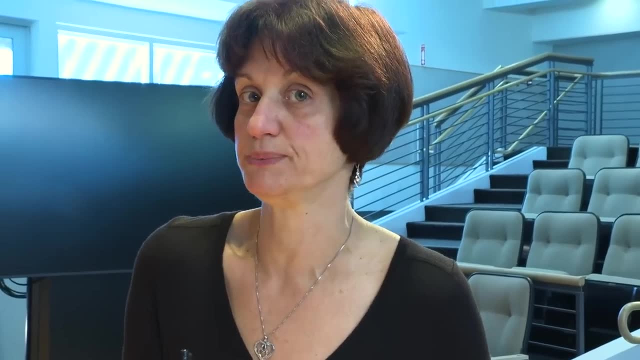 is that you need to know the answer ahead of time. Induction by itself is not going to tell it to you, But once you have it, or some annoying classmate of yours gives it to you, pretending they know too much, you can use induction and try to prove it. So how do we prove? 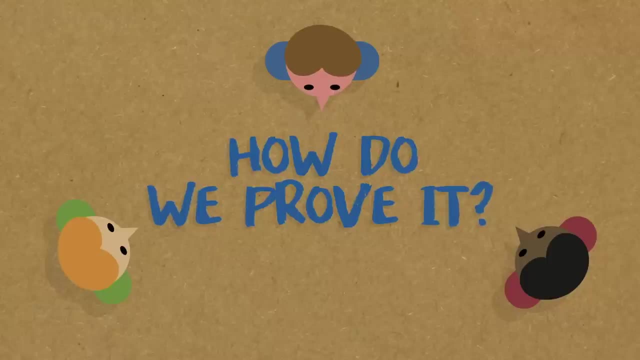 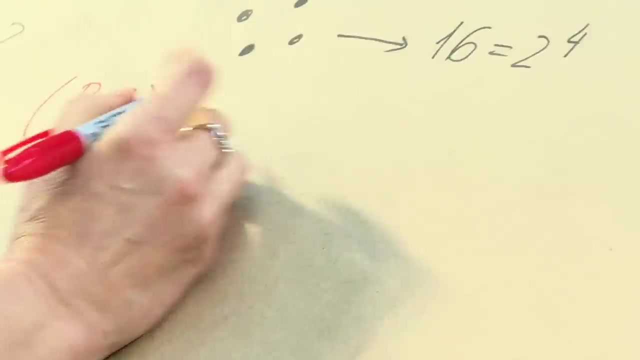 this particular warm-up problem. So induction starts with turning on the engine, your key ignition. So we're going to call it the BS base step. Usually call it base case, but BS really caught you, So base case or base step. 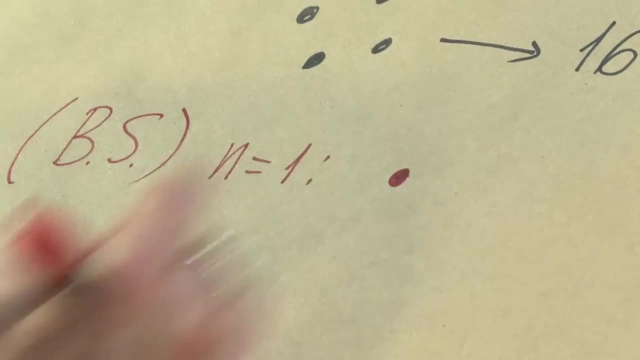 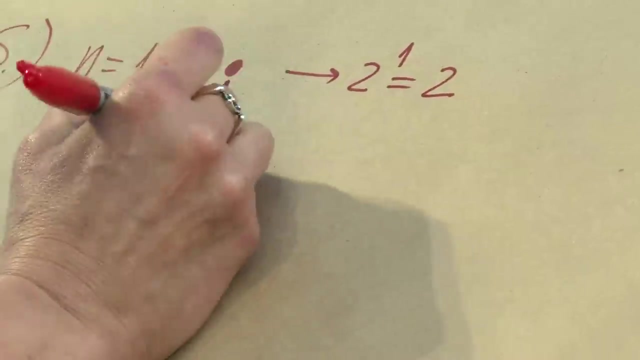 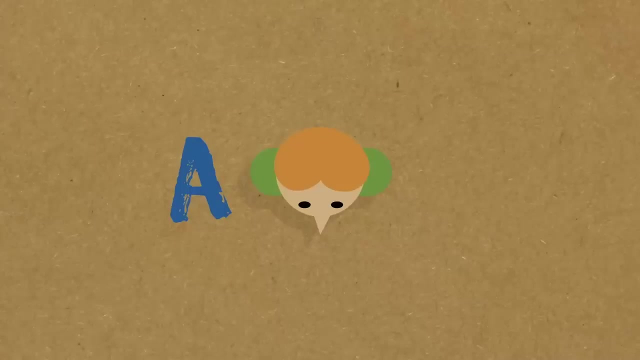 n equals to one. So for one person, how many subsets do we have? Well, we're supposed to show two to the first two. Of course, I can have this person A by themselves alone. Where is the other subset, Brady? do you see another subset here? Is it no people? Yes, no people We forgot about. 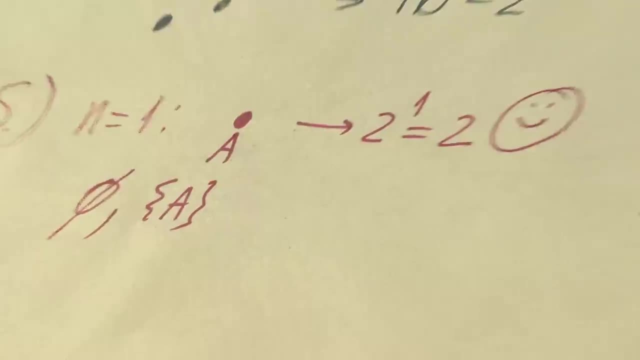 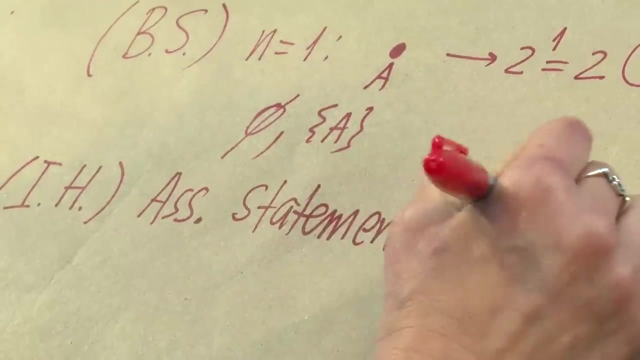 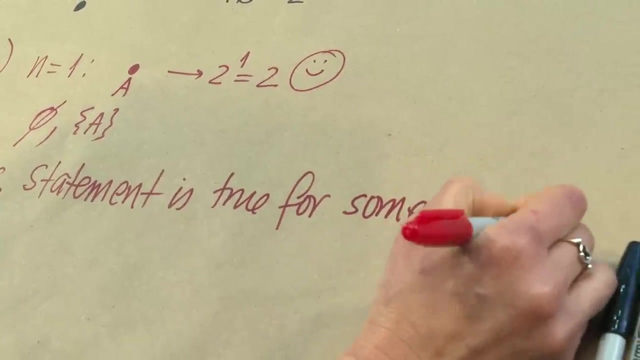 them Great. So that's two. We are done with the BS. Next I'm going to do something called the inductive hypothesis, IH. So I'm going to make a bold, bold assumption. We shall assume our statement is true: for some n greater than or equal to one- And by that I mean a natural 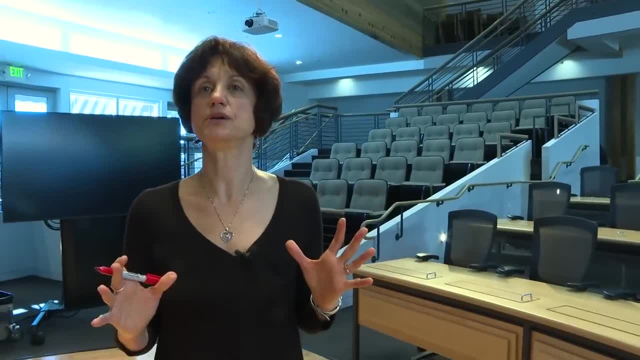 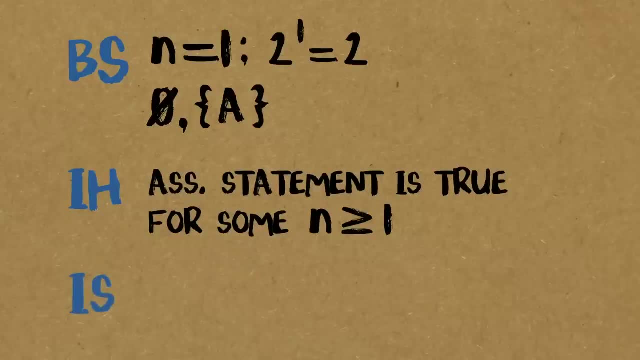 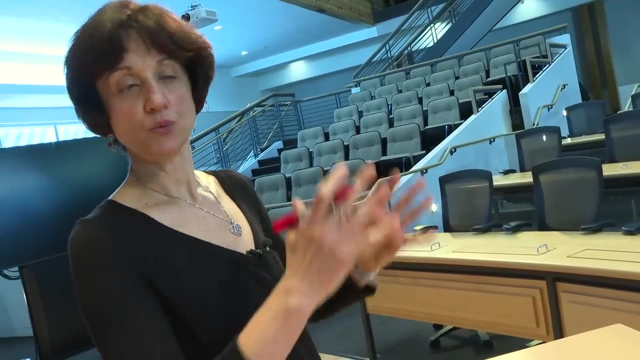 number. I'm not going to tell you what this number is, And that's the key, because I want a general frame that works. And then the creative part of induction. this is where you come in: How many subsets do we have? Well, I'm going to show our statement, And the next statement is also. 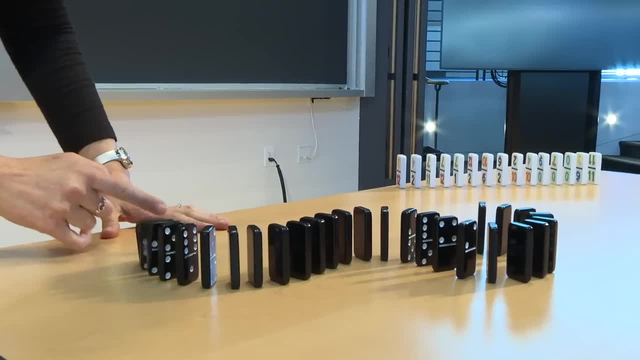 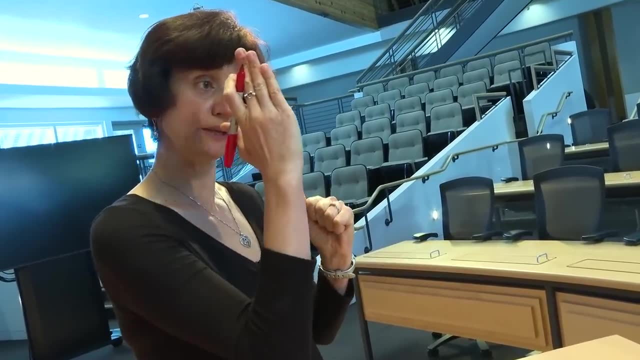 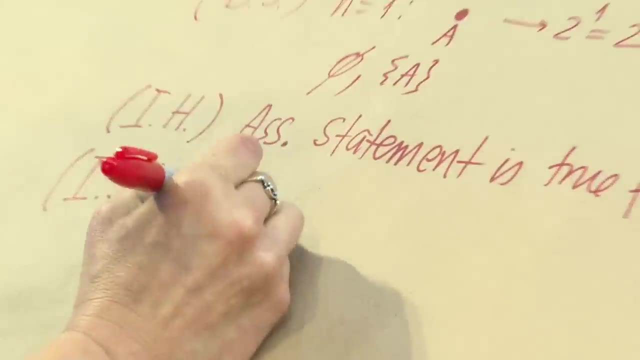 true What you saw with the dominoes. we place the dominoes close to each other so that when one domino tips, the other one is also going to tip and fall over. That is precisely what we are doing. We are assuming that the nth domino falls and is going to trigger the n plus first to do the same. 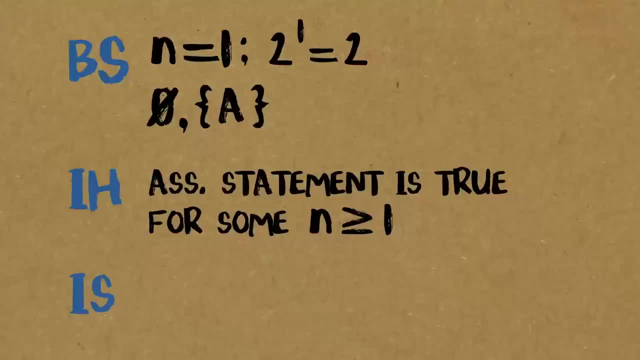 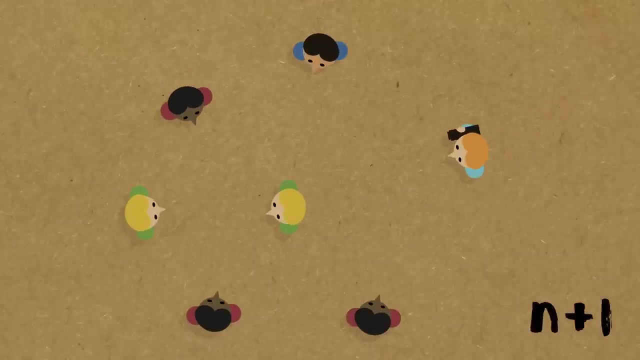 thing. OK. So in this problem we want to show that if you have n plus one people, that means that you have two to the n plus one subsets. OK, How does this work? Here are my n plus one people. I'm just drawing a few points: n plus one. We're going to call one of them Brady, And Brady will. 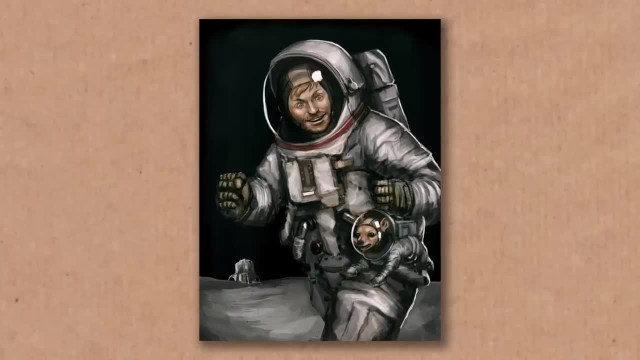 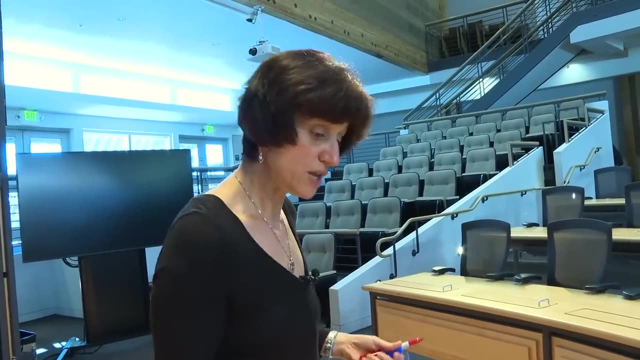 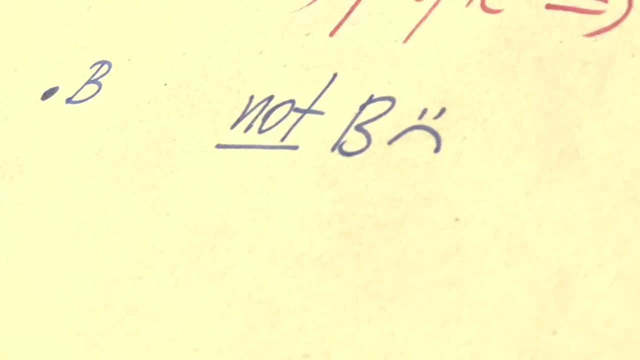 either be selected on a team to go to the moon or not. So we want to know how many such teams we can send to the moon from those people. So if Brady is not selected, so Brady he's not happy, He's not going to go to the moon. How many teams do we have? It means that we are 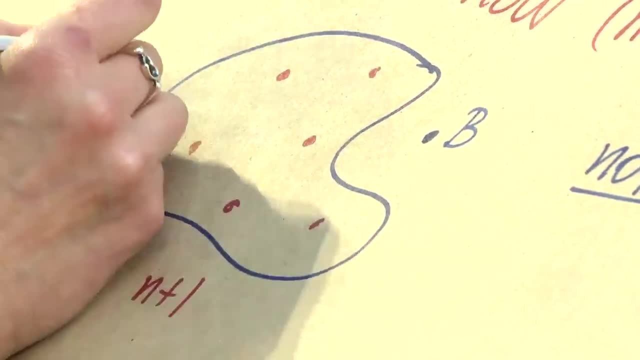 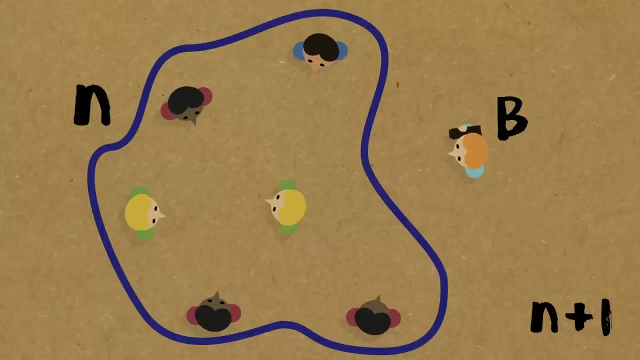 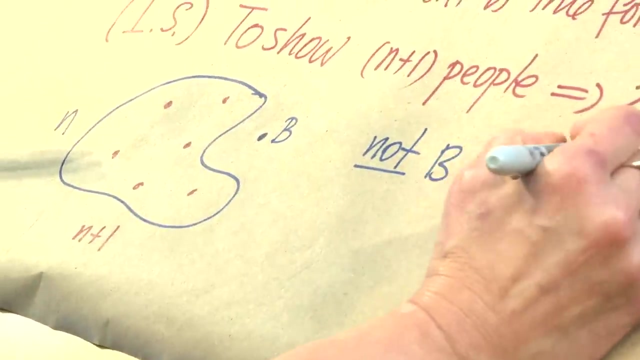 choosing teams or subsets from the remaining n people, But we already assumed that our statement is true. In other words, for n people, I have two to the n teams or subsets. So if Brady is not participating, I have two to the n teams. Now, if Brady is participating, I have two to the n teams. 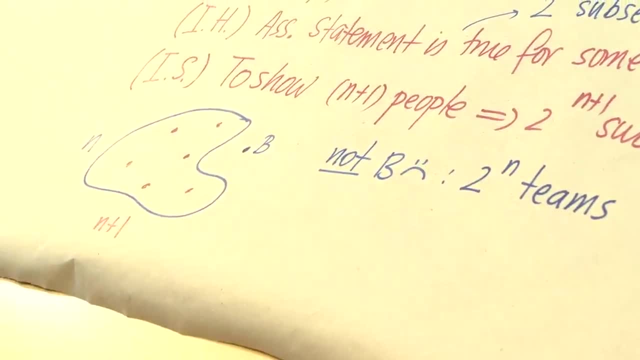 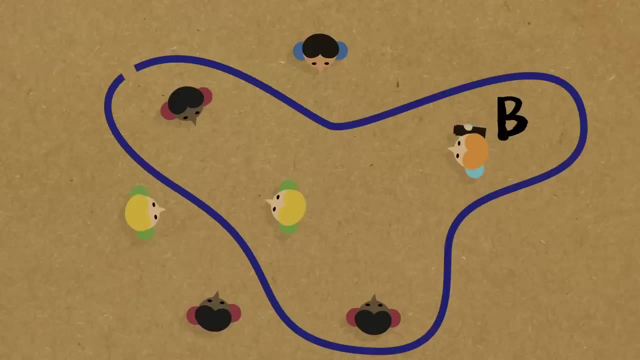 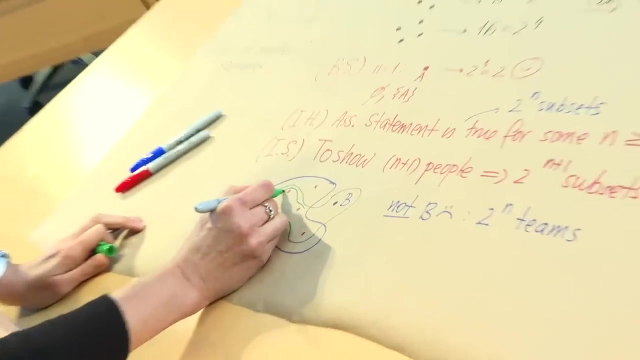 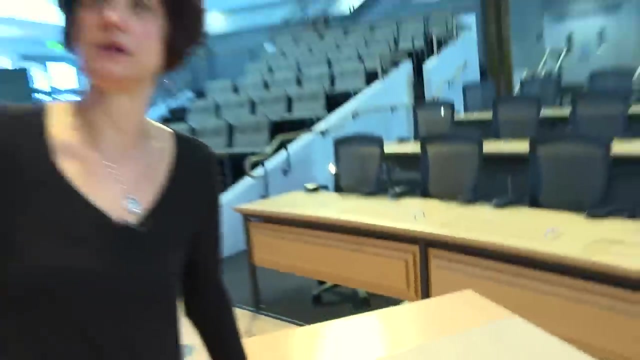 Now, if Brady is participating, how many teams? Well, what is such a team? Such a team will contain Brady and probably a bunch of the others, right? But then such a team means that I have to choose the non-Brady part and add to that part Brady. So Brady is not relevant again, unfortunately. 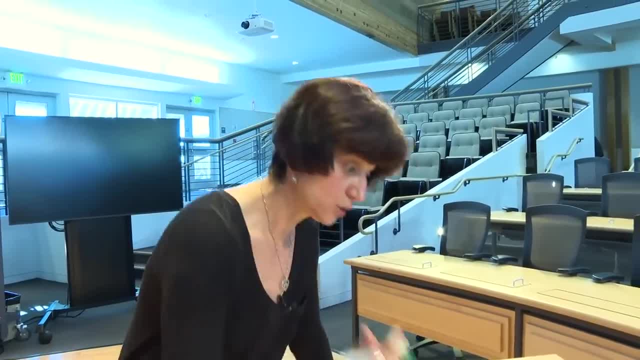 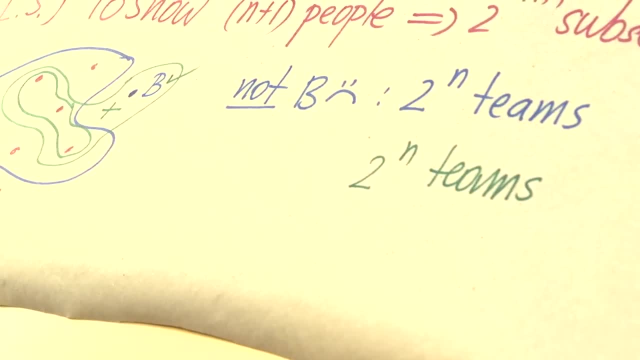 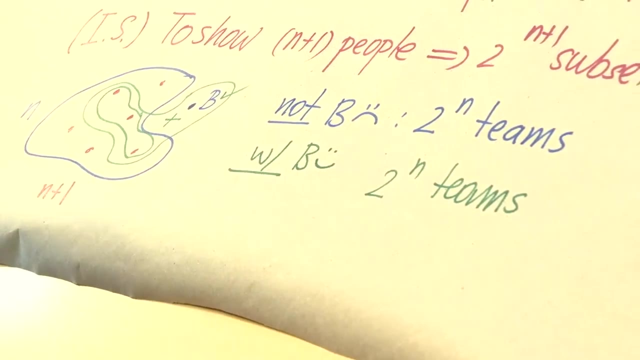 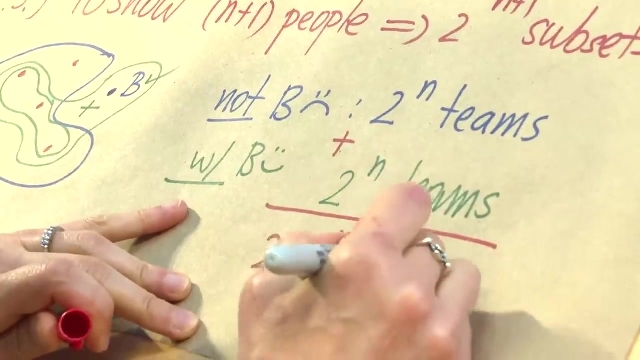 I just have to choose a team without Brady, 2 to the n of those teams, by our inductive hypothesis- and then add Brady. Okay, so how many do we have now Overall? all I have to do is add 2n plus 2n, so that's 2 times 2 to the n, 2 to the n plus 1 teams. Excellent. 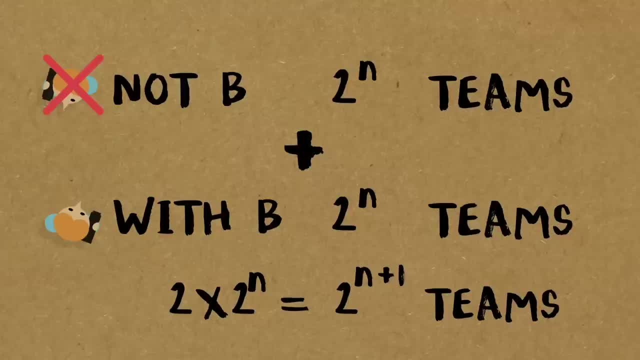 So we have 2 to the n plus 1 teams- Excellent. So we have 2 to the n, 2 to the n plus 1 teams- Excellent. So we just showed the inductive step And here, if you want to be absolutely formal, you. 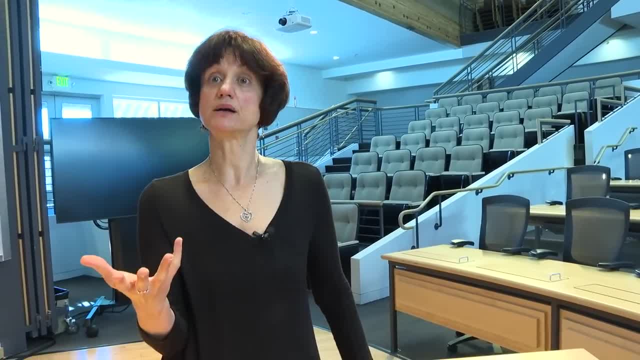 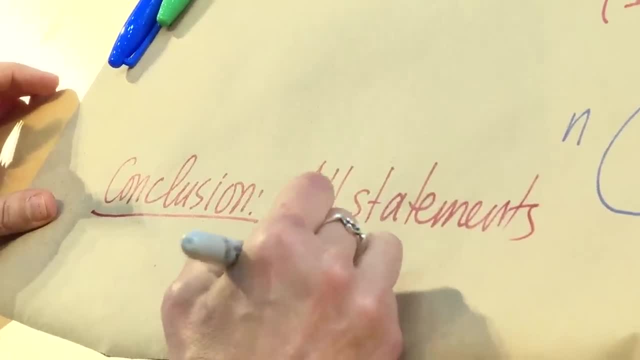 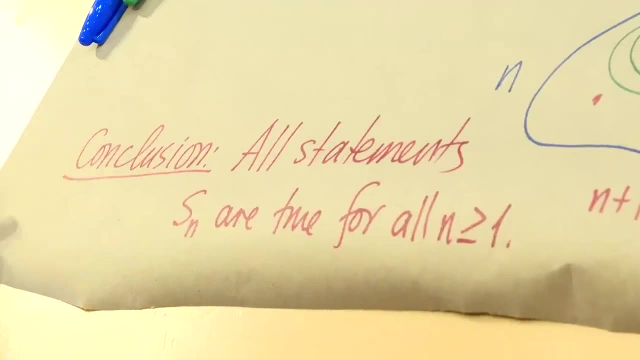 want to receive a receipt for your proof, you have to make a conclusion. The conclusion says, therefore: all statements SN are true for all n greater than or equal to 1.. This seems like a lot to say, but actually that is the domino effect. 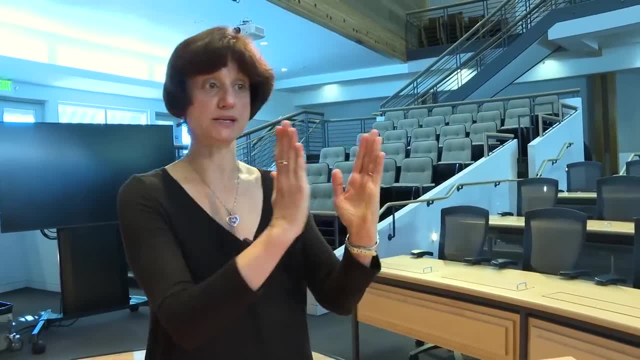 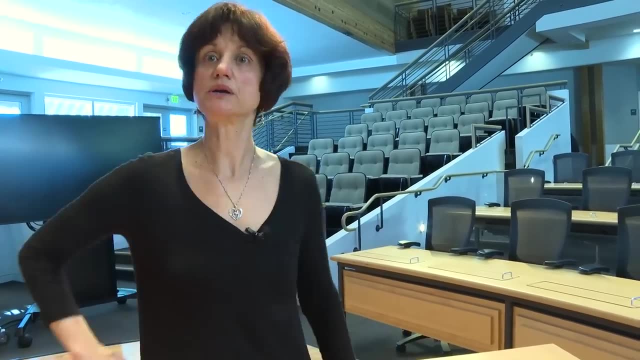 If you believe that when the dominoes are placed close to each other, then once you push the first one, all of them will fall, then you should agree with this. Alternatively, let's think about Grindelwald: evil magician. Okay, so he does. 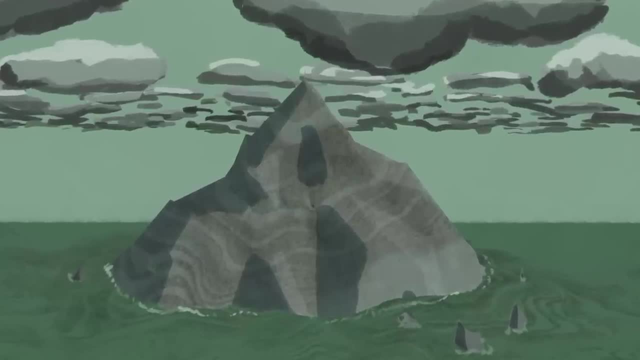 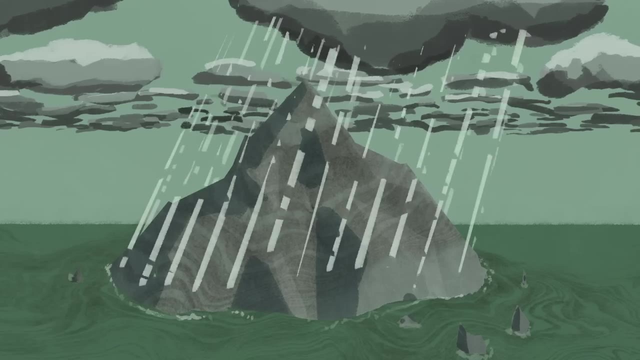 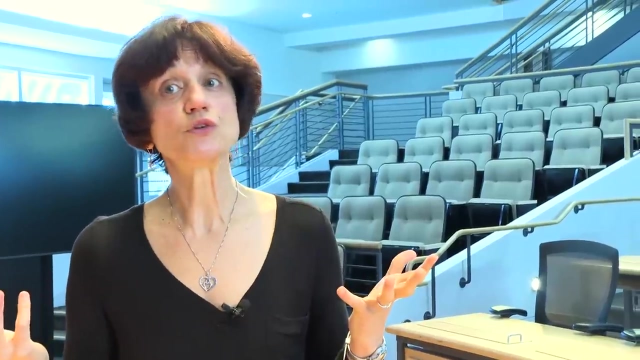 all sorts of bad things. on an island, the good magicians gather together and they're gonna exile him Upon leaving the island. Grindelwald casts an evil spell: If he trains, one day, it's gonna rain, the next day It rains today. Will it rain forever? Brady on this. 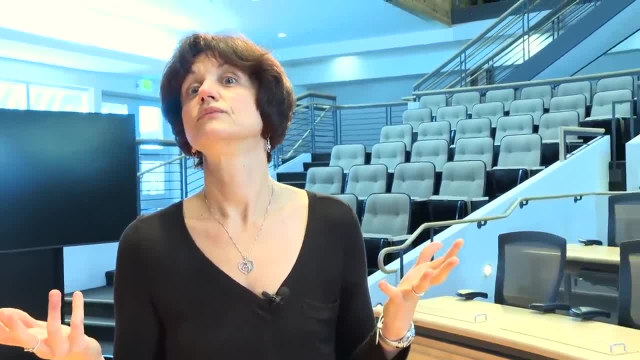 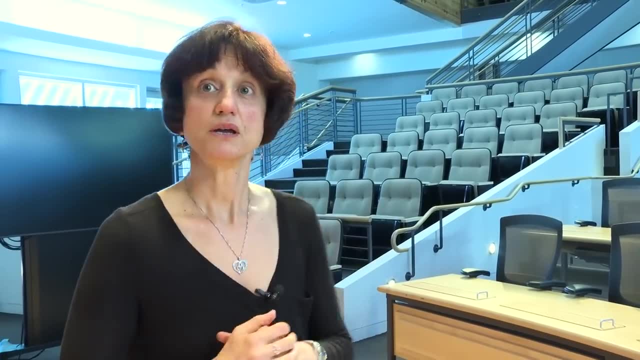 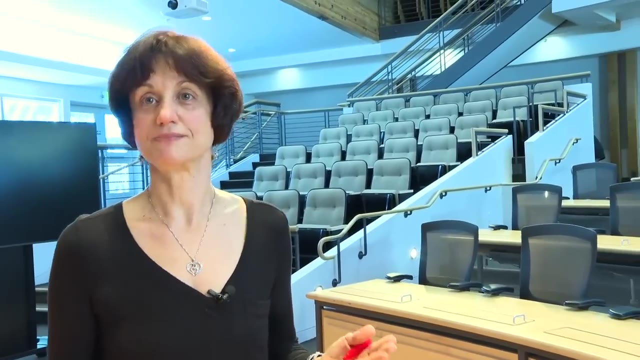 island. What do you think? I think it will, yeah, Yeah. and so it means that Brady believes in the method of mathematical induction, because in this example with the evil spell, what is the BS, The BS or Bay step? is it rains today? What is the? 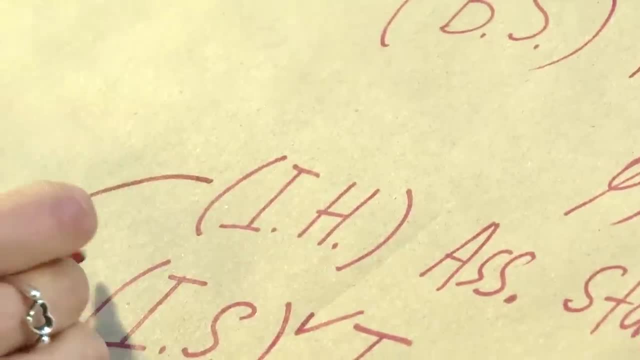 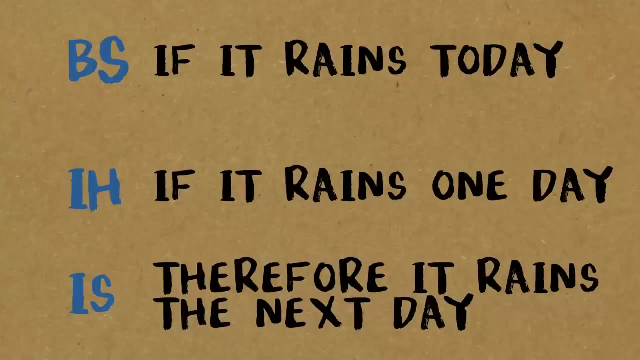 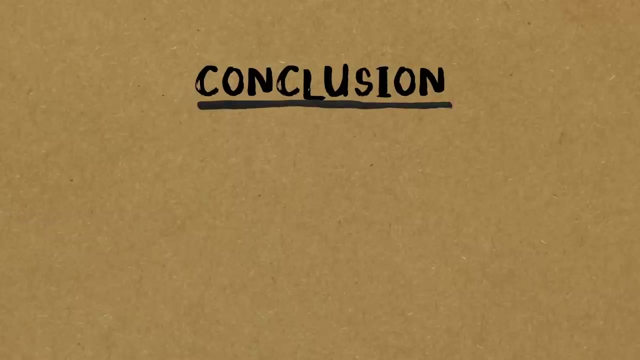 inductive hypothesis and the inductive step. Well, that's the magic spell. The inductive hypothesis would be: if it rains one day, and the inductive step will be: therefore it's going to rain the next day, And so we're gonna conclude that, in this case, Grindelwald will win. 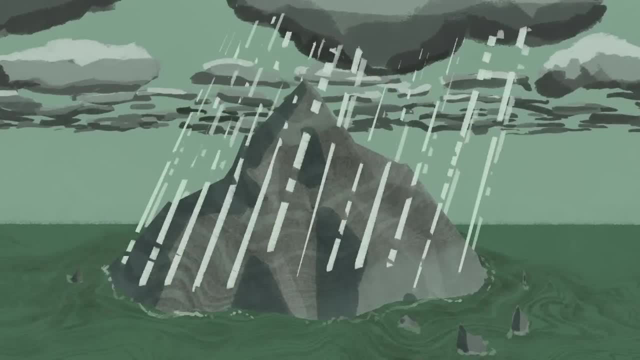 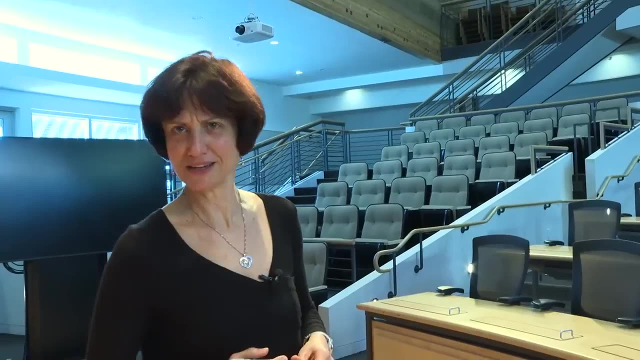 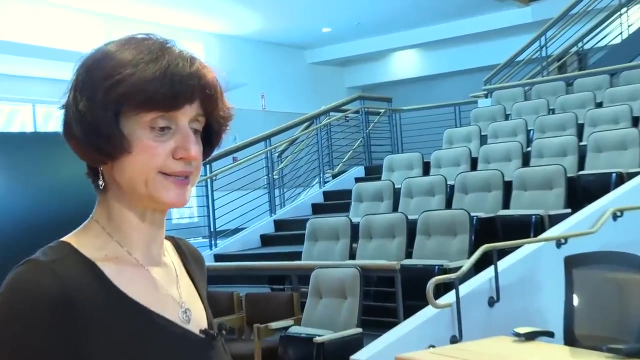 On that island it will rain every single day, So you might think about the domino effect. it's a little bit more optimistic, but either way will work. Now just a little bit of a story Switch here. Once you realize that the statement for the number of teams was: 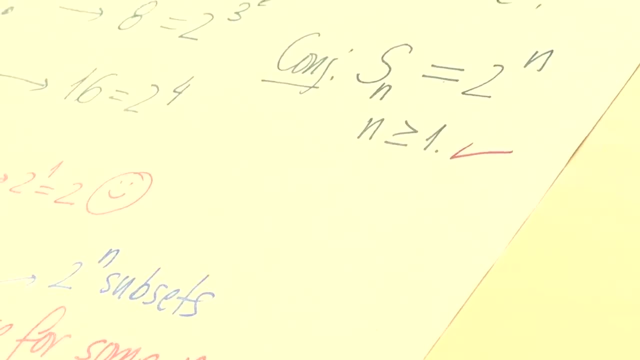 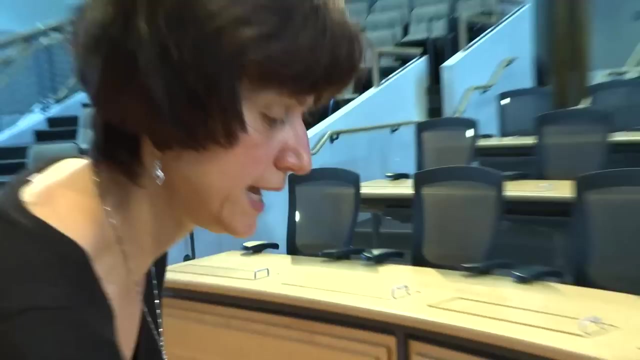 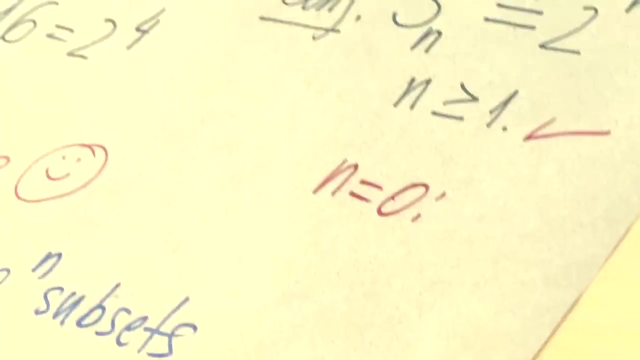 correct for n greater than or equal to 1, you start asking yourself: can I slightly extend this? Doesn't induction always have to start with n equals to 1?? How about n equals to 0?? Would that work? So, if you have no people, how many teams? 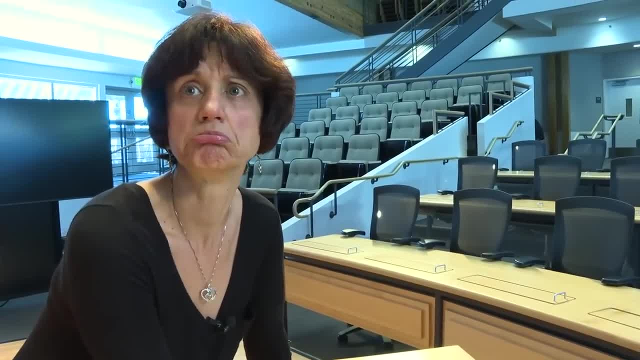 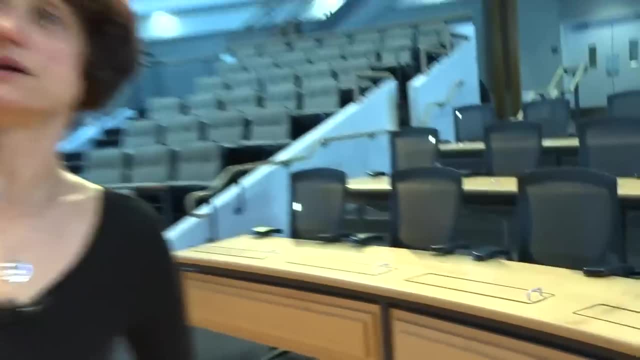 do you have, Brady? what do you think? 2 to the 0.. 2 to the 0,, which is 1.. And what's that team? That's the empty one. Wow, So we are extending actually our formula to one more case and indeed induction can start from. 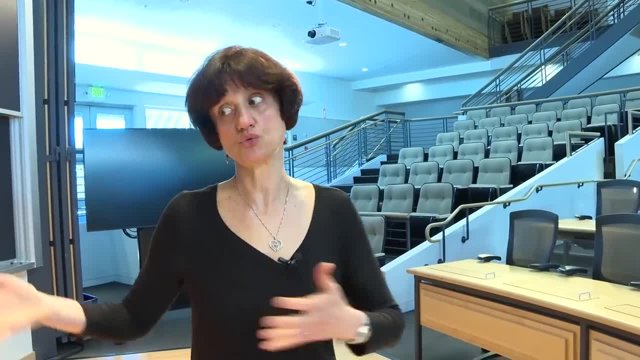 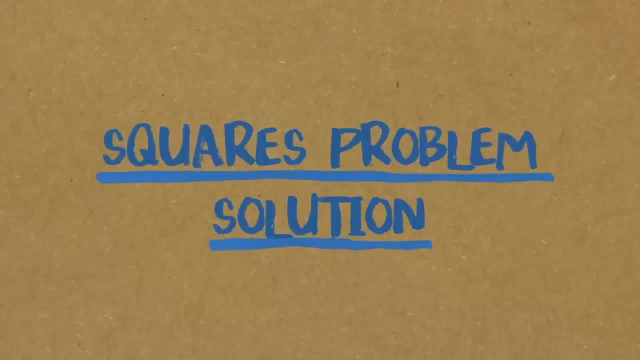 wherever the statements are true. It could start from 10, or you can even started from negative 5.. So now we are ready for the squares. Remember, into how many small squares can we cut up a square without any monkey business? No overlaps, no other things. 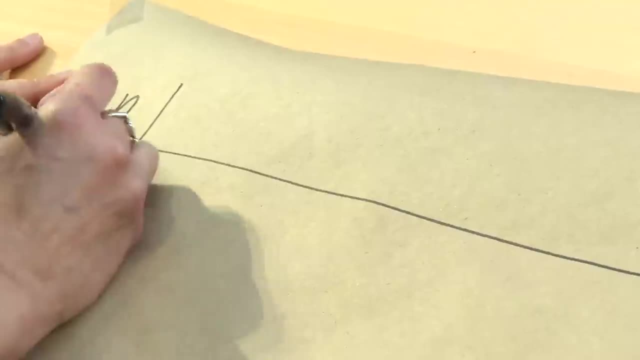 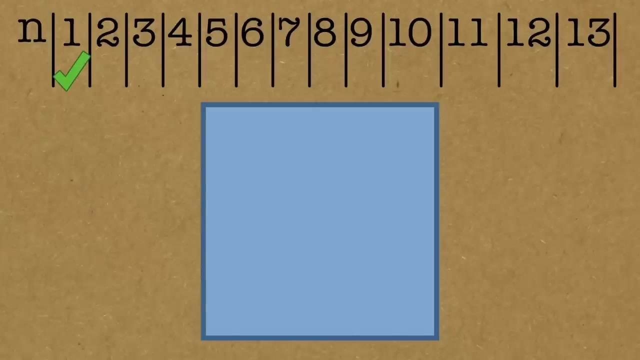 stuff. so n is going to be the number of squares, and then we will say whether we can do it or not. okay, so if n is one, obviously we can do it. this is our square, there is nothing to talk about. but once we start going higher, things get trickier. Brady, just think and tell me one of those cases where 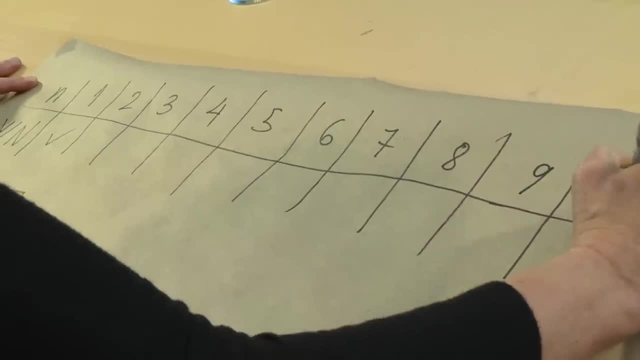 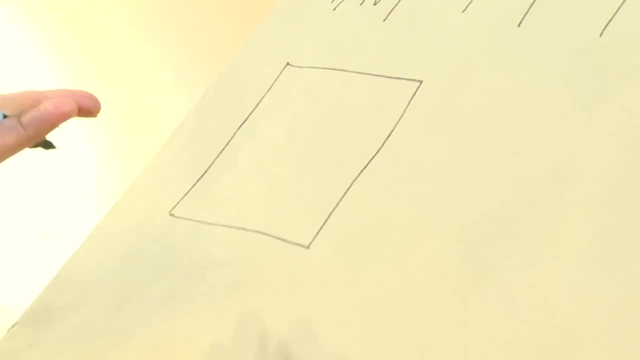 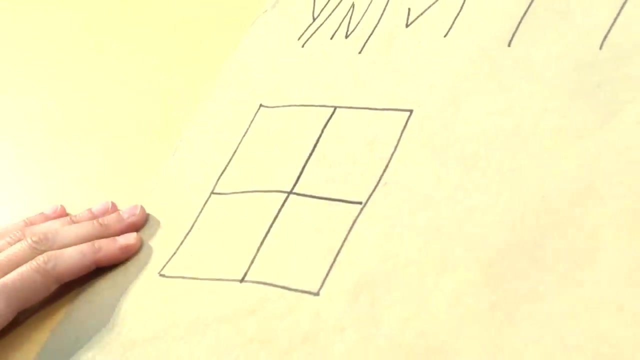 you think it's definitely possible to split a square into smaller ones. four, four, yes, and how do you propose i split this into four smaller squares? you cut that in half vertically and horizontally, correct, and we're gonna call this the window technique. we see a nice window here, so four. 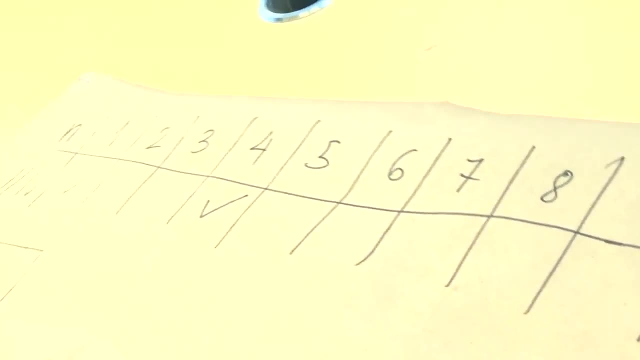 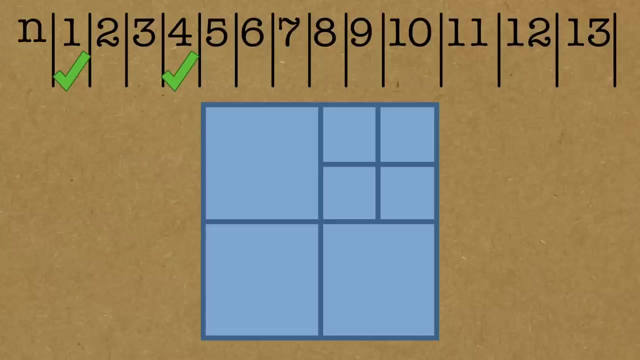 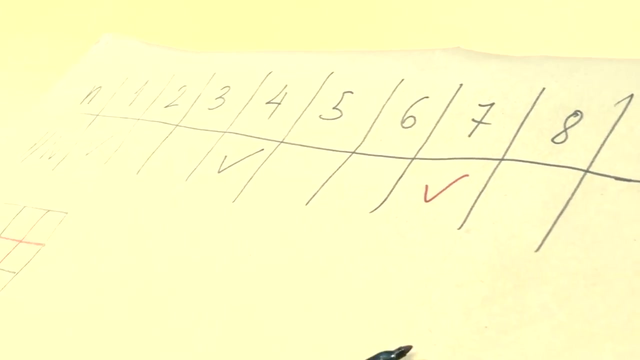 is fine. um, anything else? um, i could use this one. you could window all those squares. oh, i can window in one of those. and how many did they get? did they get eight? no, no, what, seven? what? what happened? so, seven is okay, but what happened every time? 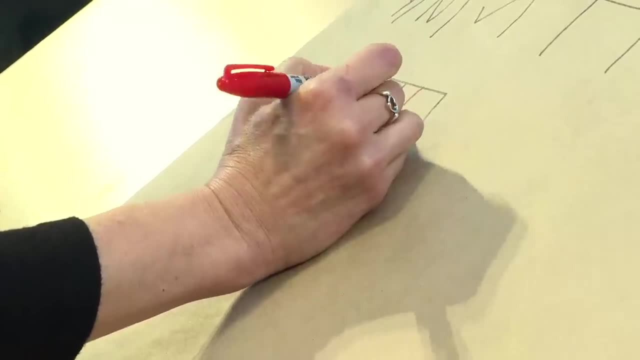 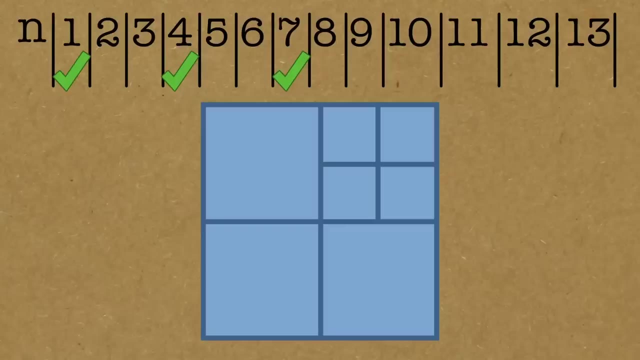 you use the window technique, you are replacing one square with four, which means that you are adding only three. so once i have seven, what else would i have ten? ten, because we will start adding threes here. excellent, and obviously i can have them. thirteen, which is out here. but now what? i still have some gaps. what do i want to do with the others? 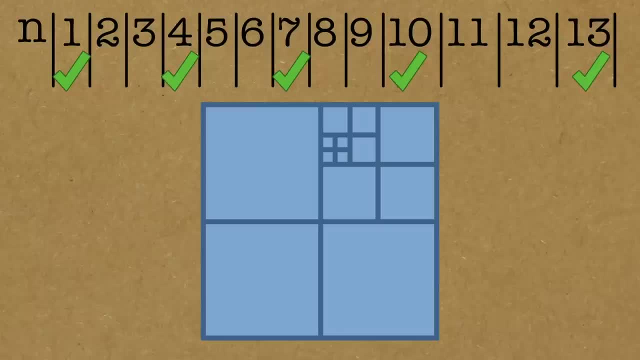 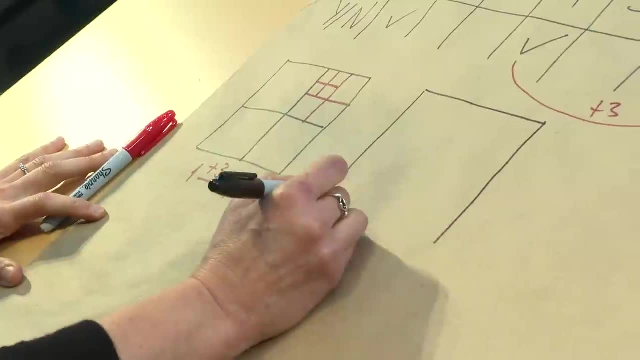 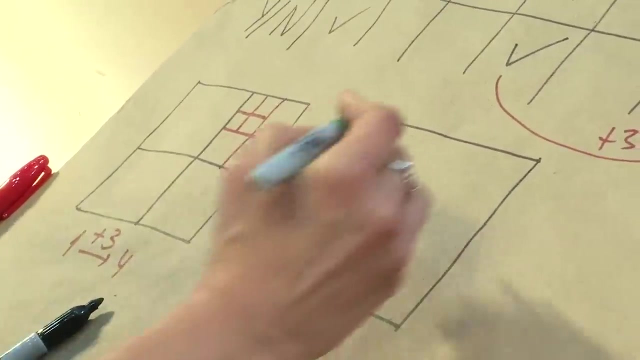 this is not so easy anymore. maybe i'll help you, unless you've already discovered how to do it. is there a way to do it for six? now? we have to be more inventive, okay, so suppose for a moment i split this into nine squares- right, and everyone agrees- into nine. 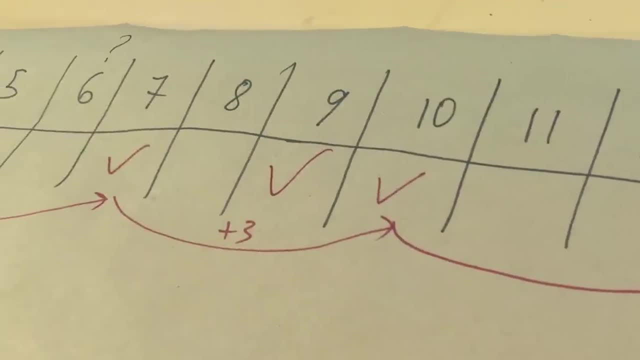 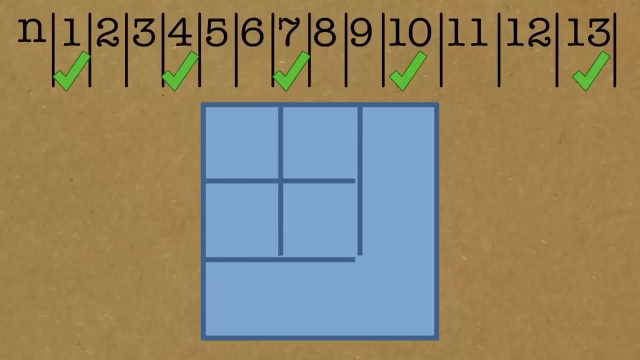 it's possible. oh, so that's possible, and then i'm going to use only some of those for my six squares in particular. these four squares will be now lumped into one large square. well, how many do they get? one, two, three, four, five, six. ah, so six works, and then from six on, oh, this is really fun. 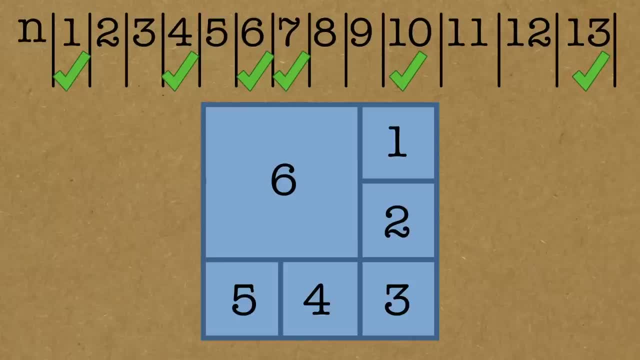 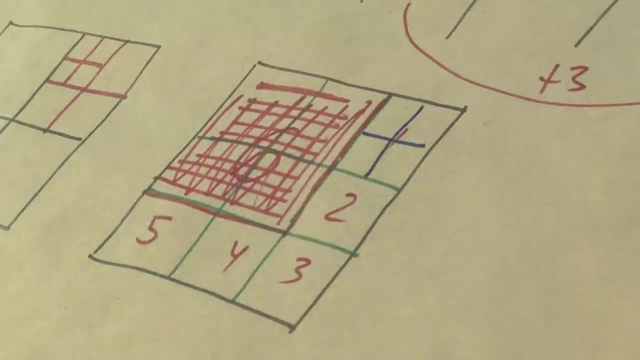 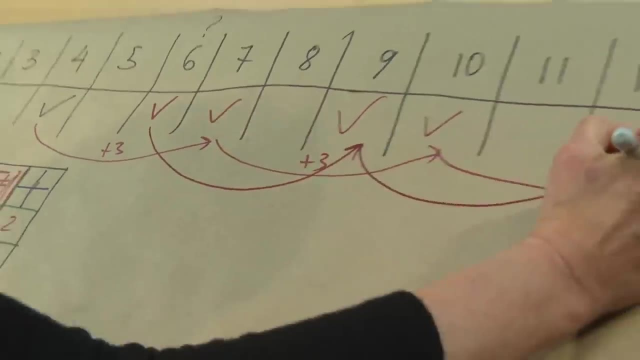 because i know how to do nine. that was our original cutting, but now i have another way to do nine. right, i can use the window technique on my six and split like that. but at any rate we now know that with the window technique we can go and cover. 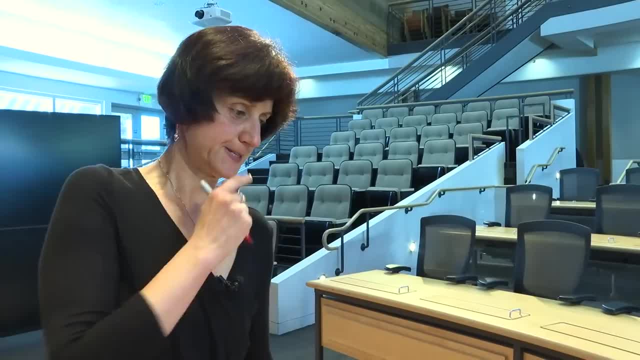 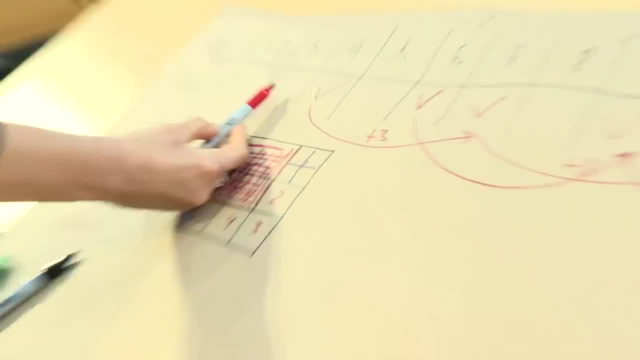 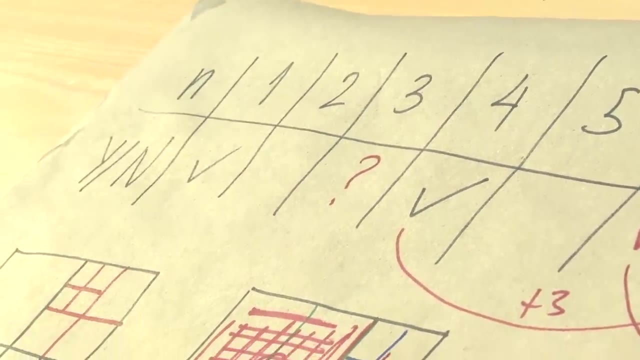 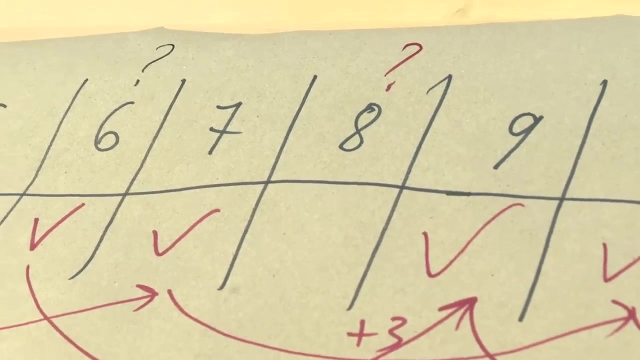 another long sequence of of events here. we can do it. six, nine, twelve, um, i wonder, can we roll back to three? can you possibly do it with three? i can't quite see it, so let me just let this boil a little bit. simmer on the back burner. um, something else. how about eight? can we do it with eight? what we 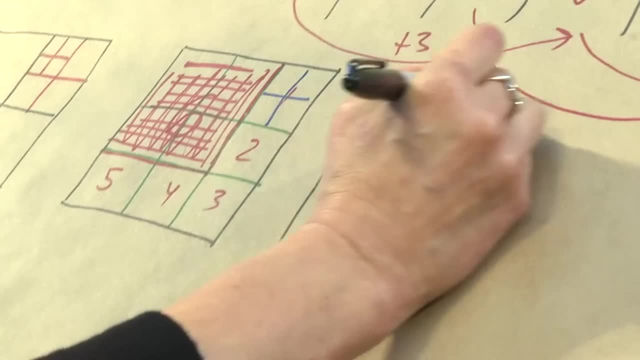 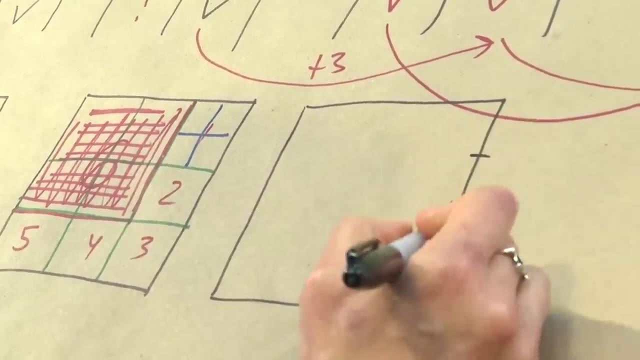 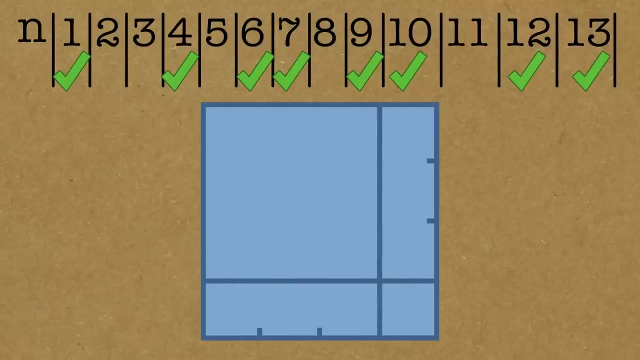 did with six can be generalized for eight. so for eight you could in principle do the following: cut the side into four equal parts, those two sides, and then go straight only along some of those and finally cut up the remainder. so you're gonna get one large, two, three, four, five, six, seven, eight total, so seven small squares. so 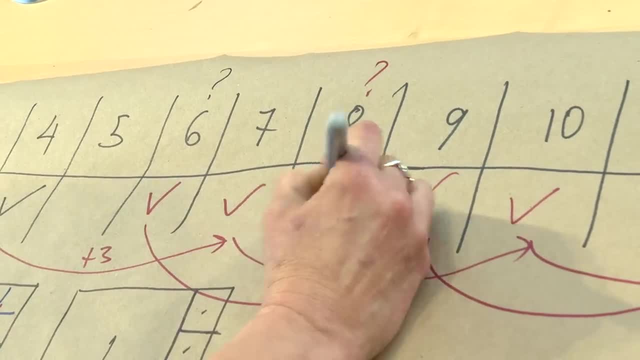 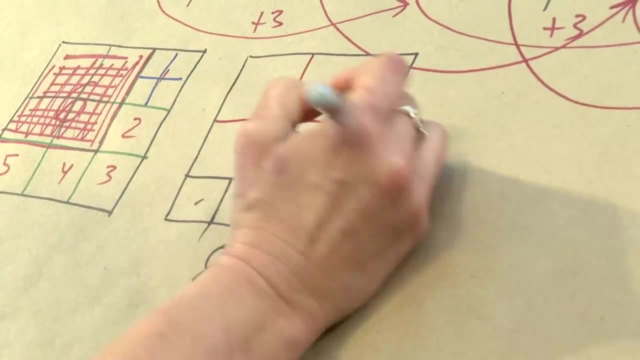 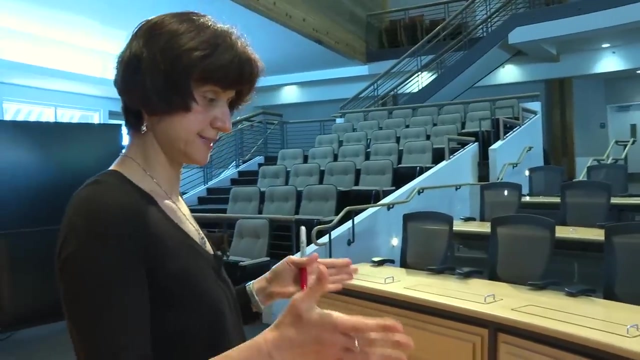 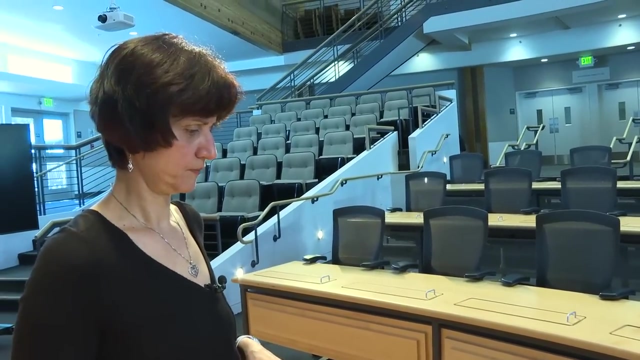 that's eight, so we are done for eight, and that will trigger eleven with the window technique 14 and looks like we are fine from now on. so, brady, what do you conjecture based on this table? when is it possible? from where on is it possible? well, so far it seems like it's possible from six, everywhere onwards. 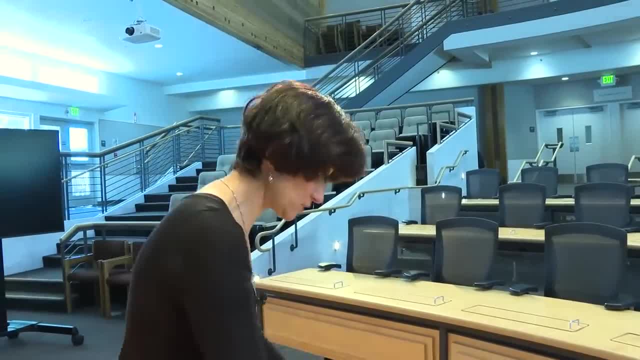 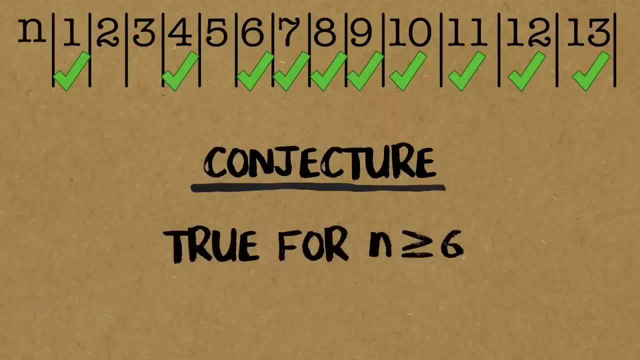 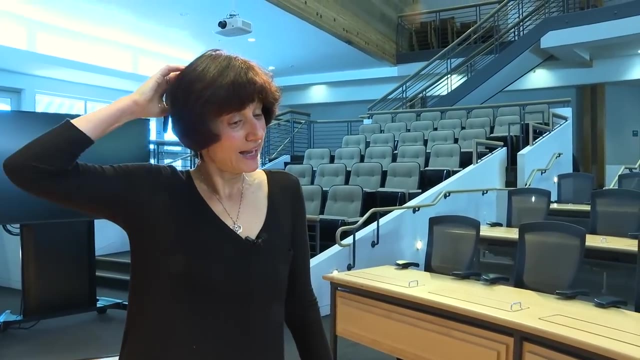 correct. that's where the dominoes start. that, yeah, and actually that's what i will conjecture. we will conjecture that this is true or possible for n greater than or equal to six. why are you conjecturing that? you've proven it? well, i said them so on, every time when you start saying: and so on, et cetera, et. 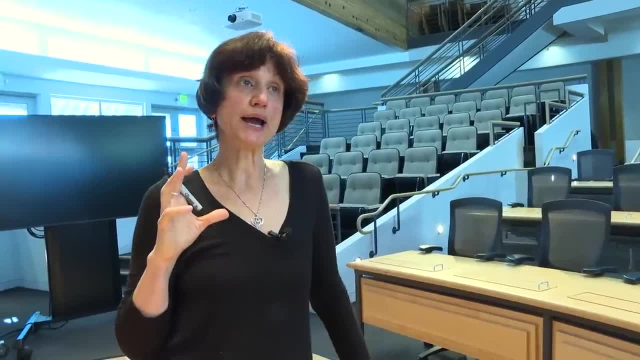 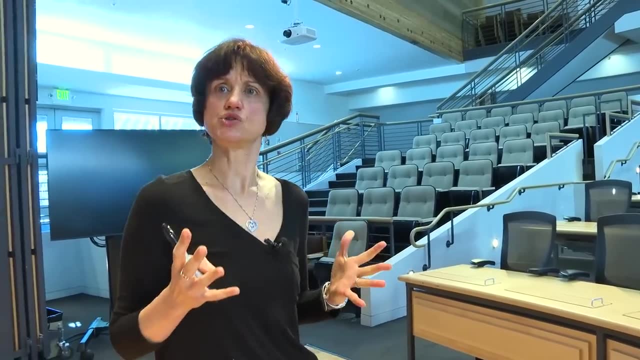 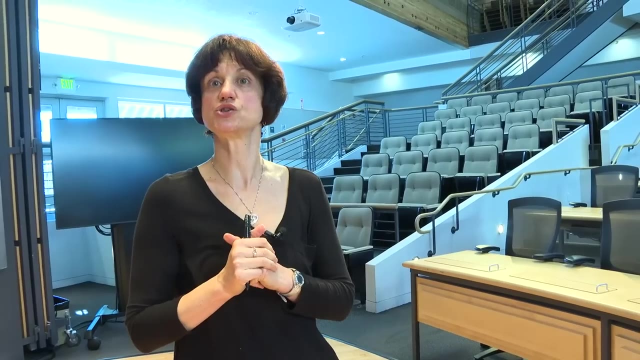 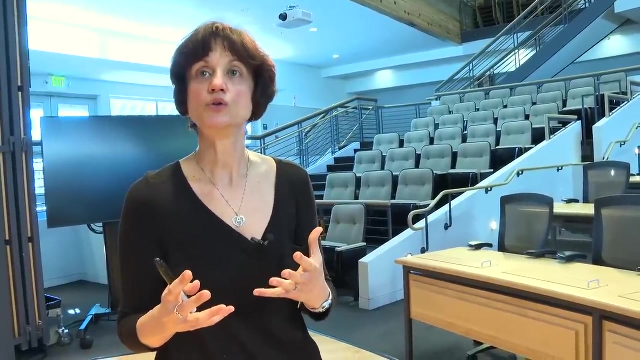 cetera. it means that you are applying induction in disguise. you're just not communicating this to your audience. now, if you were a seasoned mathematician, that would be enough for them. they know how to formally package this kind of situation into induction with induction. you haven't done it before. you may need a little bit of help. 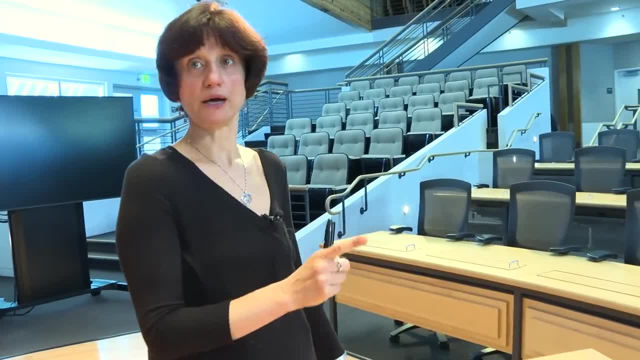 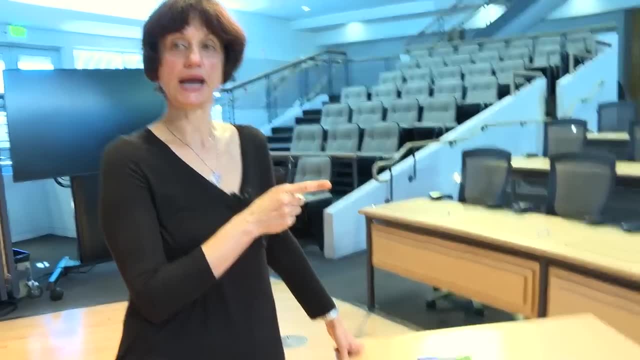 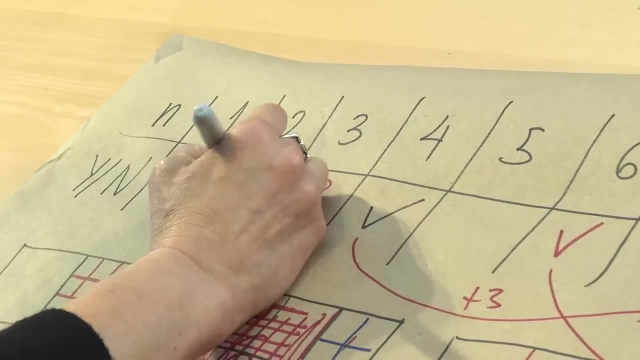 here, And before I show you how to do this formally, I want to answer the questions for the remaining gap. So what is going on with 2,, 3, and 5?? The answer here is no for all three of them. So these are kind of sporadic cases where 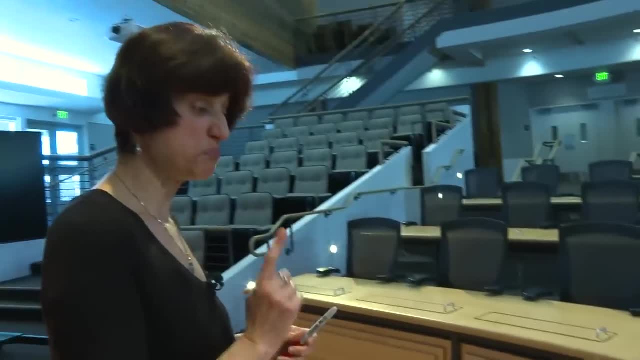 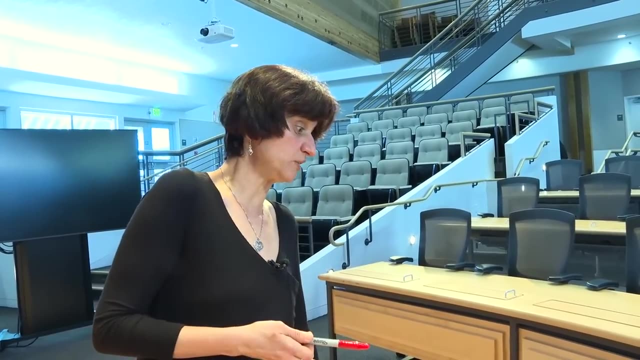 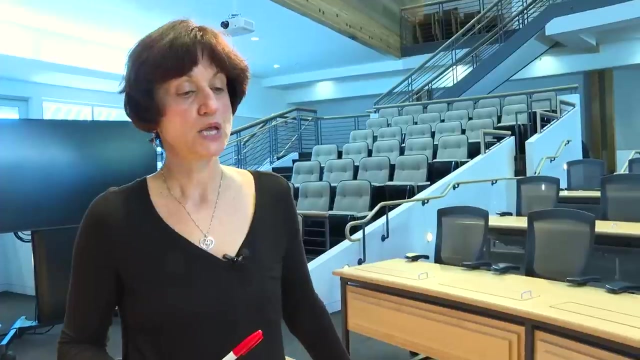 you cannot do it. But the proof that it is impossible for 2,, 3, and 5 is completely different from induction And in fact showing it for 3 may not or may be helpful for 5, but definitely that's not going to be an inductive proof. So 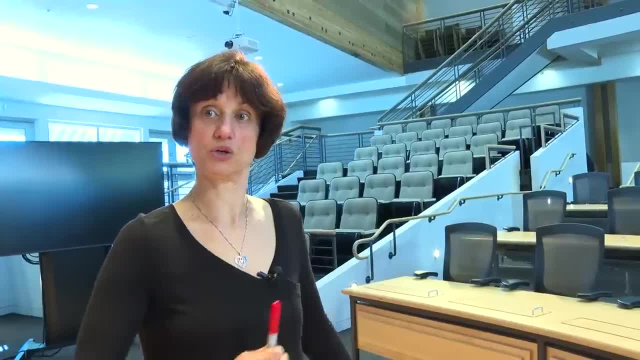 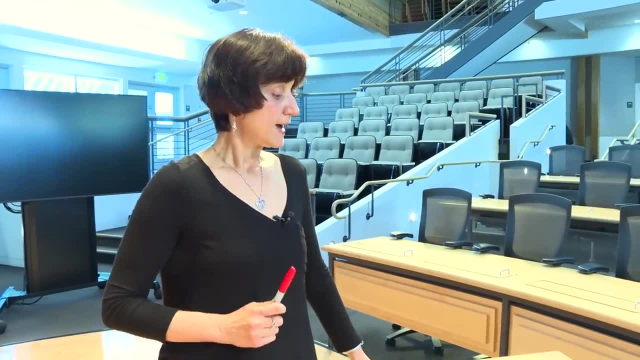 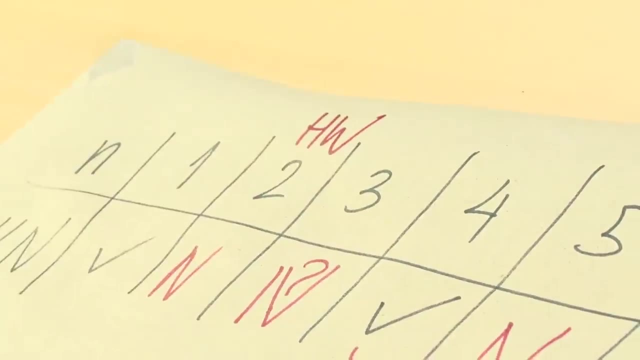 what shall we tackle first? The induction or those sporadic cases? What do you think, Brady? I'd like to get rid of those sporadic cases First. Okay, Yeah, I'm going to leave two for homework, Because after you see the cases for 3 and 5, you may quickly 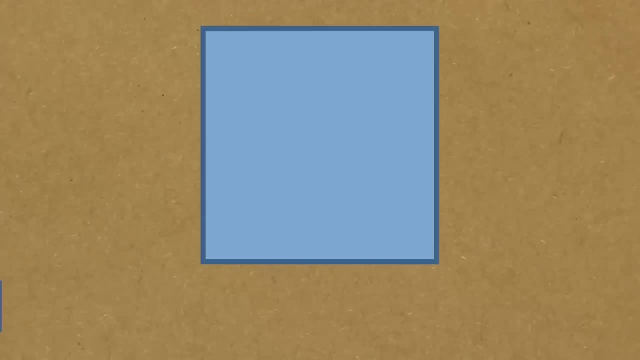 finish off for 2.. So let us see how it works for 3 and 5.. So suppose you can split a square into three smaller squares. So we're reasoning by contradiction. I'm going to use then three of those smaller squares and push. 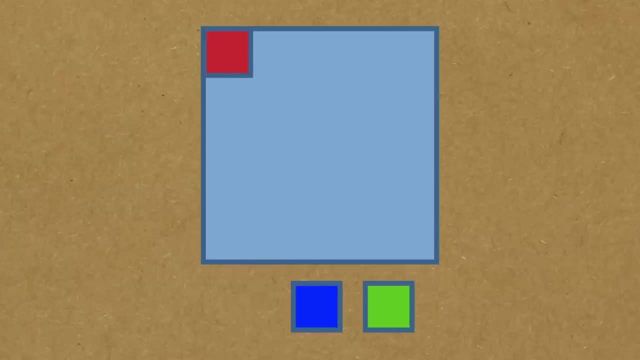 them on to my induction. So I'm going to use then three of those smaller squares and push them on to my. I'm going to use then three of those smaller squares and push them on to my bigger square, So this is the one I want to tile. There's some ground rules here. 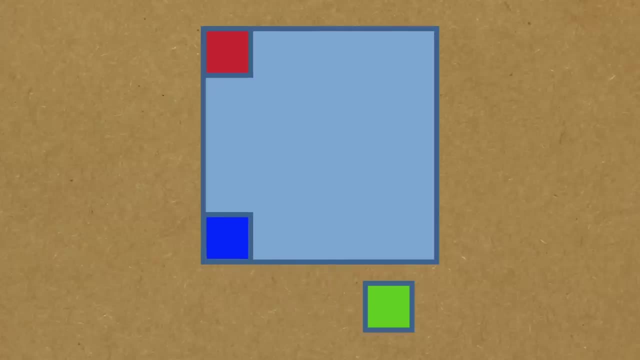 There are corners in my big square. Well, how many little squares can I use in a corner here? Can I use two? I don't think so, Because once I start doing things like that, it's going to come out of my big square, and that's no good. What we. 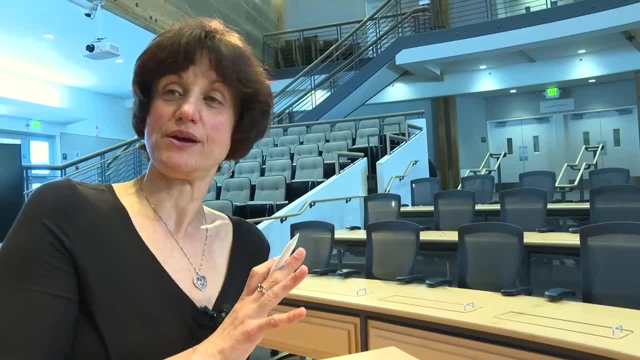 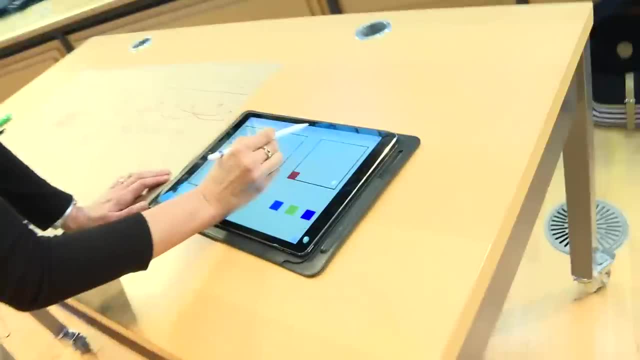 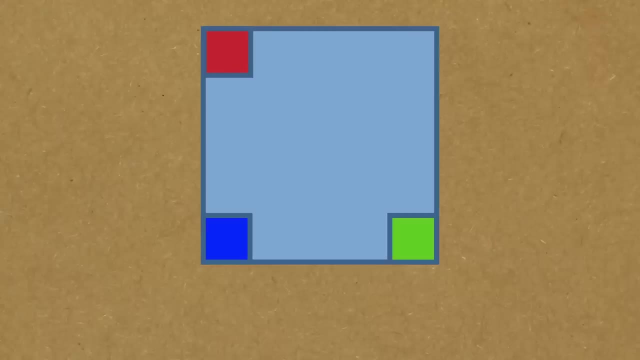 conclude from here is that every corner of our square will be covered by exactly one of our smaller squares, of our smaller squares. That's what everyone should agree on. Okay, but then we are in trouble, because how many corners do I have? Brady, You've got four And I have. 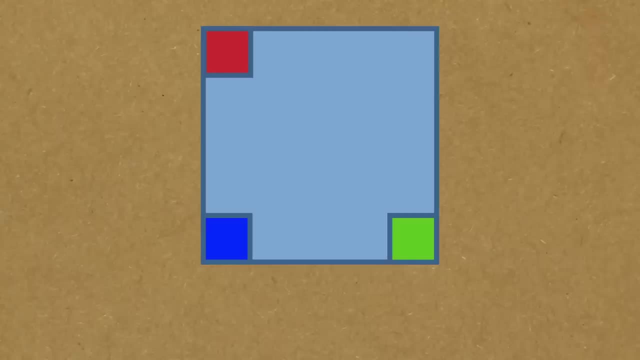 how many squares did we say You're aiming for three, For three. So what must happen? One of those small squares better cover two corners, or else we just can't do it. Let's say the green square is going to cover the remaining corner, but what? 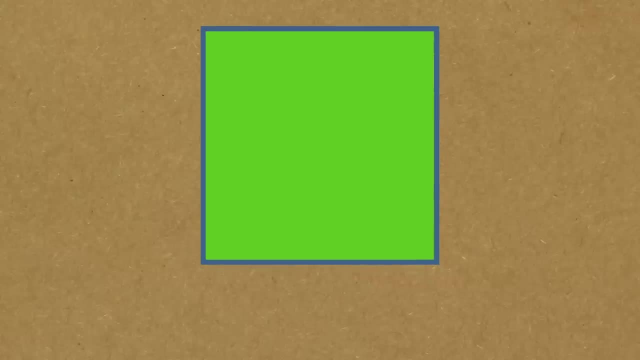 happens then Overlaps, Overlaps and I cover the whole thing with it. Well, that's against the rules. Now let us do it with five squares and show that it is impossible for five. We have four corners, so in this case we have an excess of one little square, And 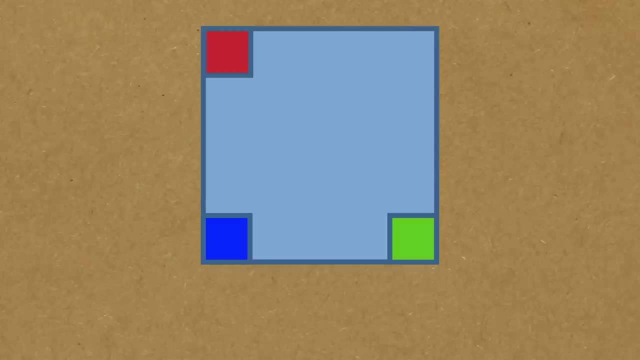 as we reasoned before, I cannot have a single square, like the green one, cover two corners, because it will cover the whole thing immediately. So somehow the fifth square has to be two corners. So I'm going to cover the whole thing immediately. So somehow the fifth square has to be two corners. So I'm going to cover the whole thing immediately. 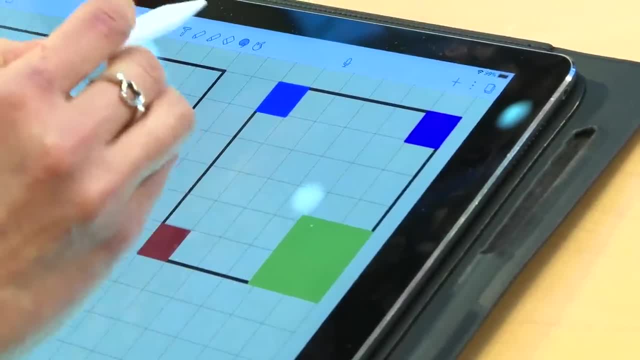 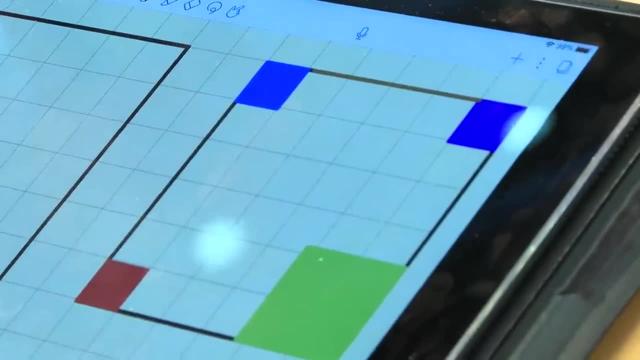 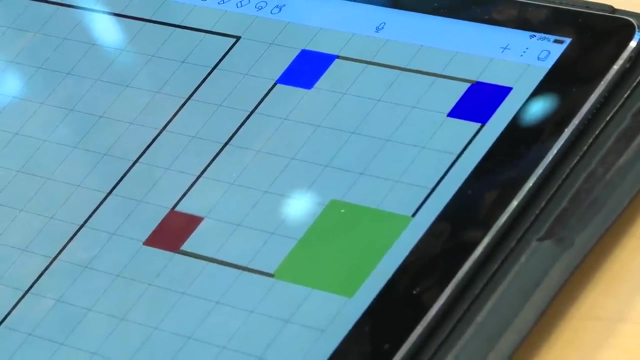 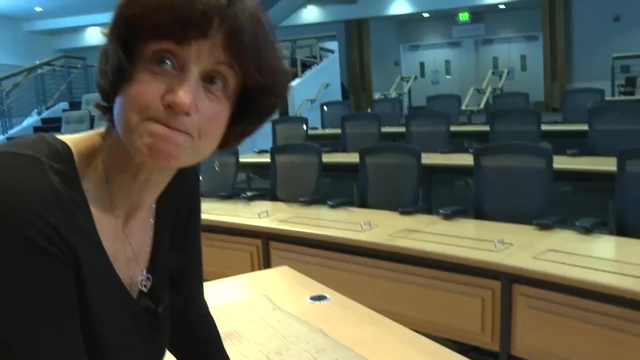 between the others. Hmm, But now I have leftover sides, like right here between those two adjacent squares, So I need to cover those parts too. Is it possible for one small square to cover two opposite pieces like that? Only if it's the size of the whole square Exactly, and I will let this for you to. 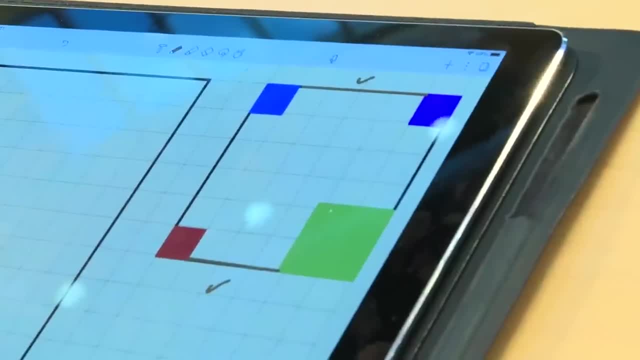 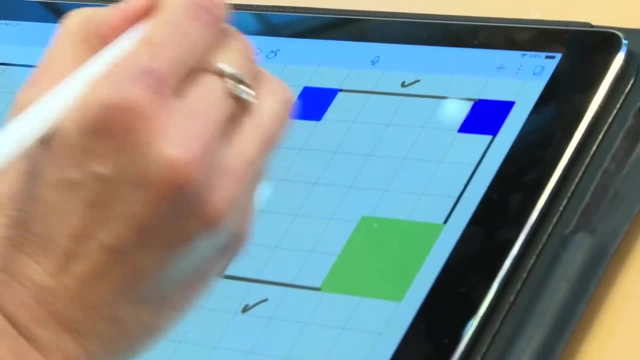 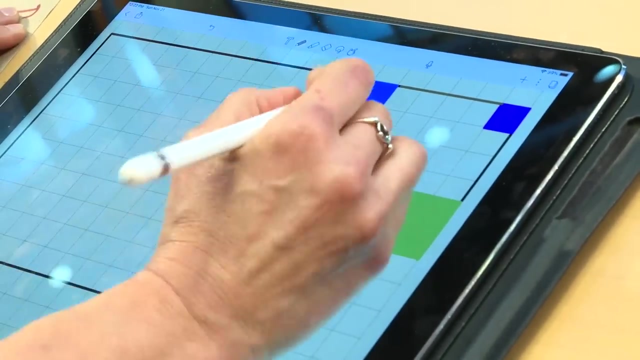 play around and see. see, It's just going to cover the whole thing. So our fifth square is going to dominate everything and immediately show a contradiction. Okay, we still don't lose hope. We say: okay, we cannot cover two opposite ones. Maybe I can cover two adjacent pieces. What will happen In that case? 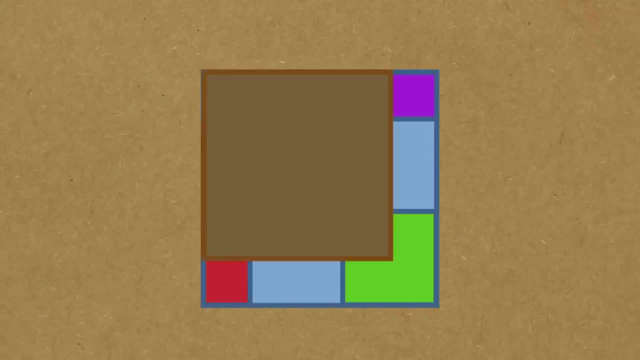 it means that this brown fictitious square, well, its sides still have to meet. It's going to go over our blue square and we don't want that. Again, we don't lose hope. We say, fine, I'm just going to restrict to covering only one piece on the side with my fifth square. 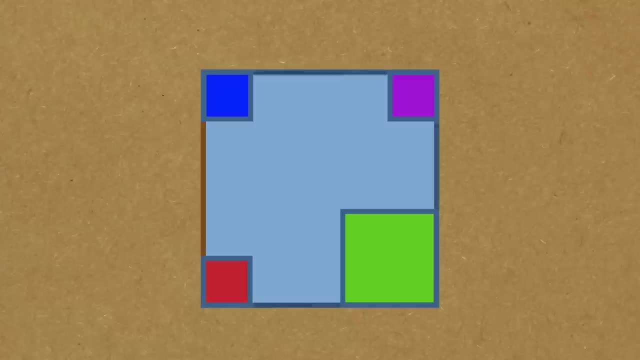 But that means that all of the remaining black pieces here have to be covered by the original four squares, So I have to enlarge them in order to do this. Okay, so I will start enlarging the purple and the green one. They don't have to meet in the middle, They can. 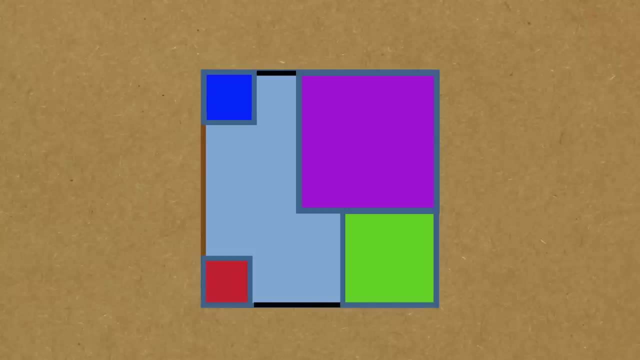 meet a little bit off like that, That's fine. I can start enlarging the blue one, Yes, And I start seeing trouble Now. the red one is supposed to meet at least the green or the blue one, not both, right, But if it starts meeting, let's say the green one, what do we see? We have covered. 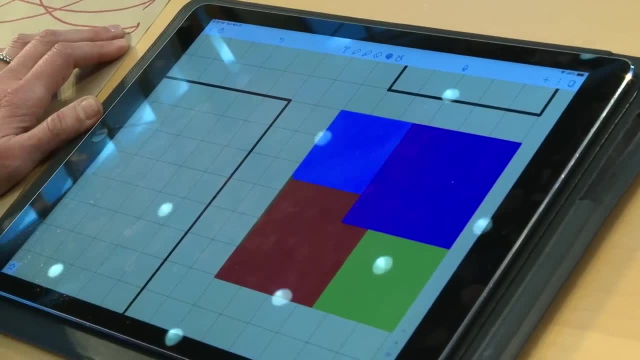 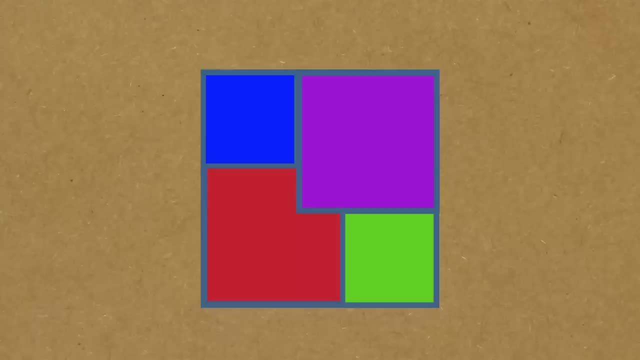 everything. There is no place for a fifth one and we are overlapping. If I do, for example, try to meet the blue one, I'll again do the same thing. So you need to label the sides, probably x, one minus x, and so on and so forth, Go around and really complete this argument, But visually. 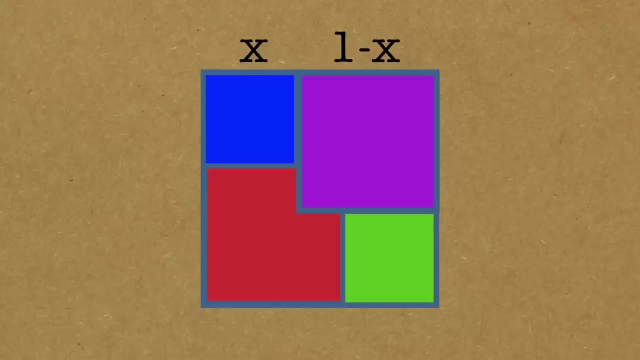 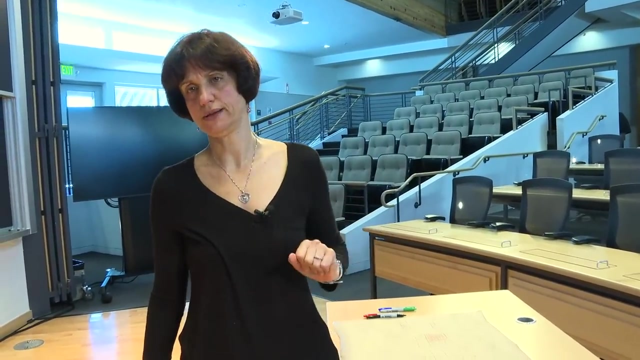 it is obvious. there is no place for the fifth square anymore. So we cannot do it with five, We cannot do it with three And for homework, show that you can't do it with two. Now, where is the induction? Now, where is the induction? 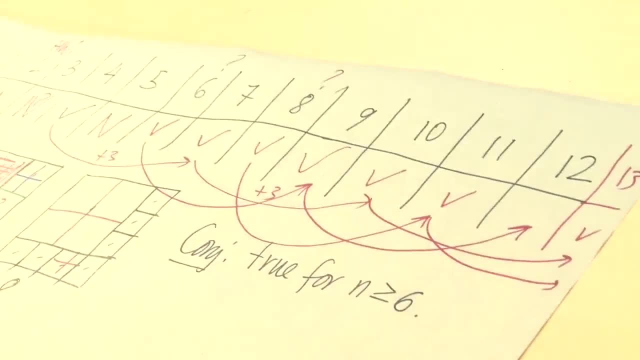 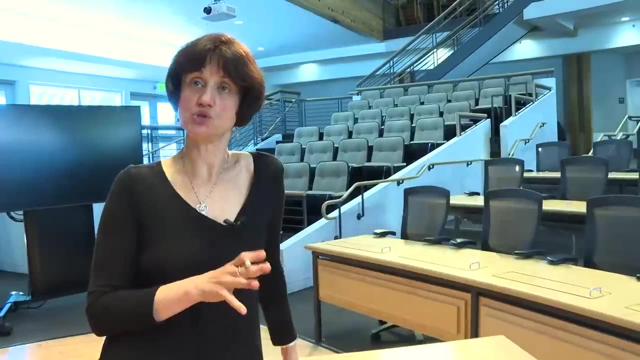 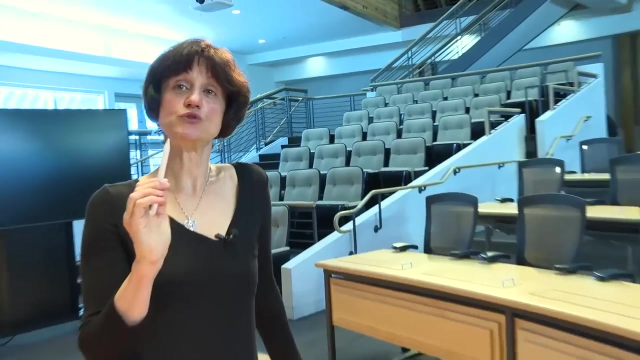 Here, Mathematicians will tell you that if you can prove a statement without induction, in other words directly, go ahead and do it. But you may not see that direct way, And that's why I'm going to demonstrate for you something called strong induction. We need strong. 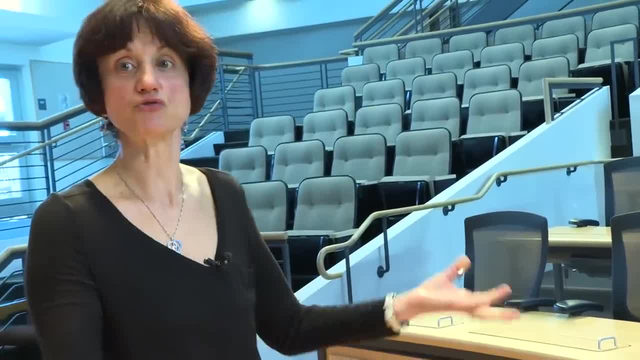 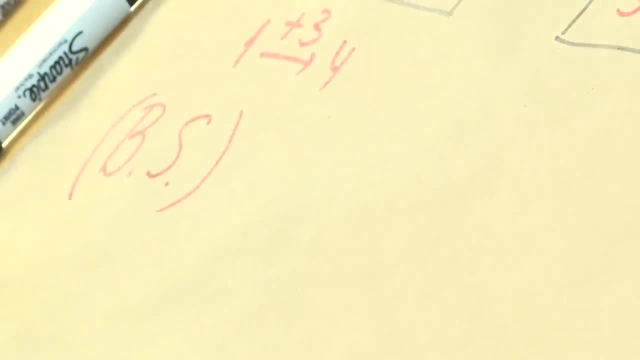 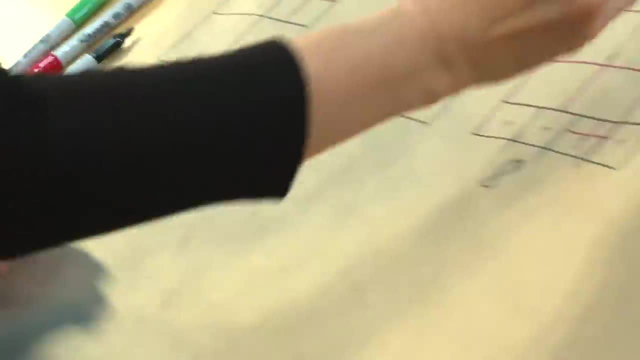 induction here in order to technically wrap up this solution. So how does it work? What is our base step? It turns out for strong induction you may need several base steps And you can easily convince yourself that you will need three base steps for six, seven and eight, And 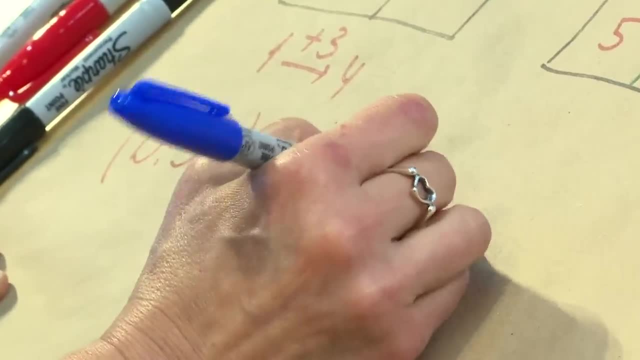 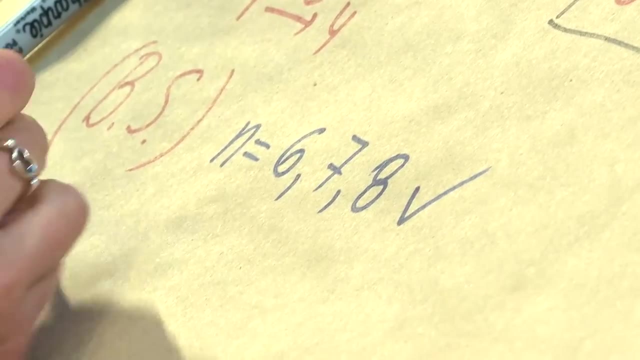 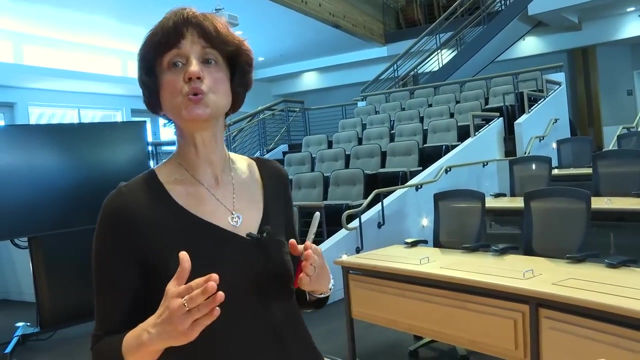 you will say: n equals to six, seven and eight, And you will demonstrate, for all these three cases, which we already did Now, what is the inductive hypothesis. Now, this is going to be tough because I'm going to seem to assume more than what I did before. But in fact, these 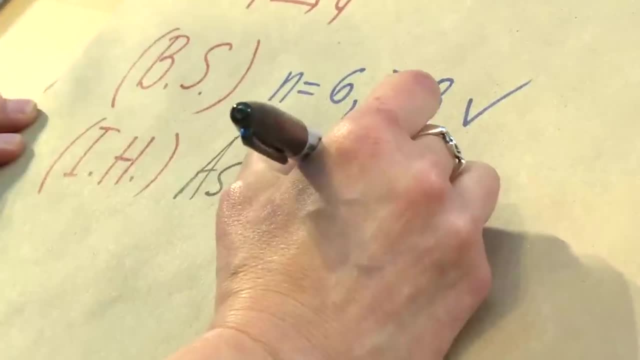 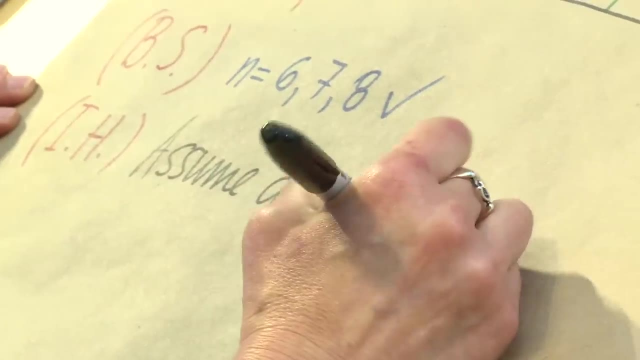 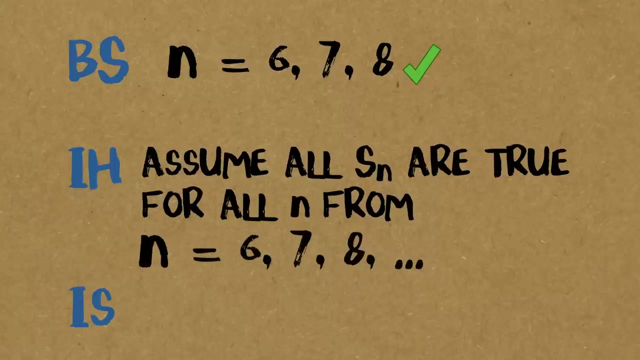 are equivalent methods, So I'm going to assume all statements as a game. where n is the number of small squares are true for all. I am from six, seven, eight up to somewhere. let's call it K. so I'm just not gonna tell you K, but they're going to be taught From 6,, 7, to 8, up to somewhere. let's call it K. 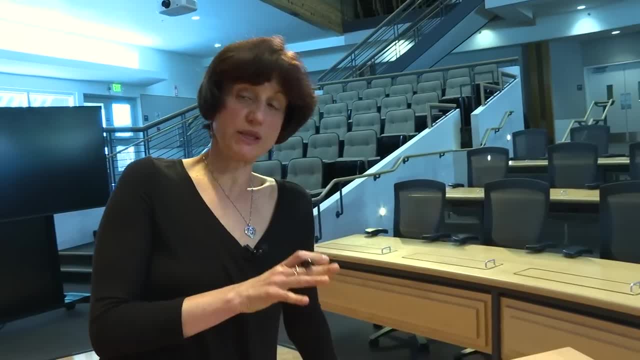 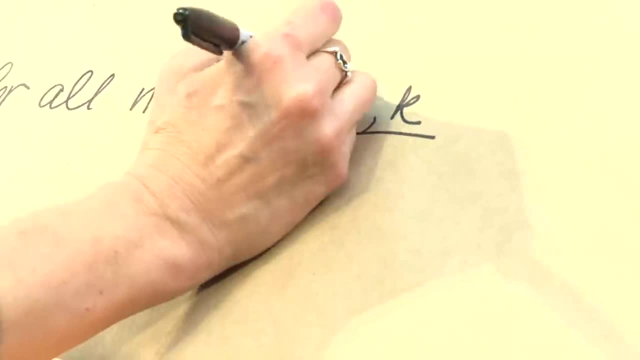 let's call it K. So I'm just not going to tell you K. But note what I have just done. I have assumed a whole bunch of statements, including my three base cases. If K is 8, we are done. I'm not doing. 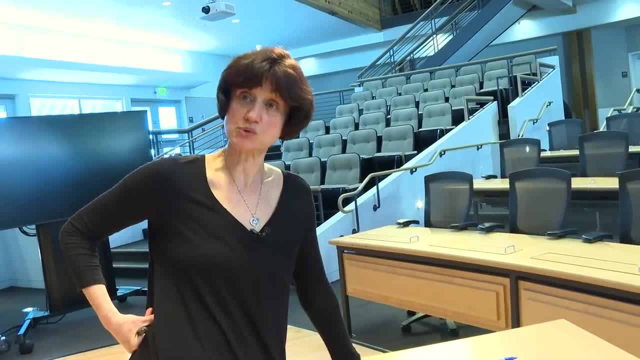 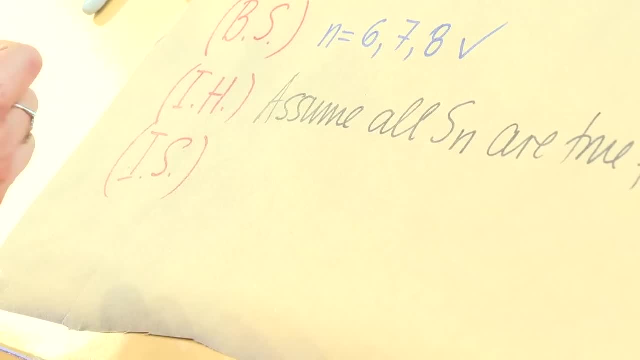 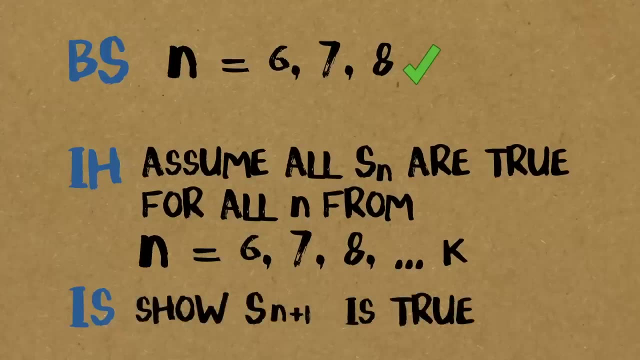 anything extra. But if K is more, I'm actually making an assumption. So what do we want to prove in the active step- This is the creative one- We want to show that S sub n plus 1 is true. So what does it mean? That we can go one for the case higher. Now why is this happening? So I have gone. 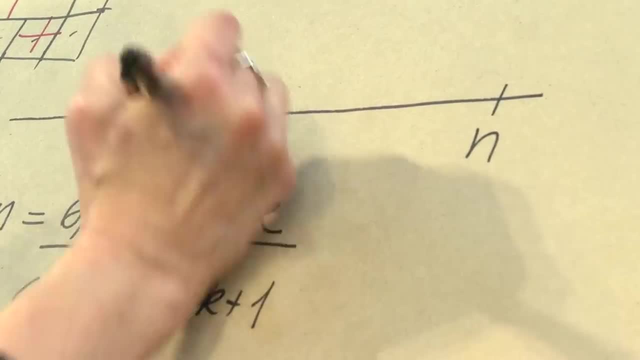 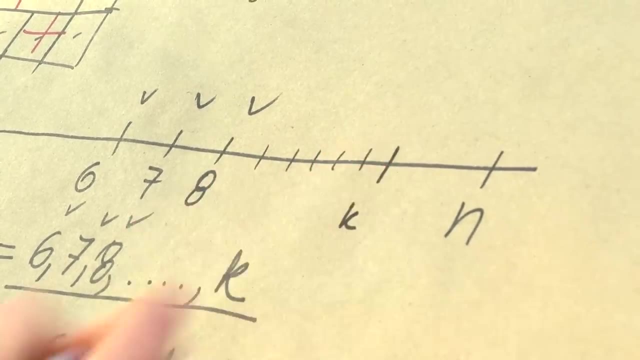 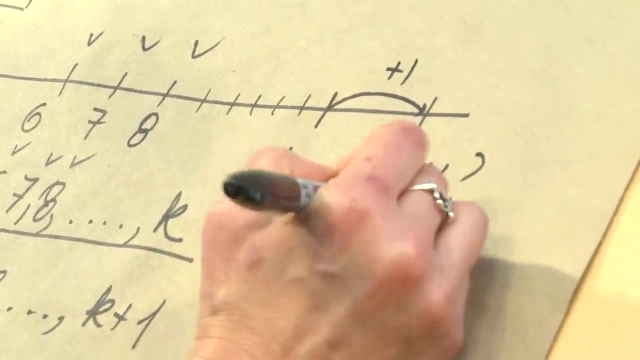 up to n. Just imagine the real line. We know that 6,, 7, and 8 are true, And maybe some more. Let's say up to here This K, And now we want to go one more higher, right? So let's say n plus 1.. As I said, my 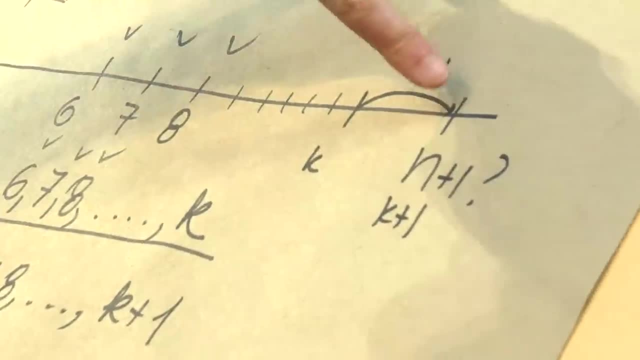 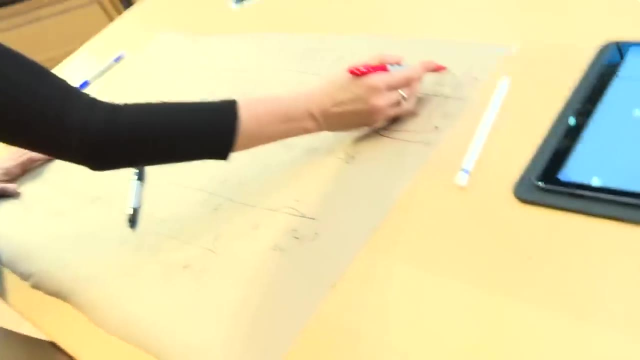 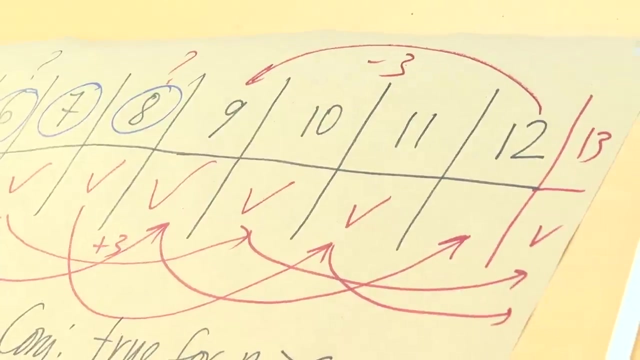 variable is a little bit funky, but that's okay. So why is this case true? As we saw messing around, the initial messing around with the problem- in order to do 12, you wanted to go back with three steps and kind of undo one window technique. And that's precisely what you're going to do here. 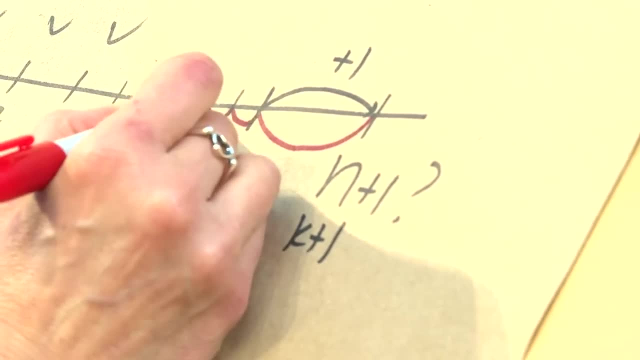 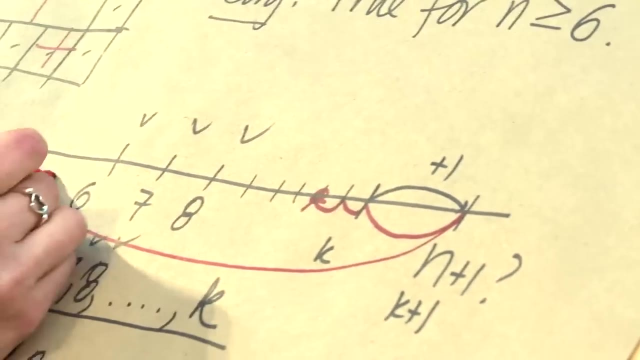 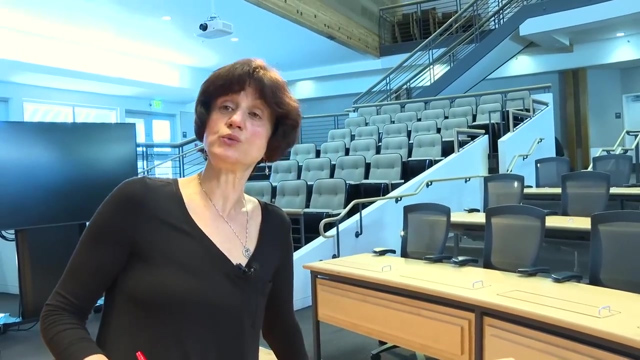 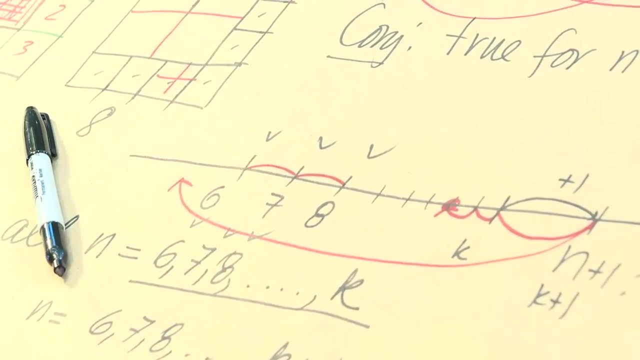 You will go back three steps. Do you still land on a statement that is assumed to be true or did you accidentally fly outside and land it on five, which we know already is not true? The answer is no. You were still within the cases that you assumed were true, because you have this barrier of three base cases that don't. 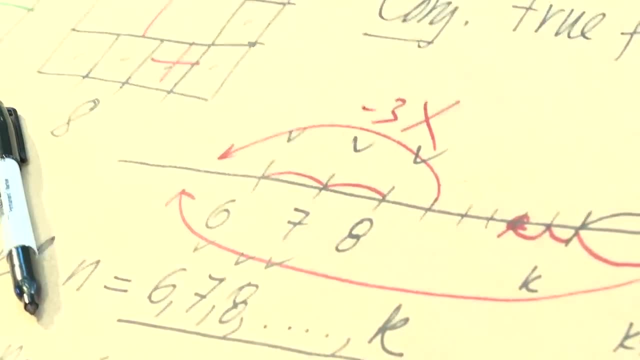 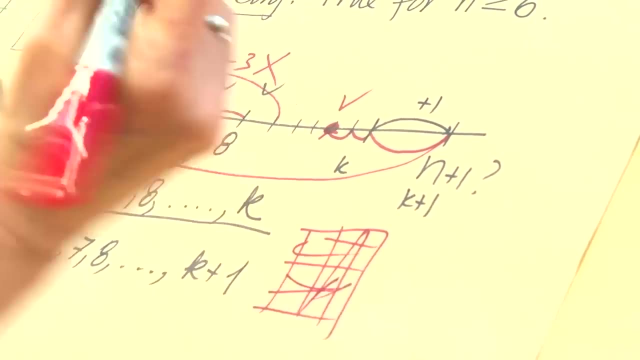 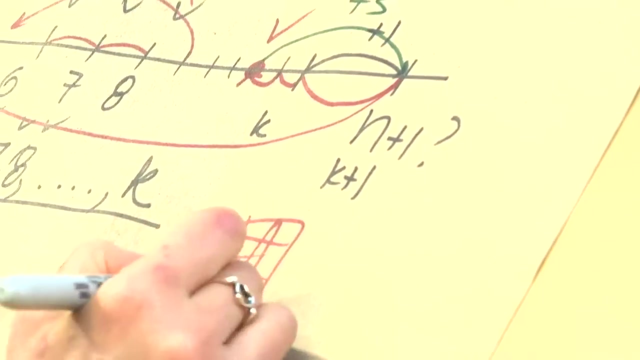 allow you to fly over them when you subtract three. So you again land on a statement that is assumed to be true is true. So you have some square that you have somehow partitioned artistically into sub squares, and all you have to do is go back by adding one window technique. 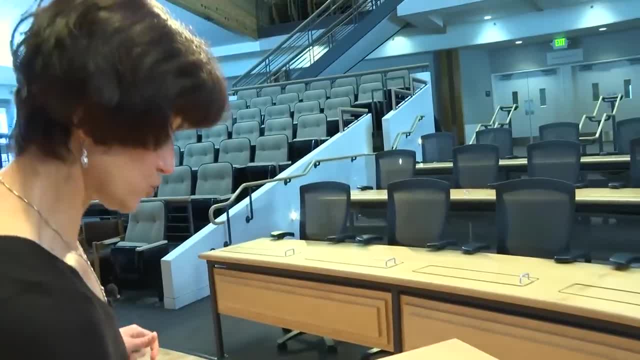 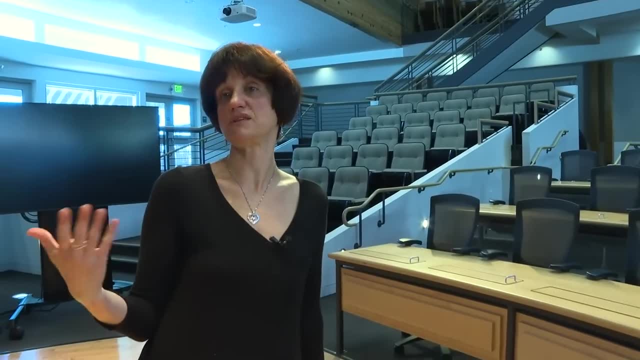 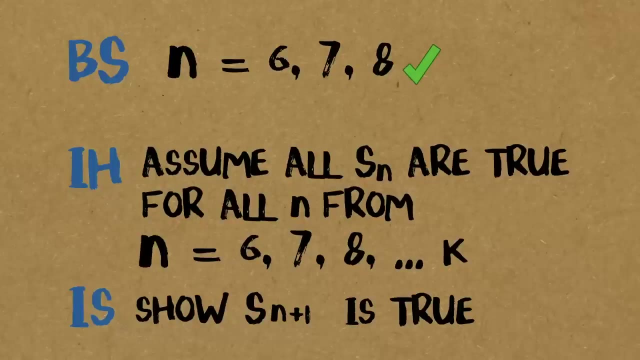 to it and three more, And that way you will show that the next statement is true. and then you will do this magic conclusion by the method of mathematical induction. All of those statements are true. This is indeed using the method of mathematical induction. They are direct proofs. I can give you a. 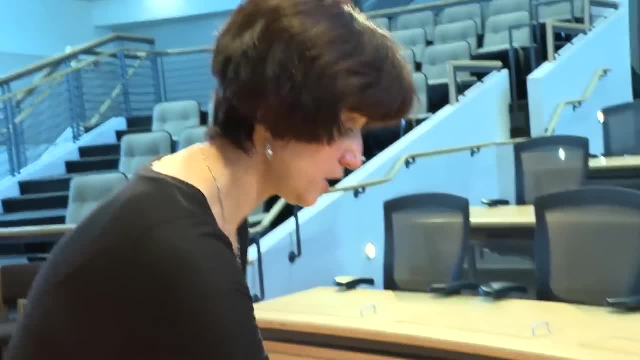 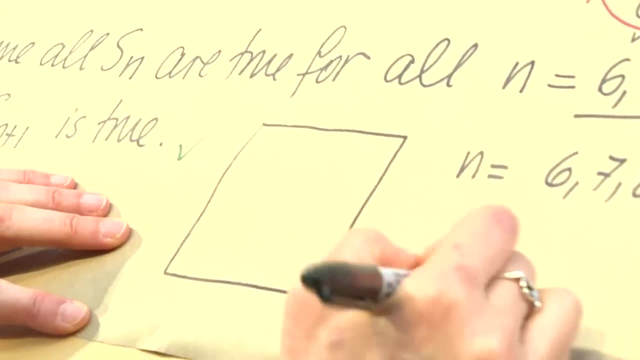 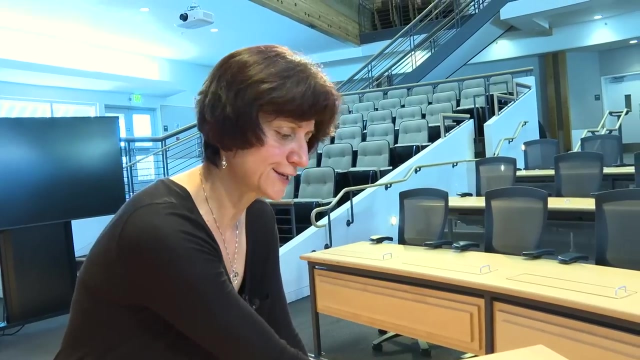 hint. First, do this problem for, let's say, a very large even number. What's such a large even number Like 2,000. Can you directly divide it into 2,000? You can do something like 6 and 8, what we did before. So I will split the sides into: 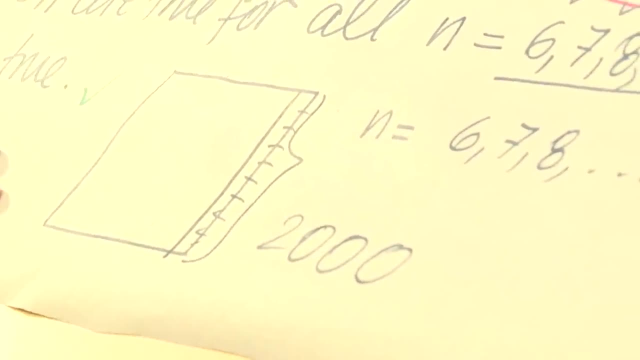 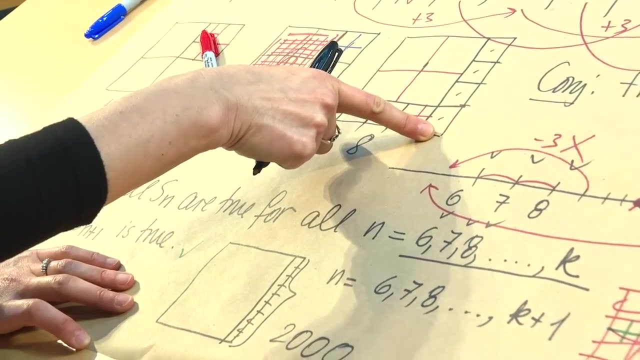 how many sub squares? do you think, Brady? A nice number. Any number, No, it has to work. Oh, okay, See, for 8, we cut it down into 4.. For 2,000, maybe we should cut it. 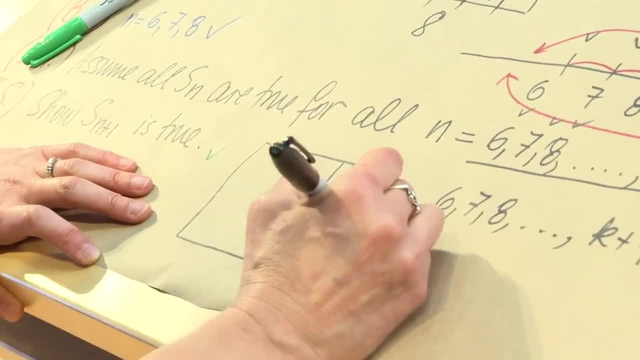 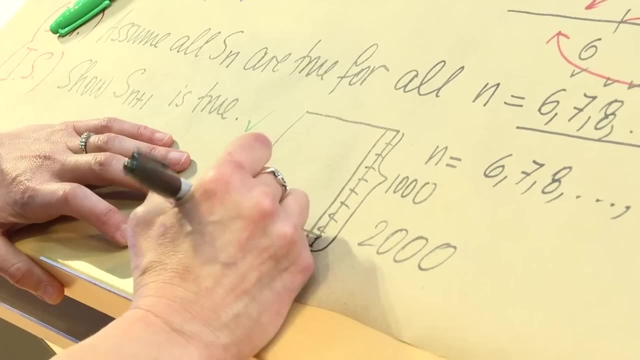 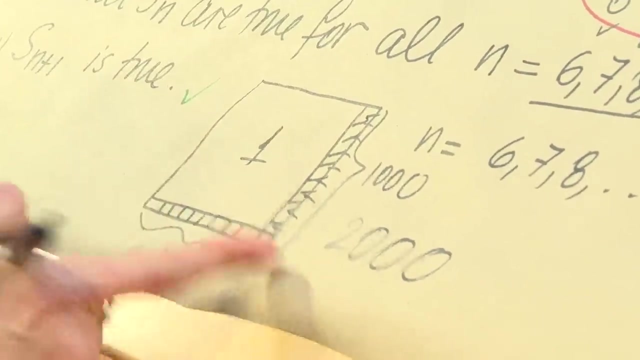 into 1,000.. Yeah, So you're gonna cut the side into 1,000 squares and then you will draw these lines and continue doing your small sub squares and one large. How many do we have? You may think we have 1,000 plus 1,000 plus 1, but you are wrong, because we are 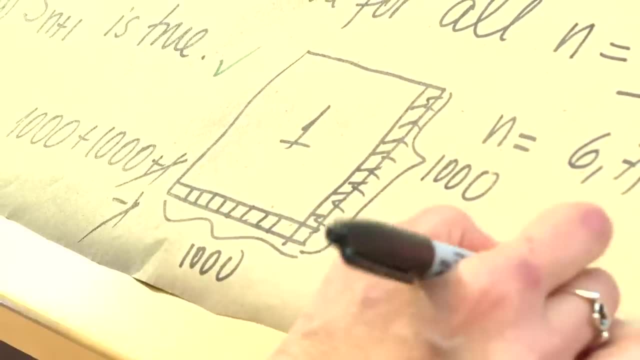 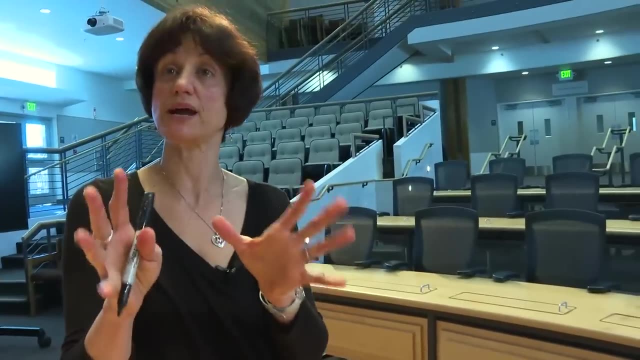 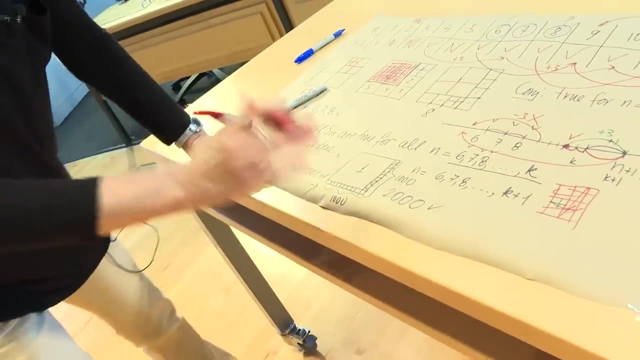 just over counting this corner. So you have to subtract that and bingo, you have your 2,000.. I think this example is general enough for you to try even numbers right away. And then how would you do a not number? If you add 3 to 2,000, you get a not number. 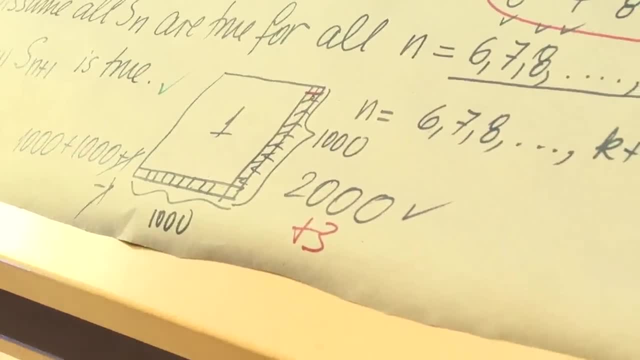 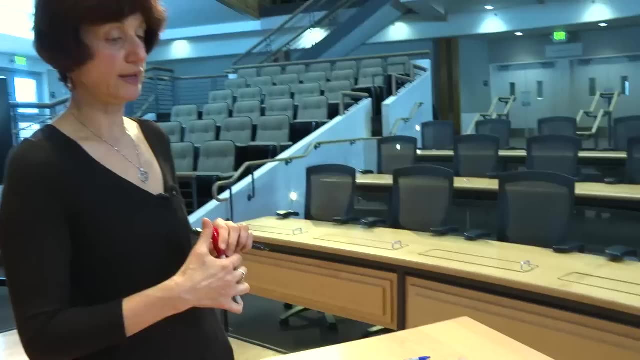 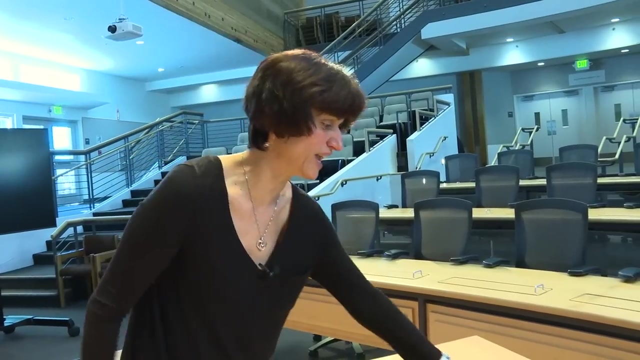 So you just have to hit one of those little squares with the window technique and you will get odd numbers. Okay, So you can wrap this up into a direct proof that will nevertheless use two cases- even numbers and odd numbers- And you still cannot get 5.. There is no way. 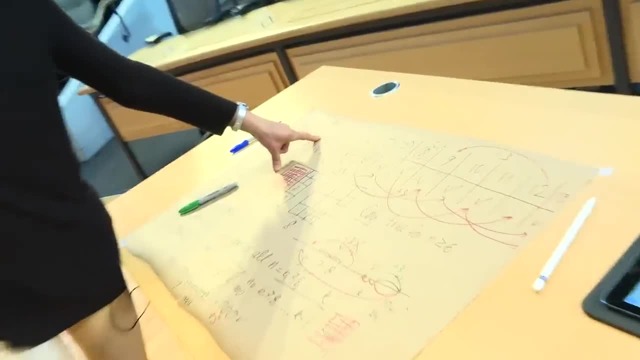 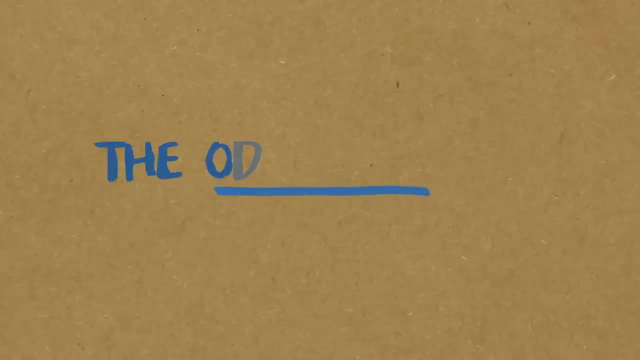 you can get 5, because if you go 3 backwards you're gonna land on 2, and that's the first and only even number for which this is impossible. Subtitles by the Amaraorg community. Let's try to throw pies at each other. I'm sure you have seen those old black and white. 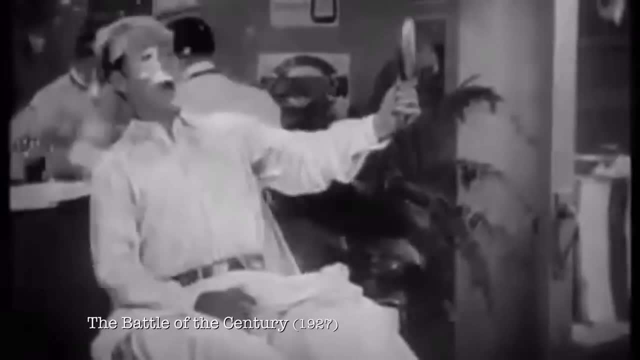 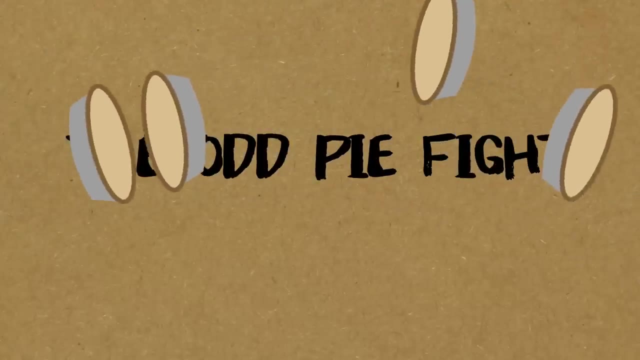 movies where everyone's having fights and pying each other. Not 3.14 pie, actual pie, Actual eating pie. And the funny thing is we're gonna call it the odd pie fight. but it's not that the pie is odd, but the number of people involved. 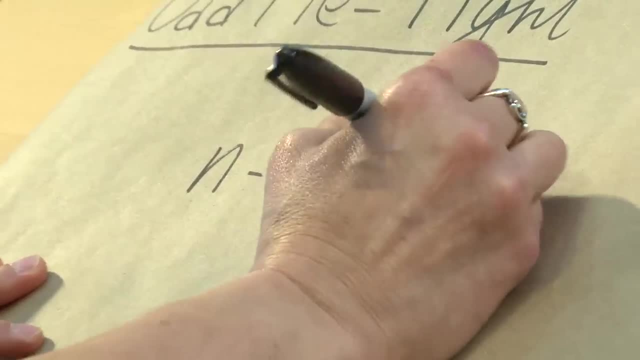 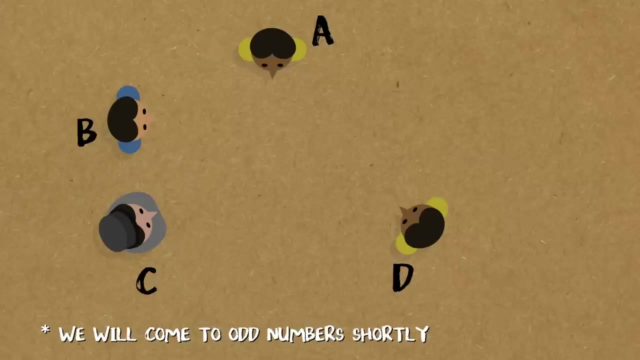 is odd. So you have all the number of people and they're standing somewhere so that no two pairs have the same distance. So if I take any two different pairs of people- A B, C, D- I will see that A? B is not equal to C? D, And this also applies to the same person. For example, A D here. 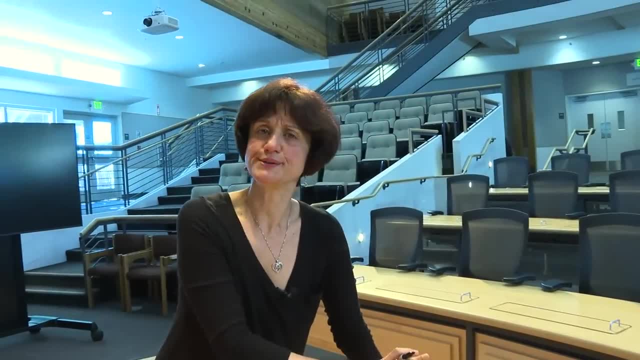 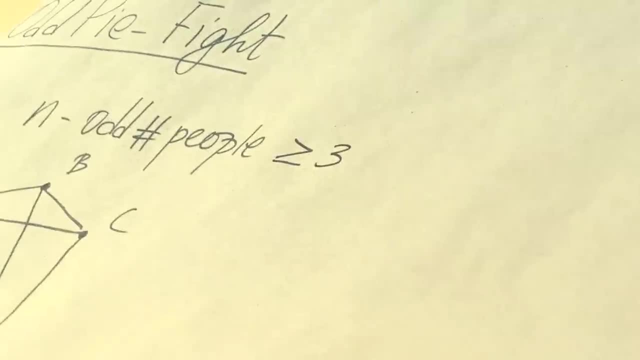 has to be different from everything else. Subtitles by the Amaraorg community. Subtitles by the Amaraorg community. The distances are different. You have odd number of people and let's make it interesting, at least three, because for one person you're not going to pie anyone. And what do they? 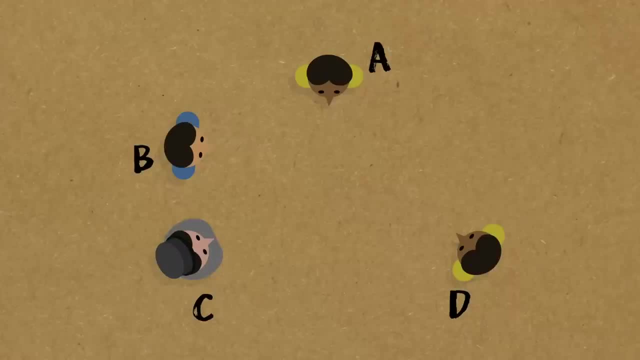 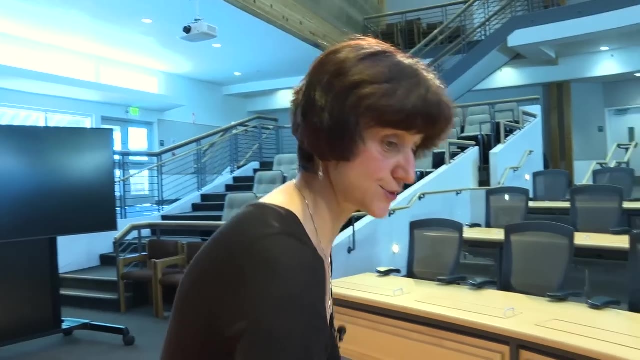 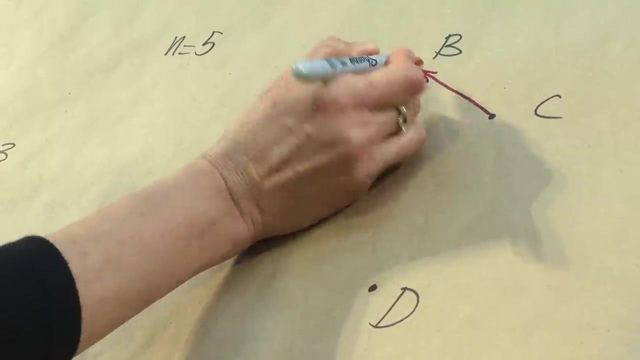 do. Every person looks at the closest to them other person and pies them. For instance, there are five people here and it looks to me that C is closest to B. C is going to pie B. What's going to happen to E? 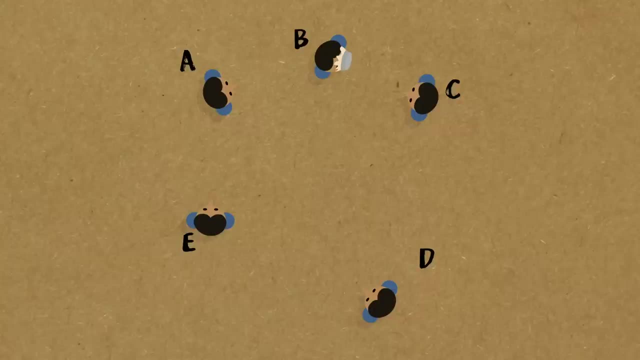 what's gonna happen to E? E looks like he's going to pie A. A probably is gonna pie B. B looks like he's gonna pie C And D. D is very far. I don't think anyone is pying D. 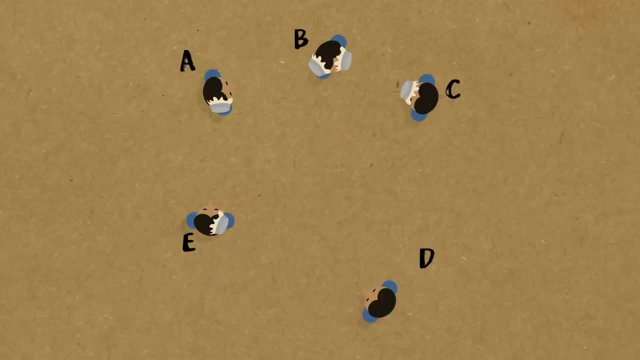 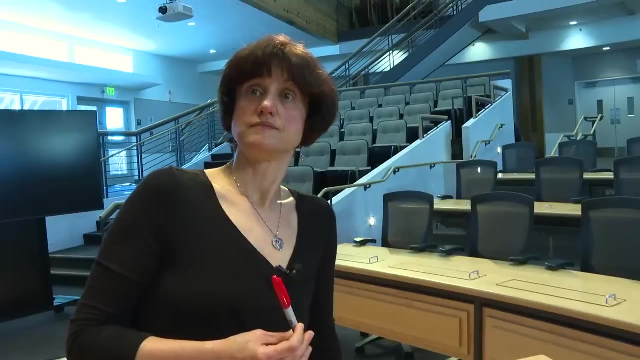 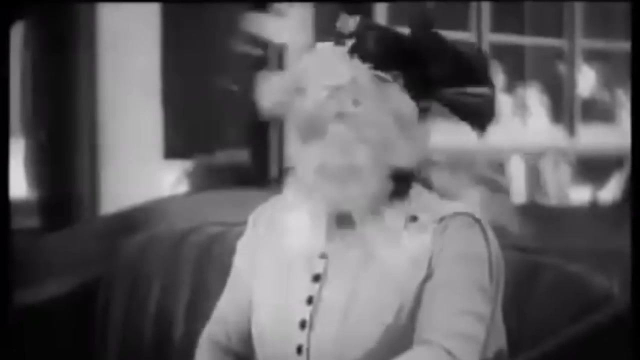 but D has to throw to someone. I don't know. maybe E All right. if you were in that fight, what would you like Brady to happen to? If I was in the fight, I would want to not get pied Correct. So do we have a survivor always? In this picture we can see that. 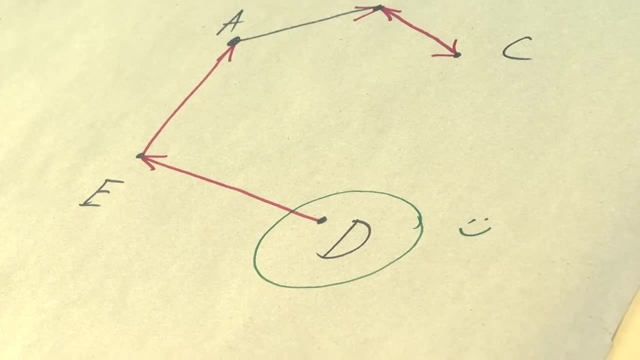 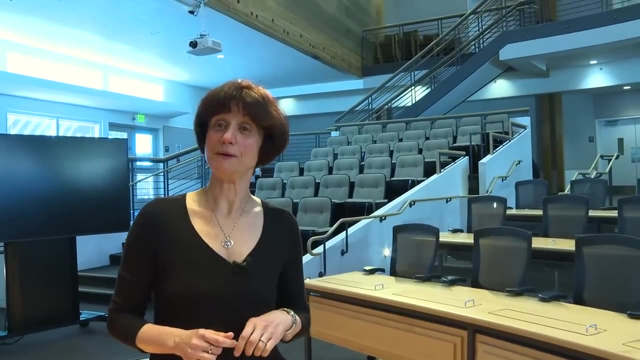 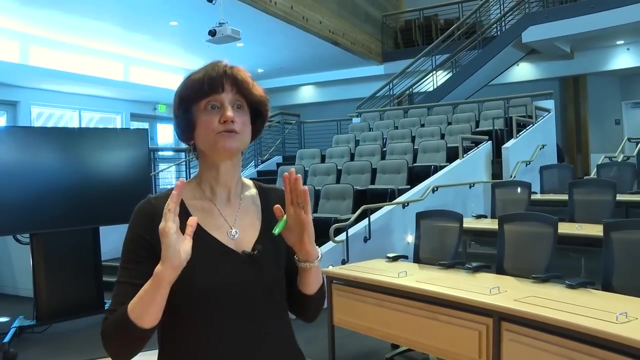 D is definitely a survivor, but does this always happen? Unpied, Unpied. So that's the beauty of the problem: Under these restrictions, odd number of people pairwise, different distances- there is always a survivor. So let's write this: 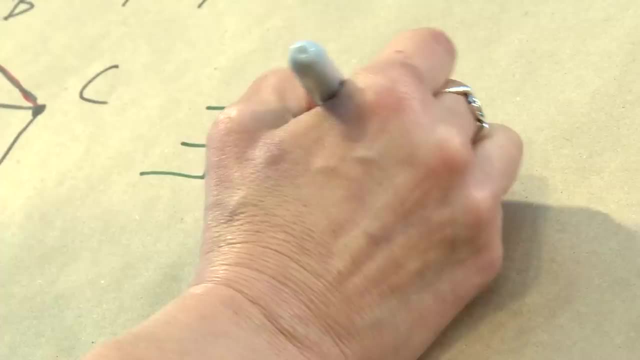 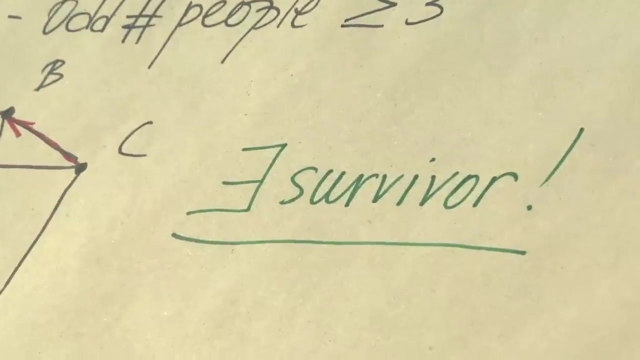 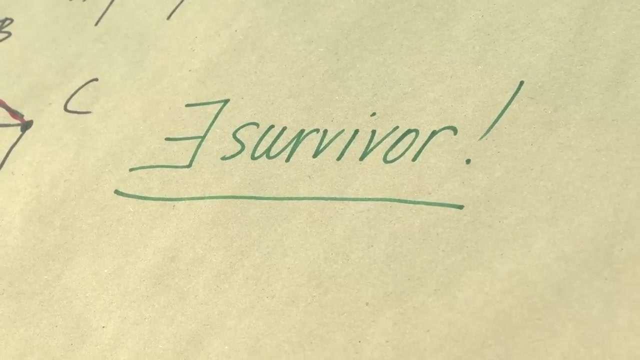 Conclusion: There is always a survivor. I'm not claiming uniqueness or any other funky things. There is always a survivor. I've not seen that symbol before. Oh, Brady, we're learning every day. Yeah, There exists a survivor. And you look at this and you say: how can this have anything to do? 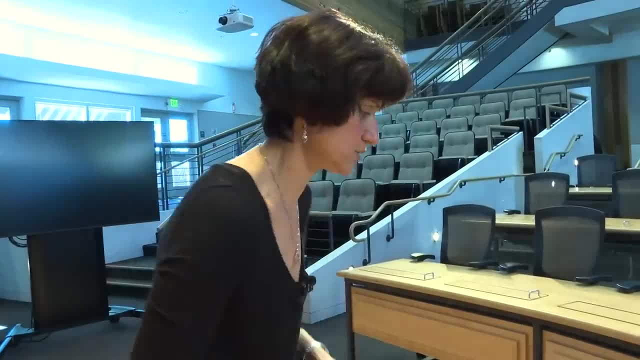 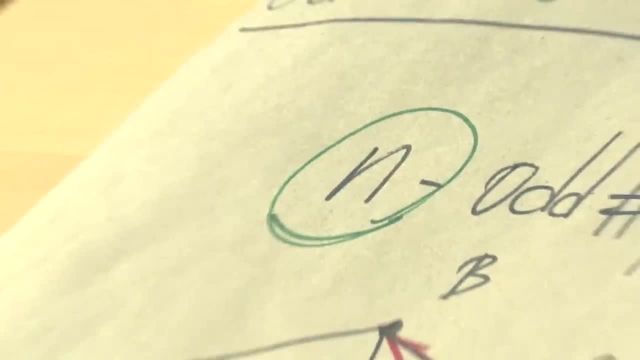 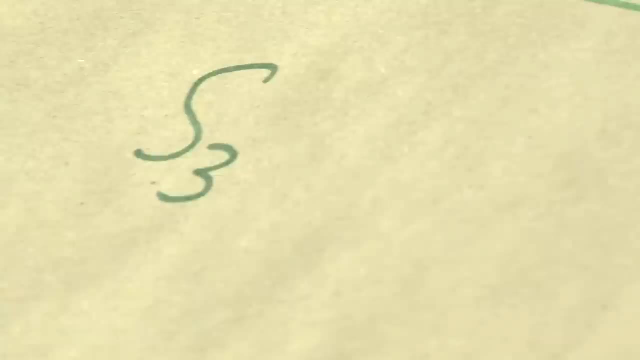 with induction. Of course it has something to do with induction, Most likely because there is an N. These are infinitely many statements. This is like the dominoes. But which statements are we really concerned here? We want S3 to work for three people, We want S5 to work S7, et cetera, et. 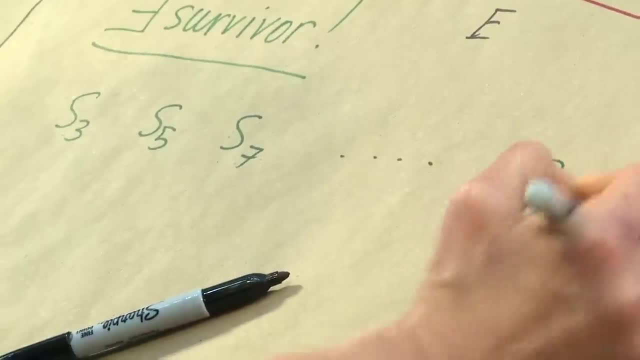 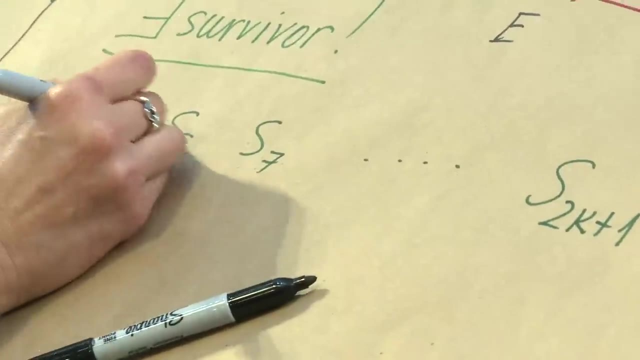 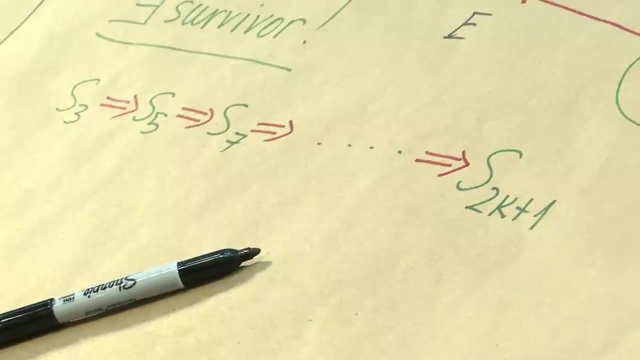 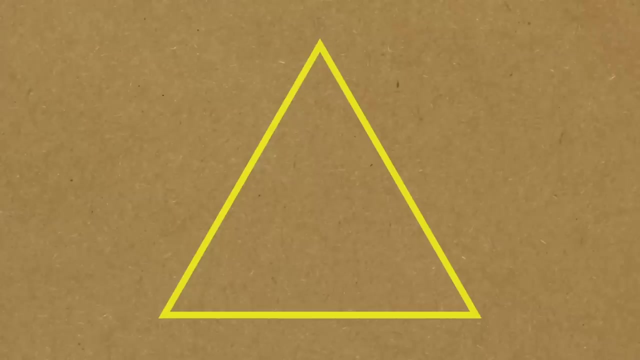 cetera, S sub 2k plus one. All of the odd statements And induction will help us show the implication. or, if you remember the evil spell, We're going to keep on flying like that, All right, So let us see how this works. All right, What's the base step for? 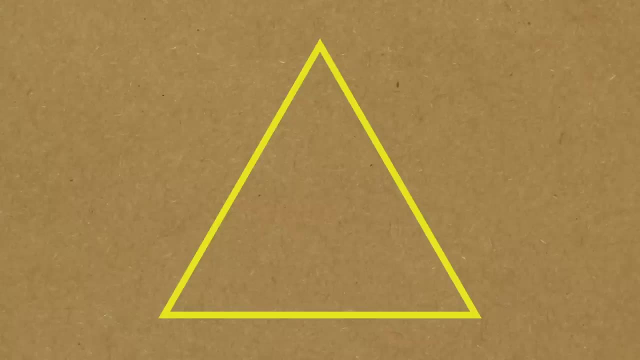 three people. What kind of triangle can this be? It definitely cannot be equilateral. Can it be isosceles? No, No, no, no, no, That's right. So it has to be something called scalene, right We? 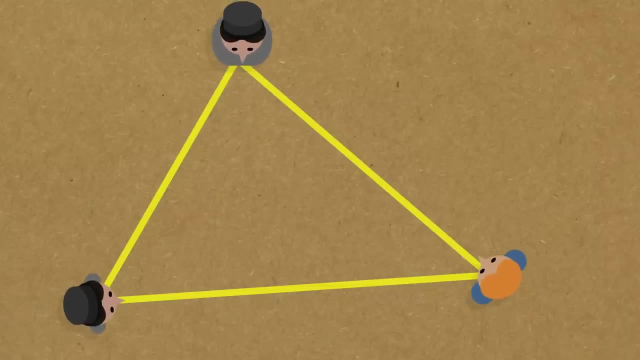 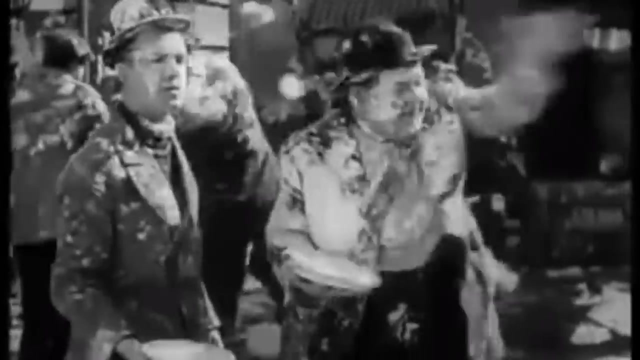 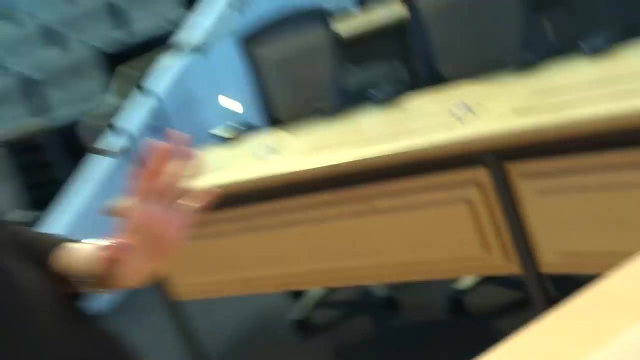 will label vertices here. You know in those old movies, Laurel and what was the name? Harry Hardy, Hardy, Hardy and Laurel, So let us use L and H for them. I have L and H like that, And Brady's going to complete the picture. Wow, I've just joined the most famous duo in comedy history. 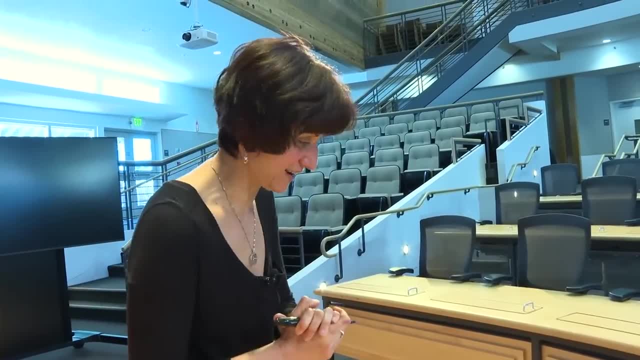 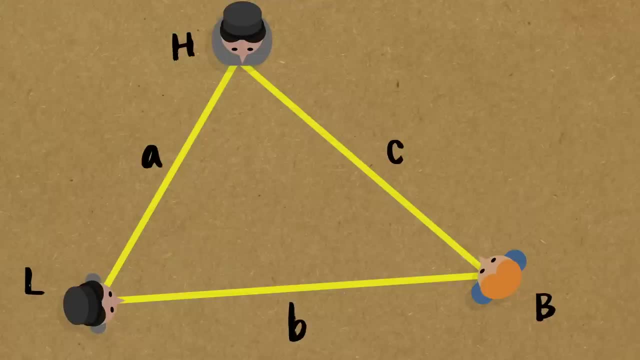 Yep. So in this love-hate triangle, what's going to happen? Since it is a scalene triangle, I have three different sides And, without loss of generality, as mathematicians like to say, I'm going to say that A is. 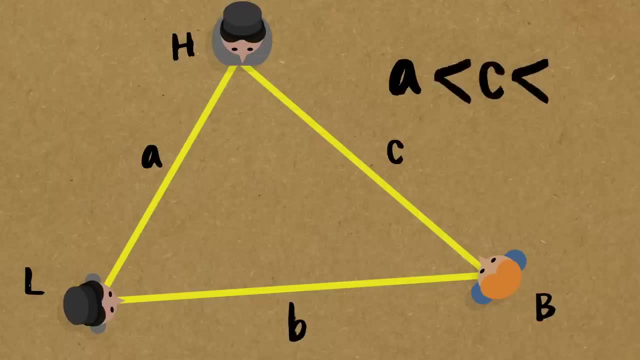 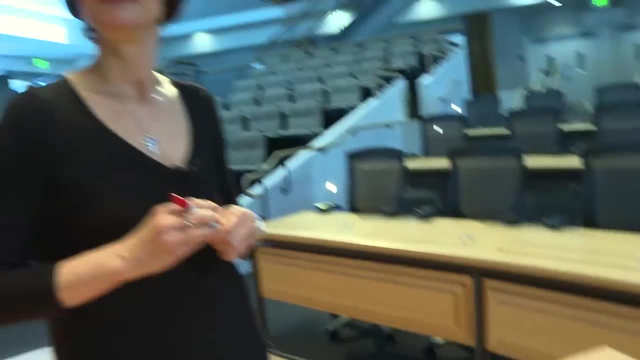 A is. A is What do you say? less than C, less than B, something like that? Okay, So A is the smallest, Exactly. So what's going to happen with the L and H? They're going to pie each other. 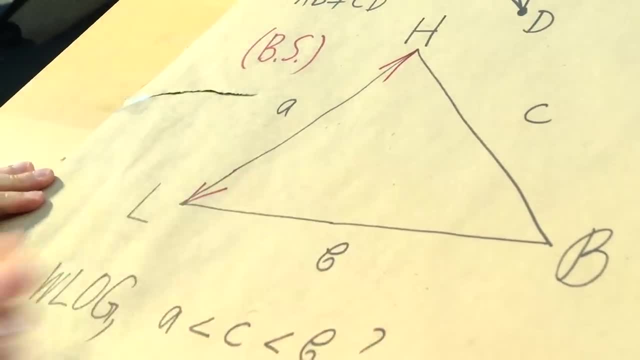 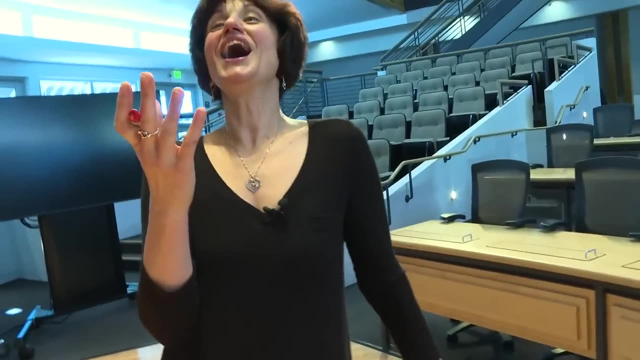 Yeah, Laurel and Hardy are pieing each other and Brandy is watching from far away. What is Brandy? Brady, You got Hardy wrong. you're allowed to get Brady wrong- Absolutely, But that B person. what is he going to do? 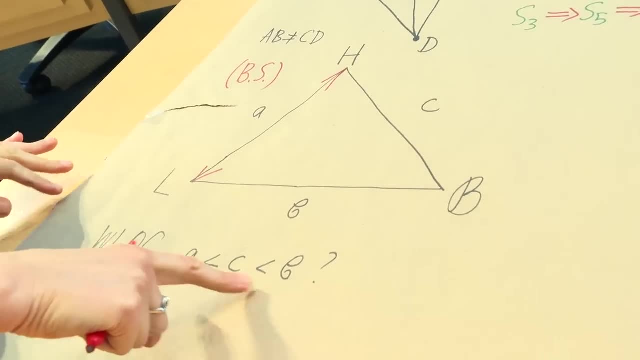 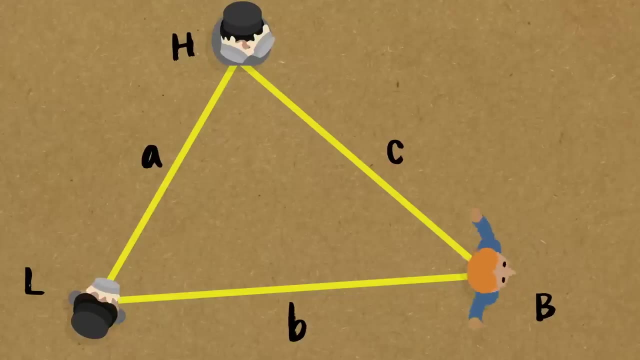 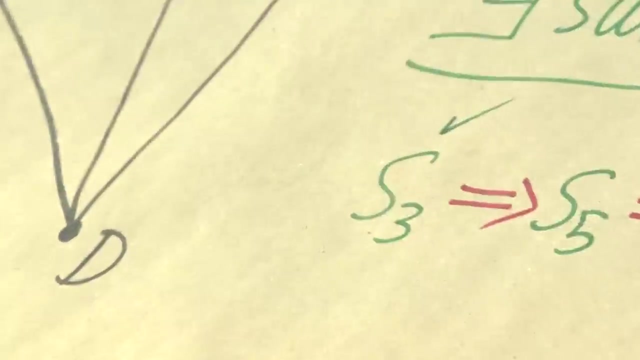 Well, He, He had to pie someone and it looks like C is less than B. So Hardy gets pied twice and we have a winner: Brady survives. Great, We've done S3.. Now, by induction, We know how to proceed: Inductive. 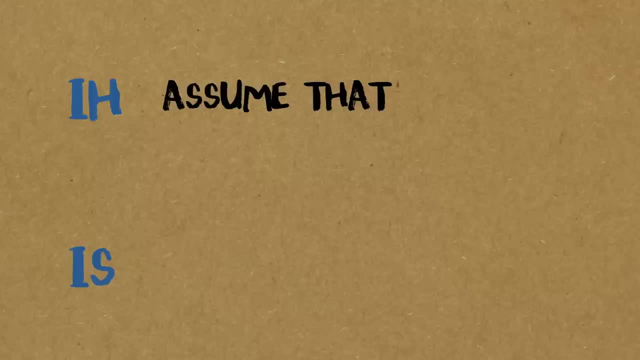 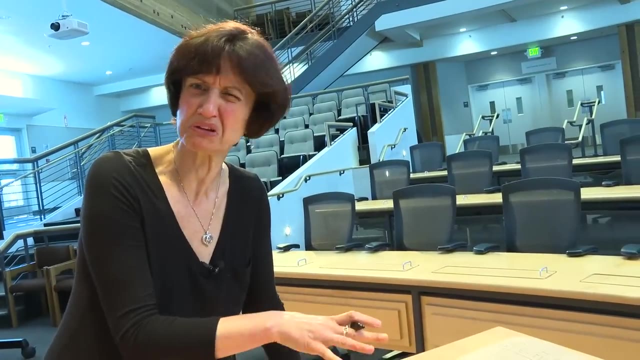 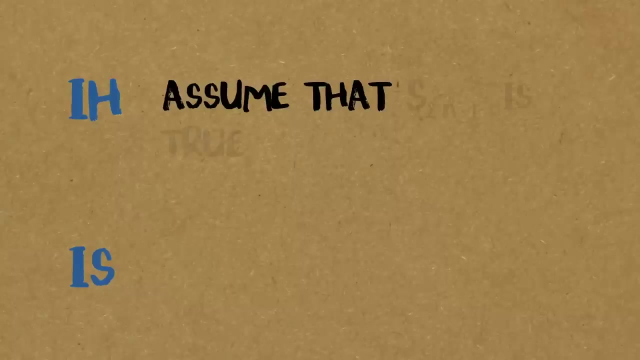 hypothesis. We shall assume that and this is not going to be strong induction like for the squares, it's going to be a regular induction but sort of skipping, because we don't care about the even cases. So assume that S2n minus 1 is true. So this S2n minus 1 is the previous statement here. 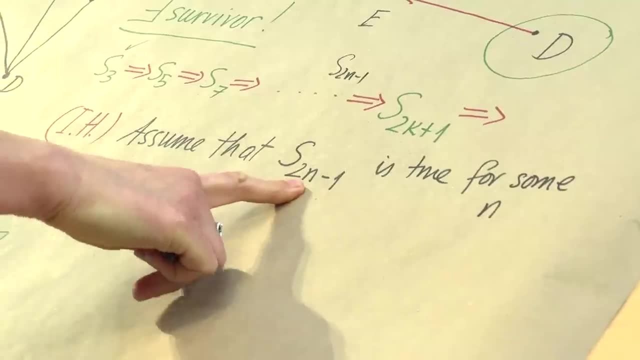 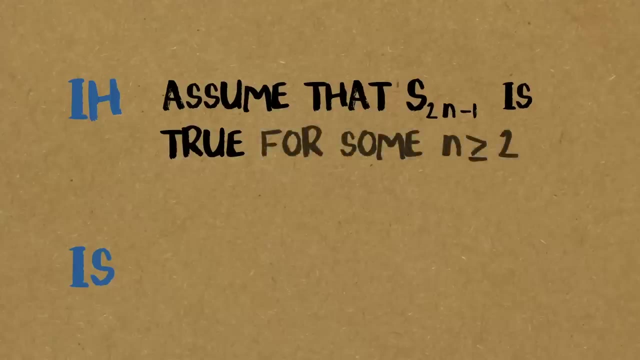 For some n. what should this n be? n cannot be 1 because it's going to be S1. So how about greater than or equal to 2?? Because if n is true, you're going to get your S3. And we want to show inductive step that S2n plus 1 is true. Now I'm going to use finitely many. 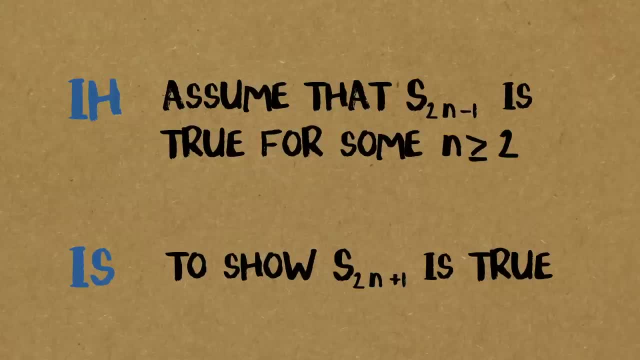 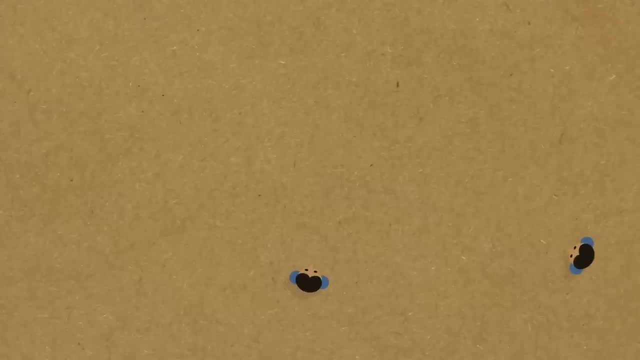 points, a small number so you can see how it works. For instance, let's say we are trying to show the seventh statement, but exactly the same idea is going to work for any n. So how many points do we have? One, two, three, four, five, six. and let's be on the 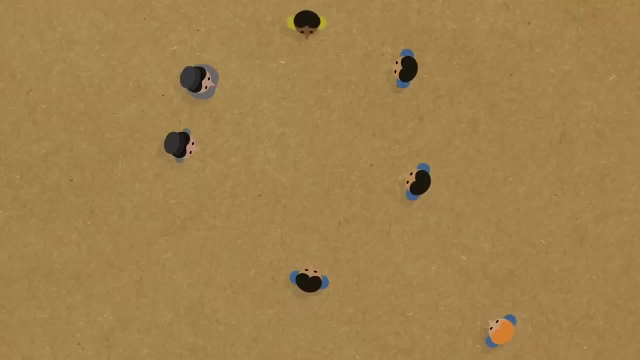 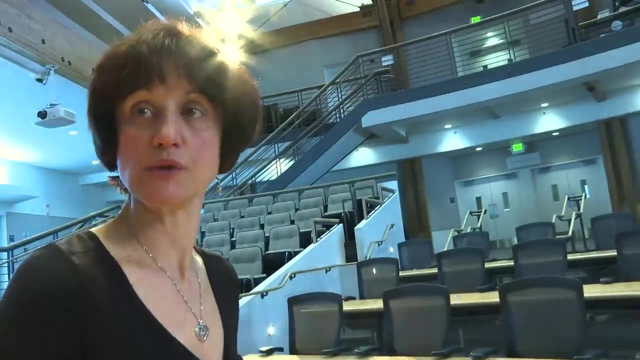 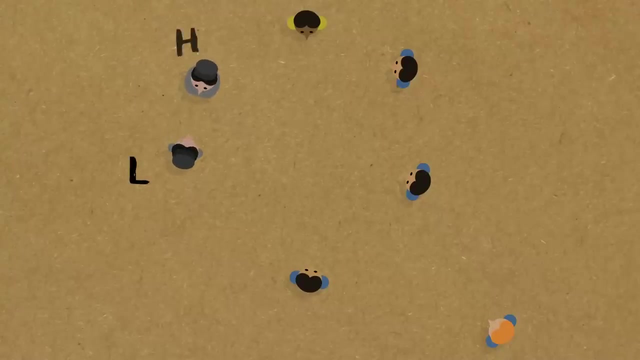 safe side, seven. Okay, so we've got seven people. We want to immediately eliminate some And we go for the smallest pairwise distance, In other words, which two people are closest to each other? Looks like those two, And of course we're going to call them L and H, Laurel and Hardy. 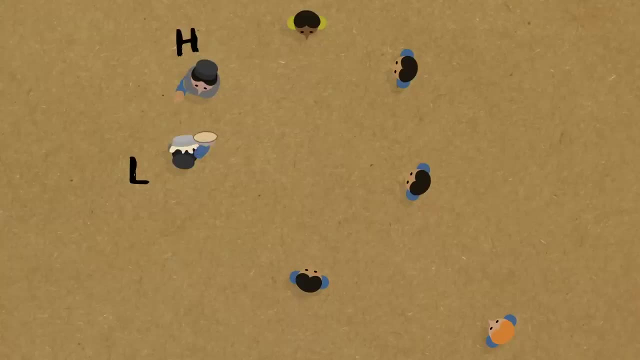 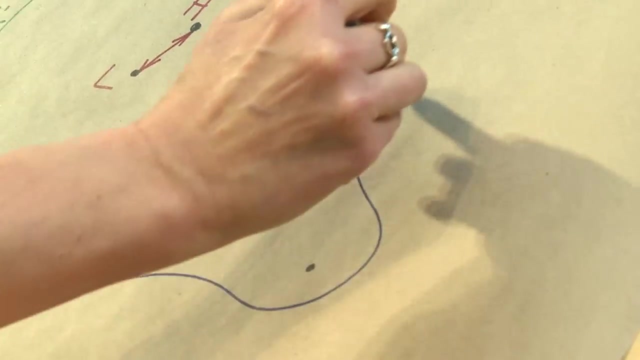 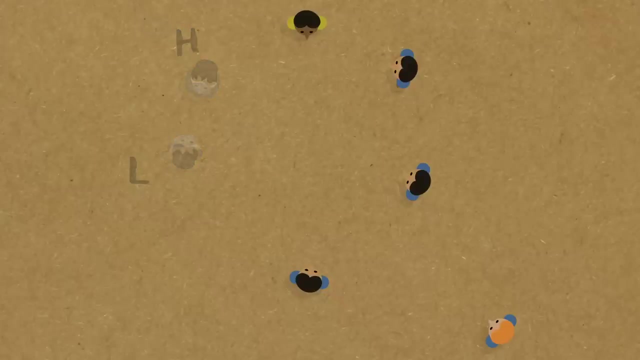 So they're going to pie each other because they're indeed closest to each other. Now, what's going to happen with the remaining five people? We are going to cool off our discussion and ask them to play another game, just temporarily, A game only amongst themselves. 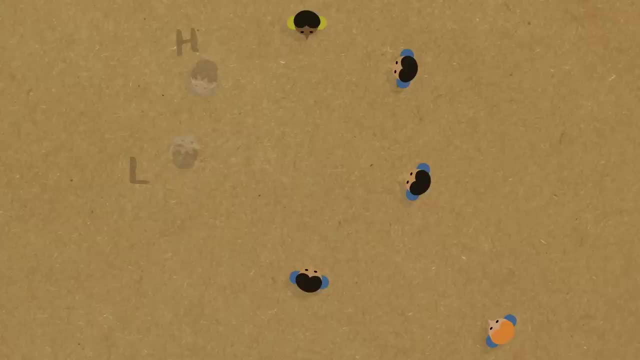 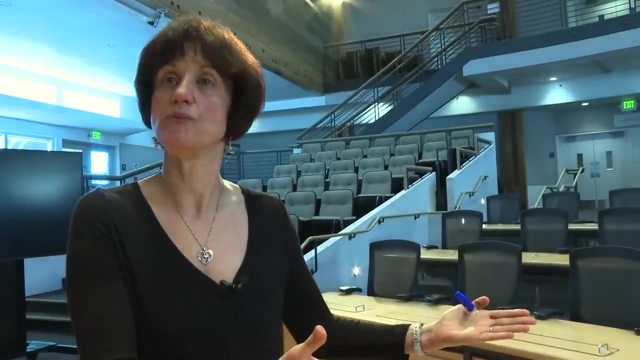 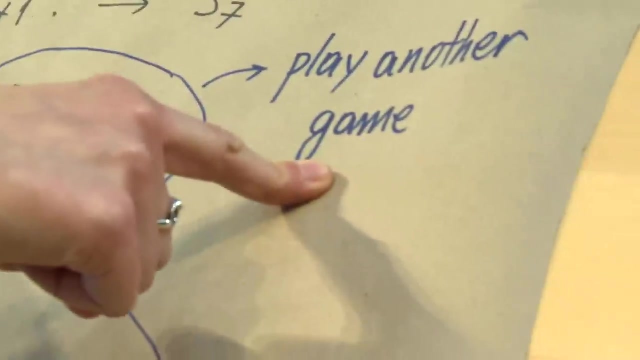 Only those five people play the game. But that's the previous statement and we have assumed that the previous statement is true. So what's going to happen for those five people? There has to be a survivor Just for those five people with this new game. someone survives this new game, So who's 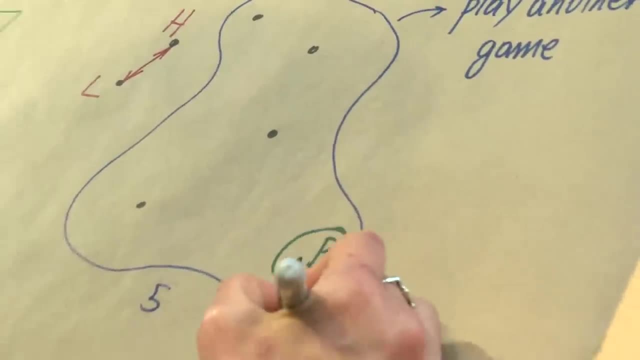 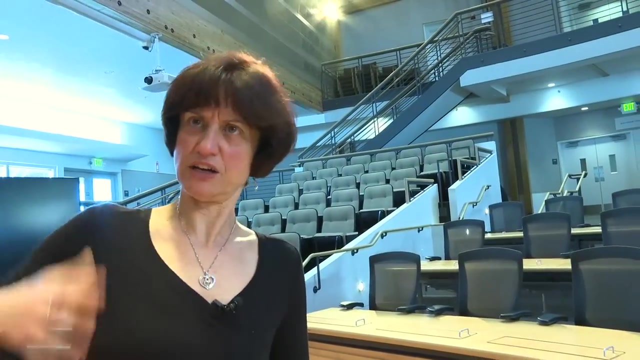 going to survive Brady. Brady survives this new game. What would you like Brady to happen in the old game with you? You definitely want to survive the original game with seven people. Yeah, If you survive this one with five, you'd like to survive the original. 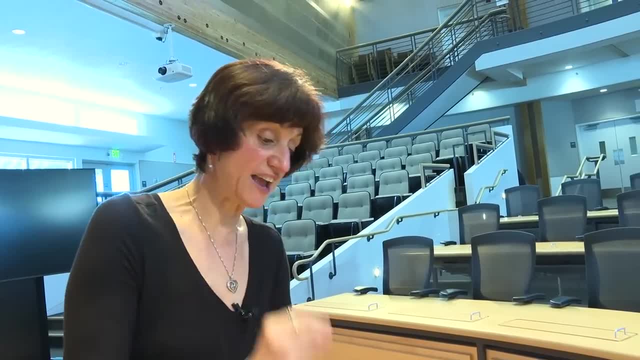 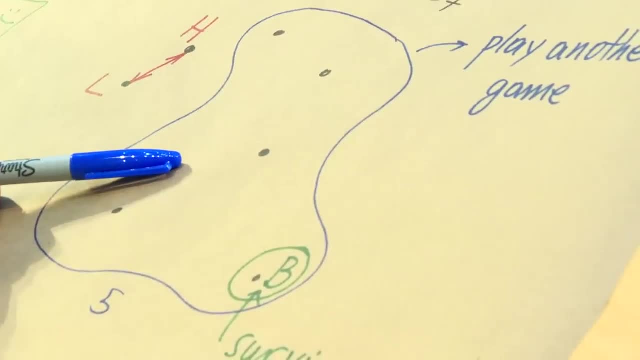 Yeah, And I claim that you will. So whoever survives the smaller game, I claim that person is going to survive the original bigger game. Okay, so now those people who played the five-person game turn around and they're going to survive the original bigger game. 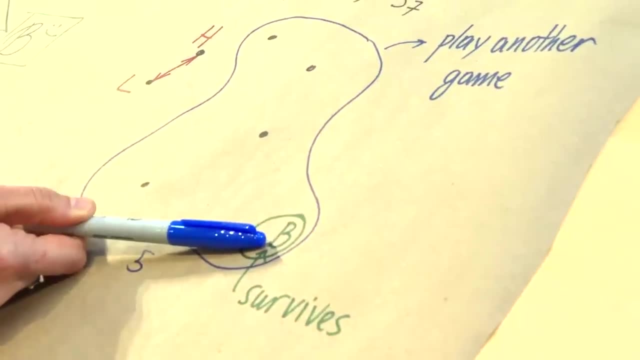 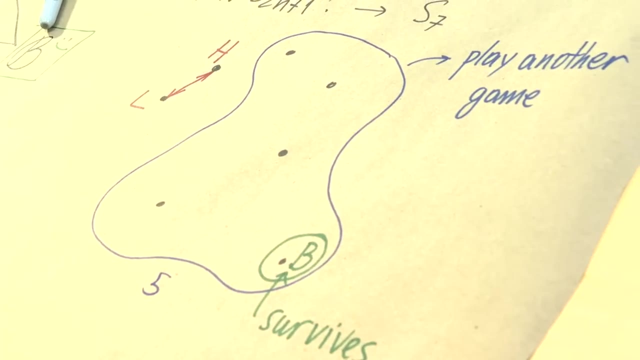 Okay so now those people who played the five-person game turn around and start playing the seven-person game. Okay so now those people who played the five-person game turn around and start playing the seven-person game. Will any pie be thrown to Brady? So what do you think? Well, what happened before was that. 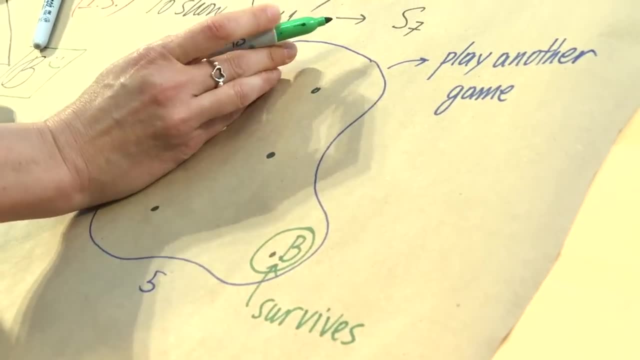 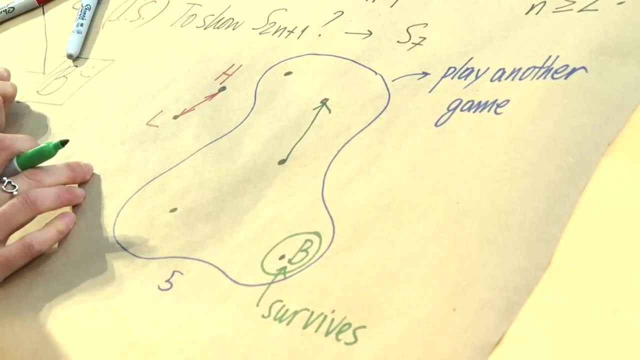 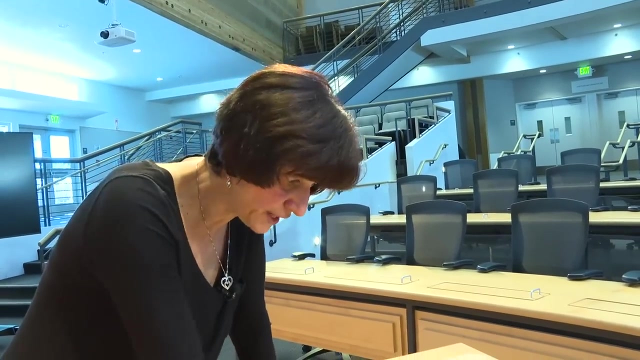 any one of those five people playing the new game. they never threw to Brady So they had a closer target to throw. So in the new game Brady is not the closest person to them because they already have someone closer. So from them nothing is going to go to Brady. But what could happen? 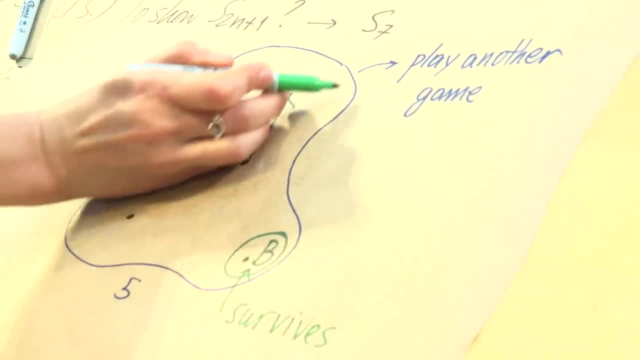 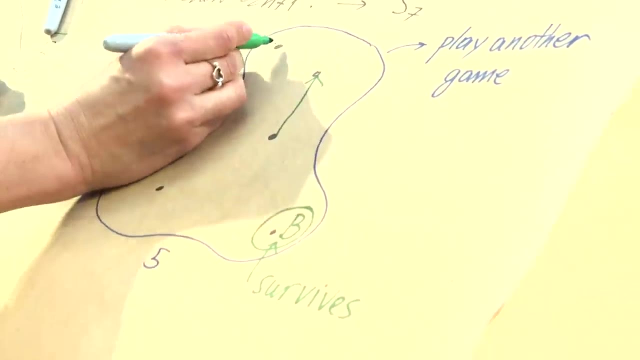 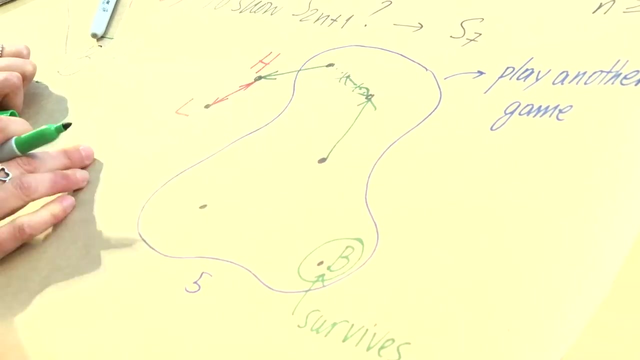 Could a pie be redirected from the new game to the old game, to outside, to L or H? The answer is yes. Maybe this person who before pied someone else here is going to pie harder. That's possible. So some of the pies in this new game could be redirected to go. 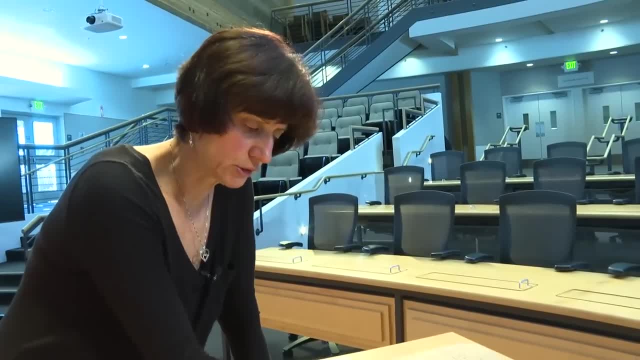 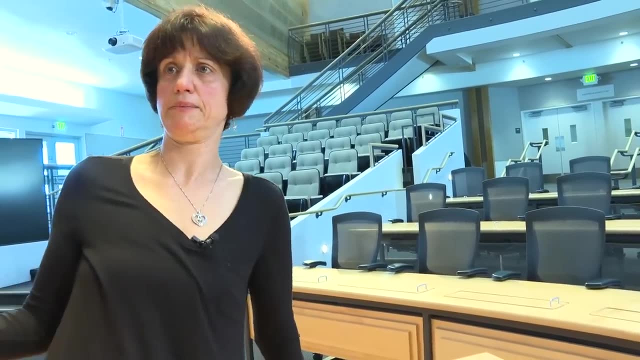 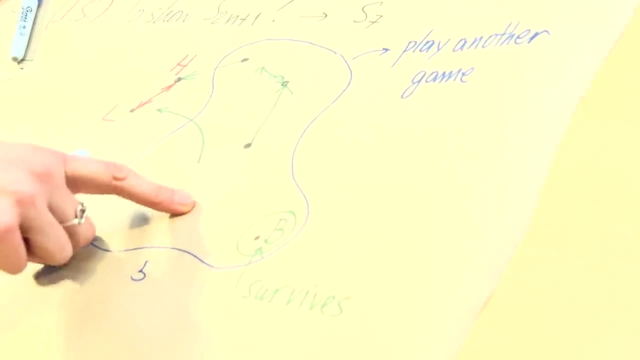 outside to Laurel and Hardy. Could Laurel and Hardy pie someone in this game? No, because they're the closest to each other under any game. So no pies are going to fly. no new pies are going to fly inside our this blue game, which means that Brady is safe. He didn't get pied before. 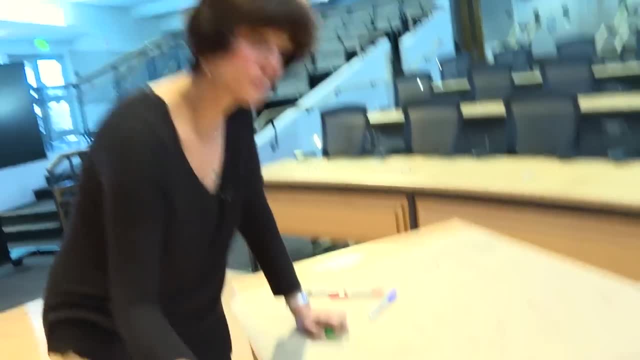 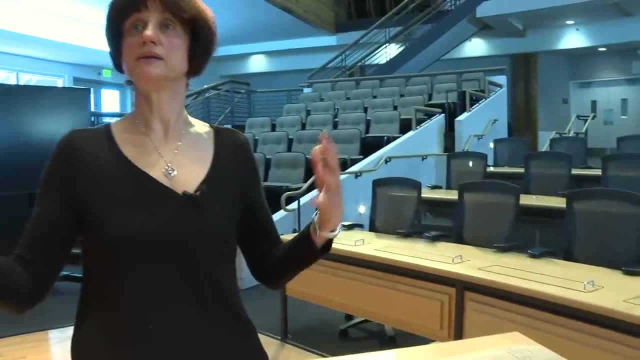 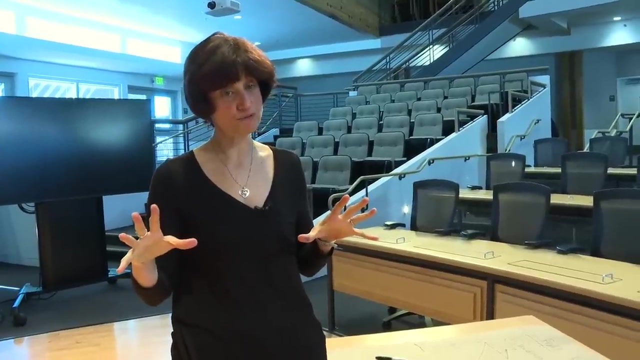 he's not going to get pied now either. And that concludes the inductive step. And now we conclude the whole induction by the method of mathematical induction. All statements are true, In other words, as soon as you have odd number of people positioned at different pairwise distances. 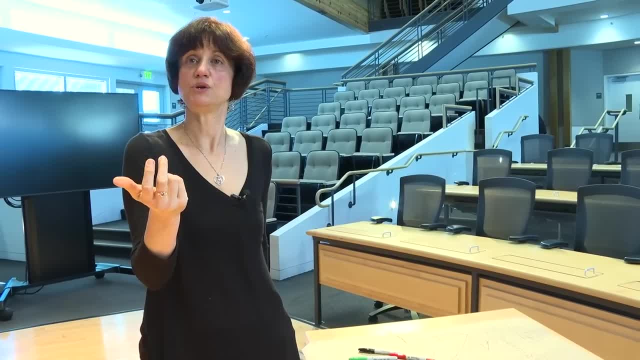 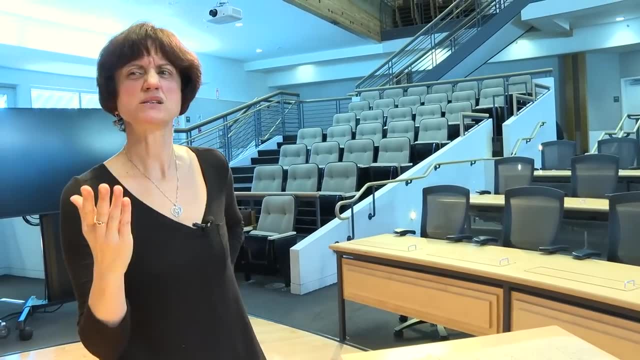 there will be a survivor, Brady. should the survivor be unique? How do you mean? I mean, for every game there should be exactly one survivor. Is that always going to happen? I don't know. I mean, if you have two people, 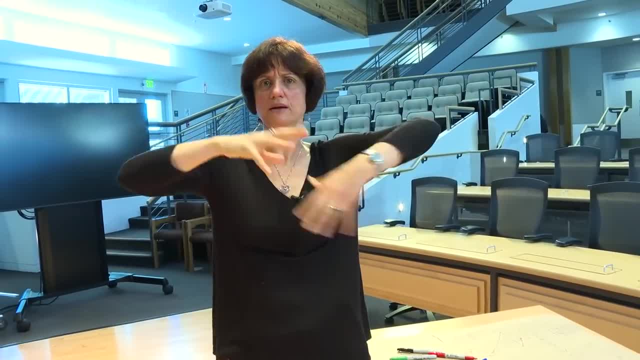 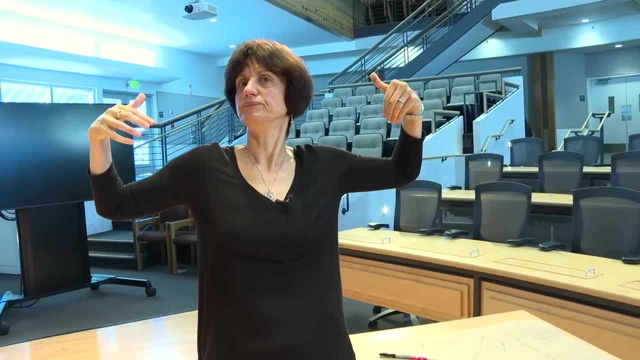 very far away from kind of the other ones. it looks like they might both be survivors. They could both throw pies into, like the center of the solar system, But nothing could go to them. So I'm not claiming that this is a unique survivor. 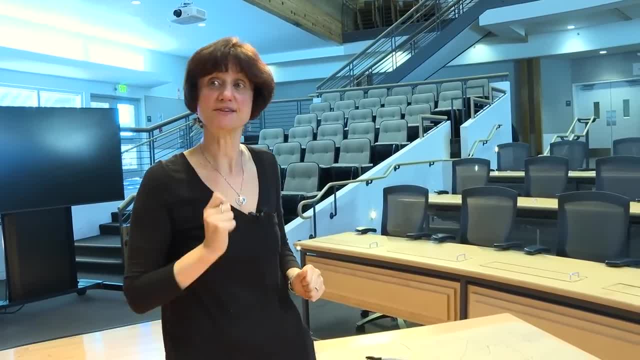 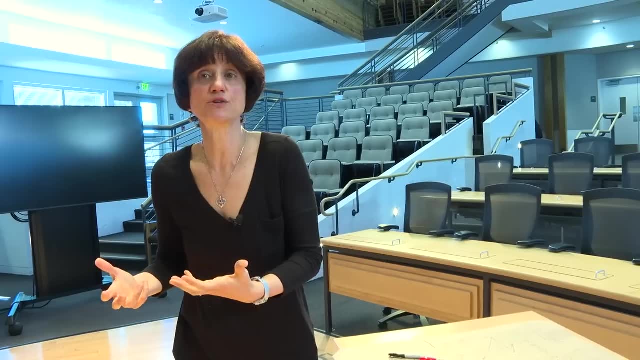 is all I'm saying, But I claim that there is a survivor. And now for homework. you can try to create situations where there are more than one survivor. So there is exactly one survivor for fun to see really well. And then you can try to create situations where there are more than one survivor. so there is exactly one survivor for fun to see really well. 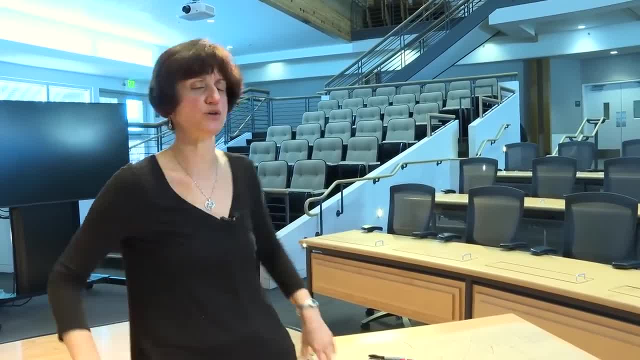 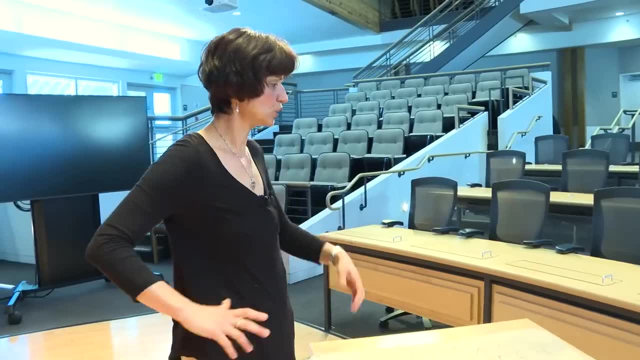 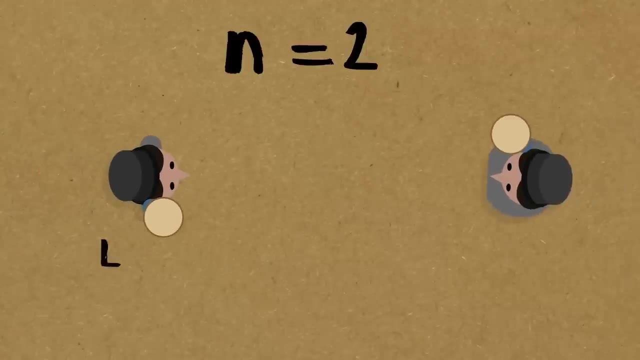 For fun to see really what's happening. But what's the burning question that comes when you solve this problem? Even number of people, Even Why did we exclude the even pie fights? right, Let's see? is S2 true If you have two people at pairwise different distances? 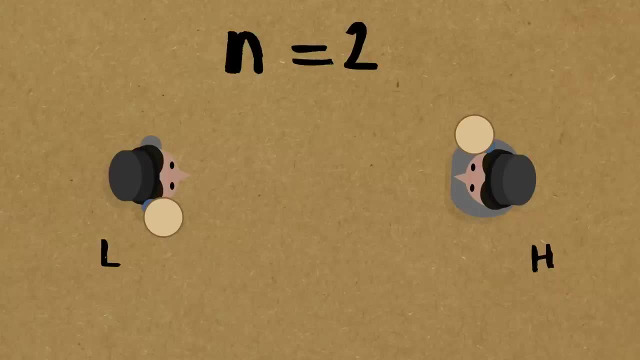 but there's only one distance between them, right, Laurel and Hardy. there is no survivor, They're just going to pie each other without question. So we already see that for two people we can't have it. Well, but you say this is really very simple. 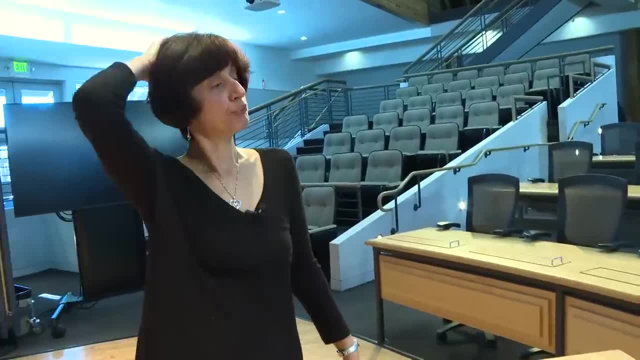 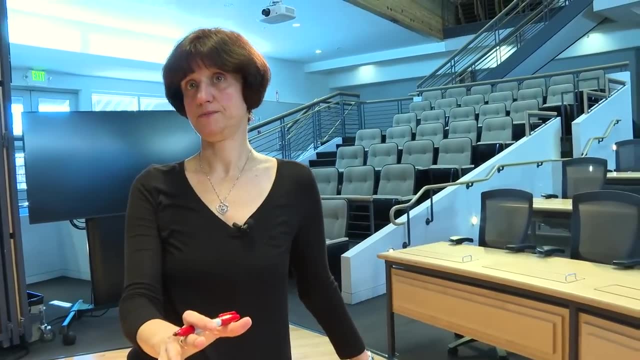 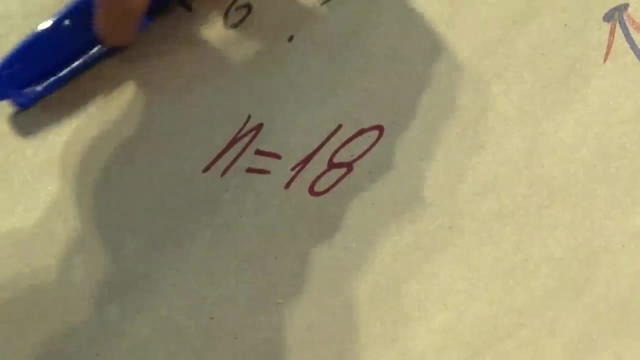 Maybe I could prove this. It's true for a big bunch. number of people, Even number right, For example, how many 18.. Why am I saying 18? Because here is what we're going to do with those 18 people. I'm going to construct for you a counterexample, In other words, I will show you. 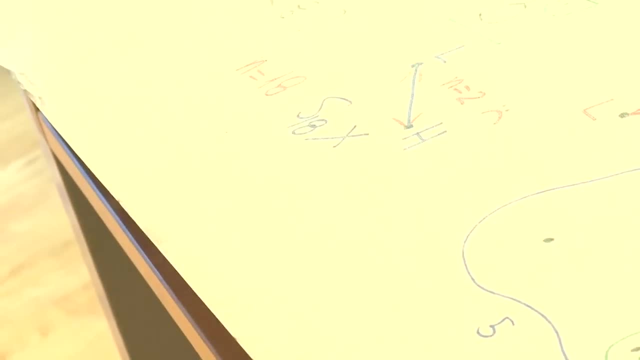 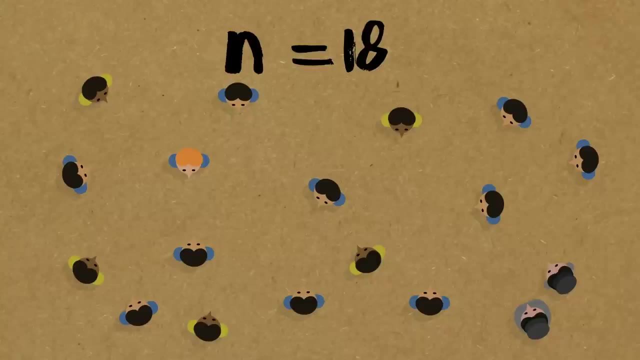 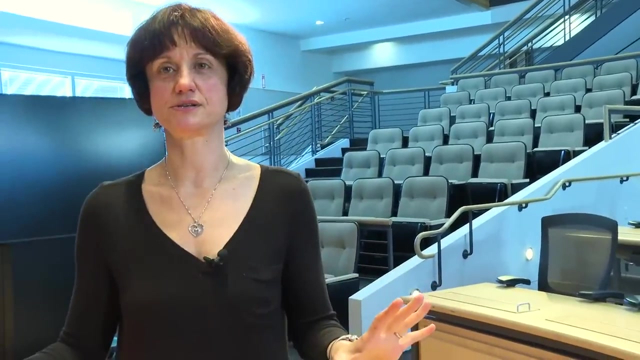 that S18 is not a survivor. Not true. We can put them in a valid configuration where there is no survivor. So what do we do with 18 people, Brady? We marry them off in pairs, disregarding their preferences, Just for the sake of mathematics. they'll do it. 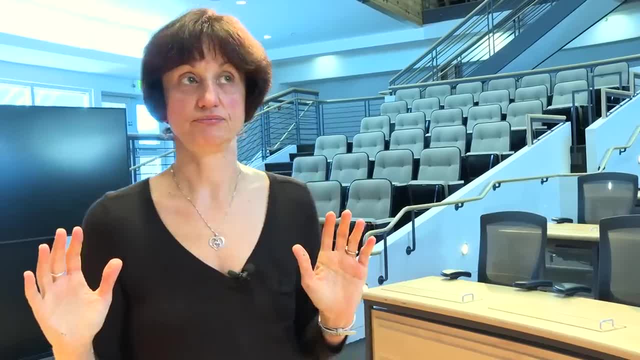 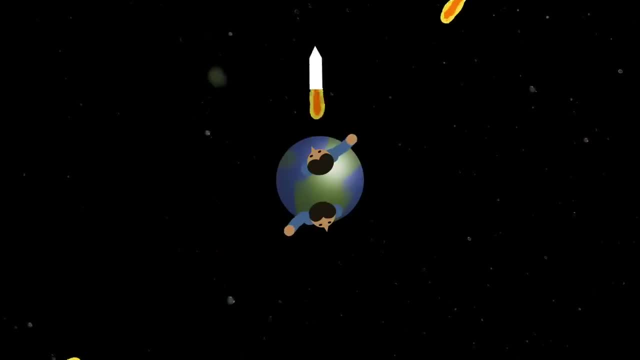 And now that we have nine pairs of so-so happily married couples, we send them off to the nine planets in the solar system. I'm not going to argue about Pluto, Don't even ask me. Okay, And we give, of course. 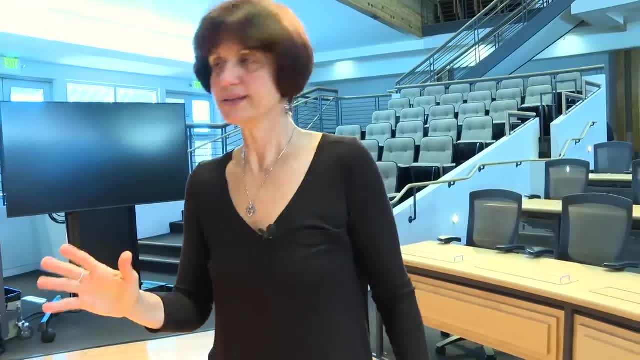 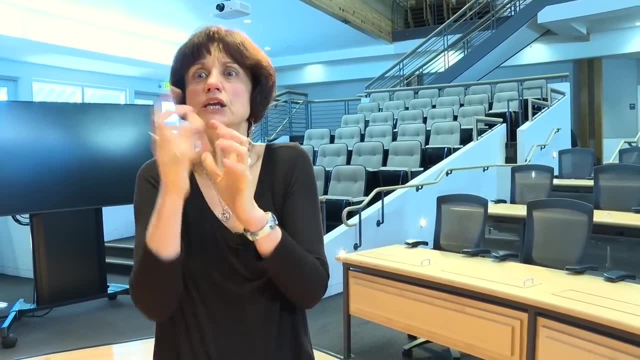 to the newlyweds a pie. Okay, Assuming that they actually survive conditions on these other planets. what's going to happen, Brady? They're going to pie each other In pairs. The spouses are going to pie each other. There will be no survivor, Why? is this happening? Because the planets are so far away from each other- they outweigh any individual distances on a particular planet, And that's why there will be no survivor. So the problem makes absolutely no sense for even number of people. But there is one little glitch that you should. 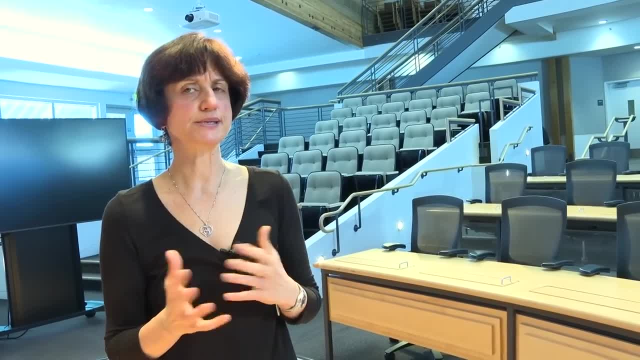 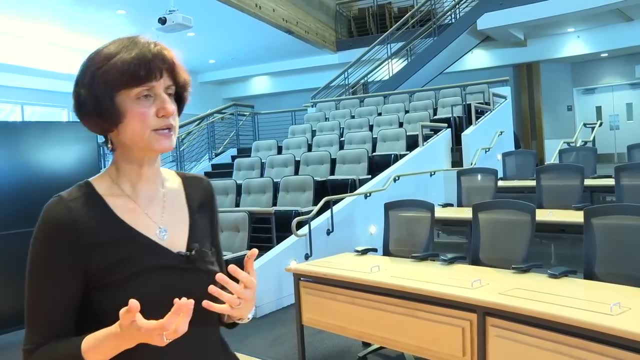 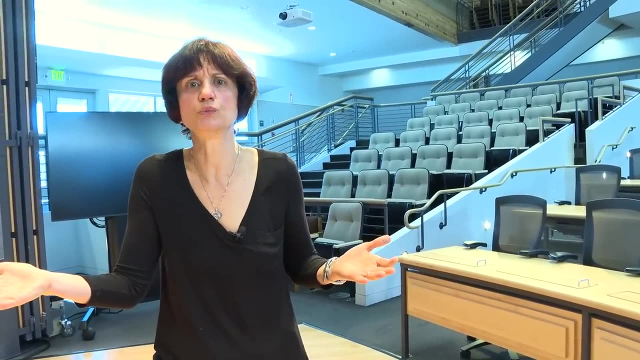 have considered: How about this business with different distances? Could we relax that? Could we allow same distances? You would say: well, if I'm at the same distance from Laurel and Hardy and Brady, then who do I pie? Give them a choice, And will there be still a survivor? Could we be? 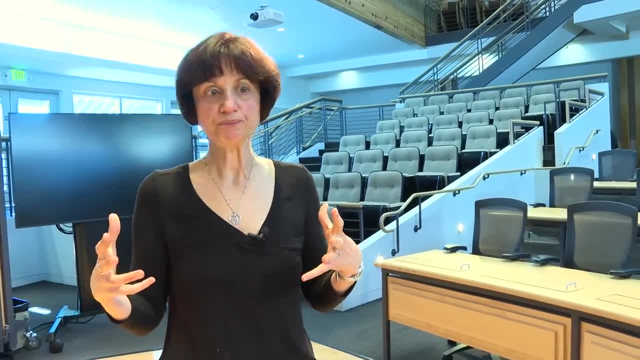 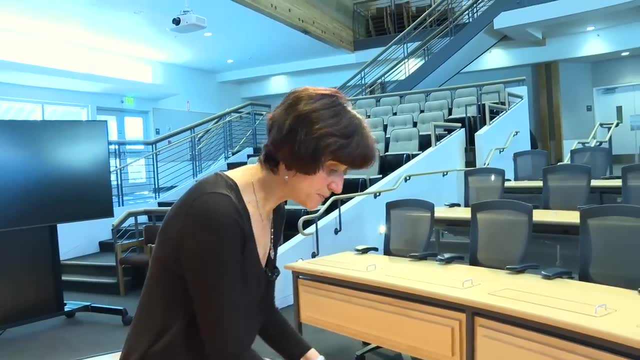 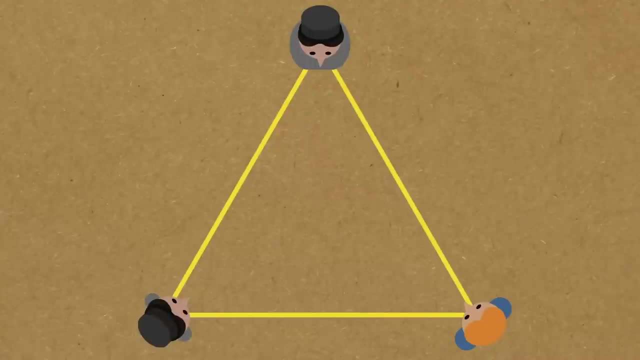 all assured there will be a survivor? The answer is no, Because the simplest situation of all number of people that form an equilateral triangle is going to be a counterexample. They have a choice. Let's say that, for an example in which this happens, that aE must have number three. 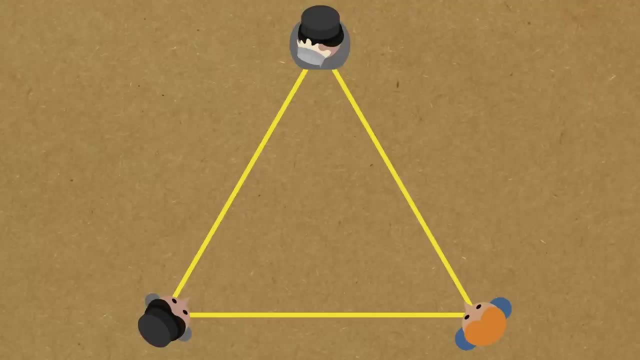 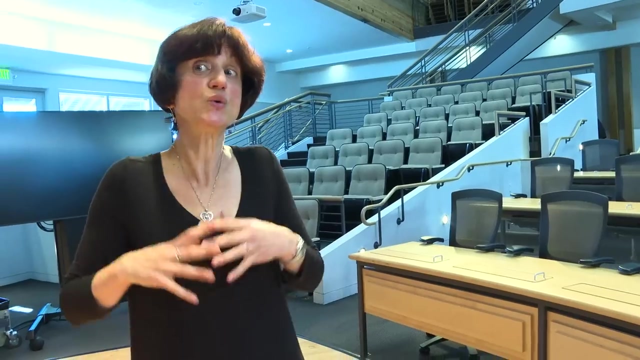 Laurel decides to pie Hardy and Brady decides to pie Laurel. Is Brady safe? No, because Hardy could choose to pie Brady, And so in this situation you don't have a survivor. So if you give this freedom of choice to people with possibly equal pairwise distances, they may not be a survivor. So you cannot. 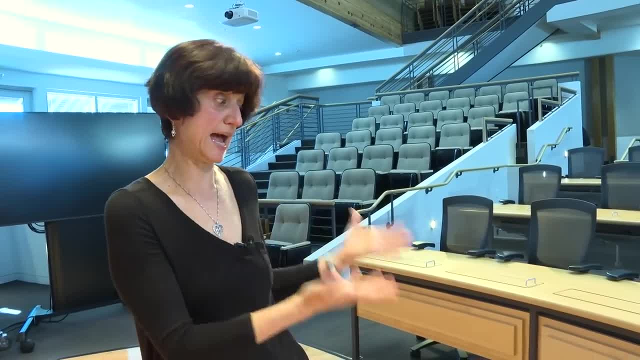 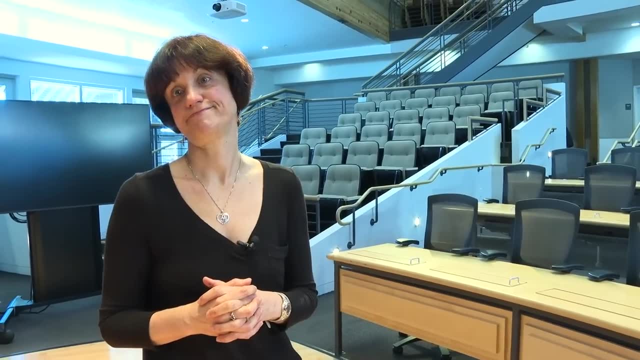 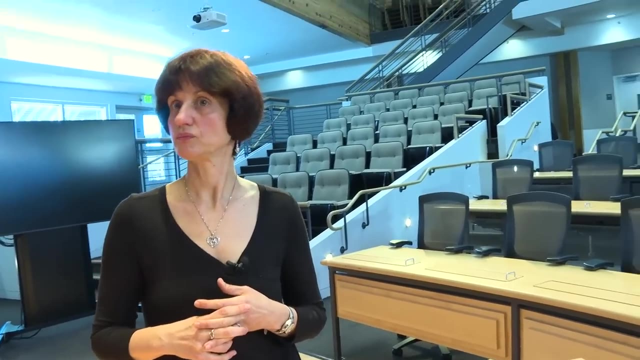 relax the conditions of the problem. The perfect problem is exactly what we solve: Odd number of people at pairwise different distances And, just to be clear, you can have an even number of people and have a survivor. but yes, but you've shown that there's always a. 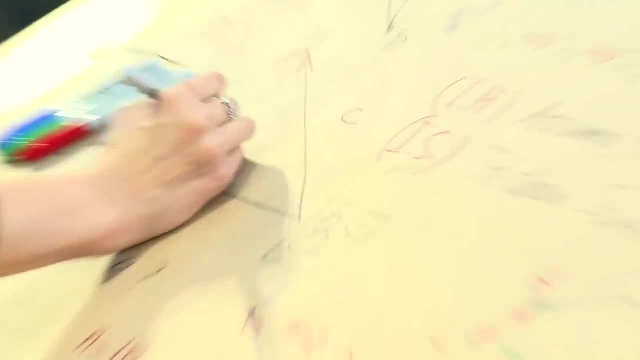 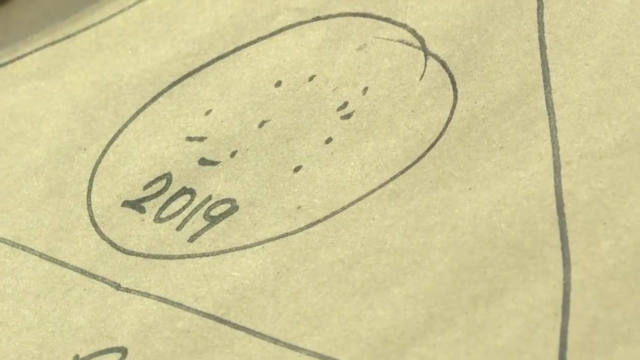 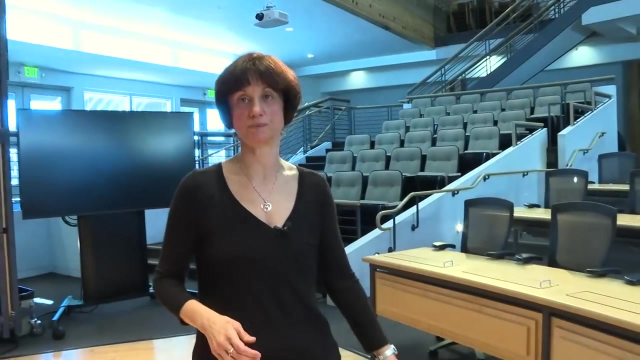 you can always do it with it, Absolutely. you can put all of the other- uh, how many people- 20,, 19 people- inside this room and send Brady to the moon. right, Who's gonna touch Brady? Brady is untouchable and he will survive that even game too. 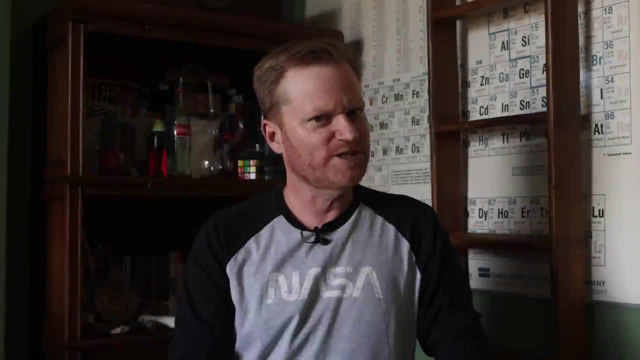 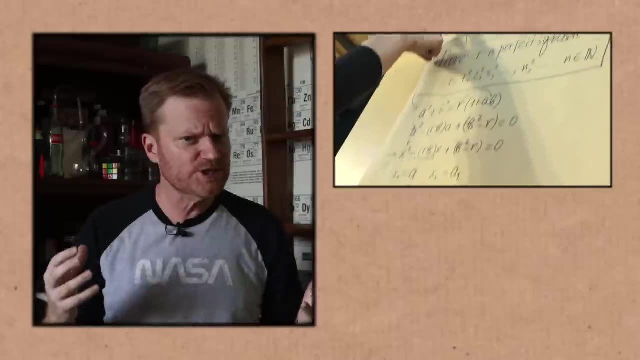 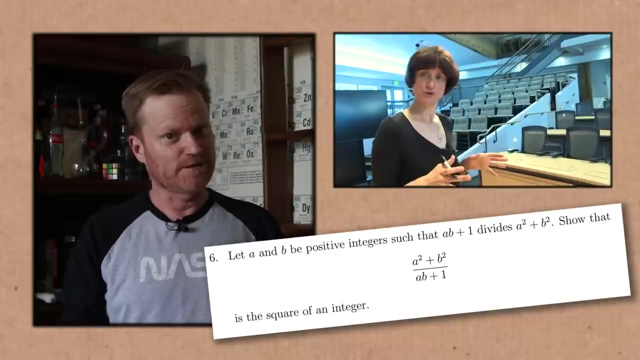 Yeah, So it is possible. We're not finished with induction just yet. In fact, in the next video, Zvezda is going to go back to 1988 and the legendary question six from the math olympiad, which she managed to solve using- you guessed it- induction.